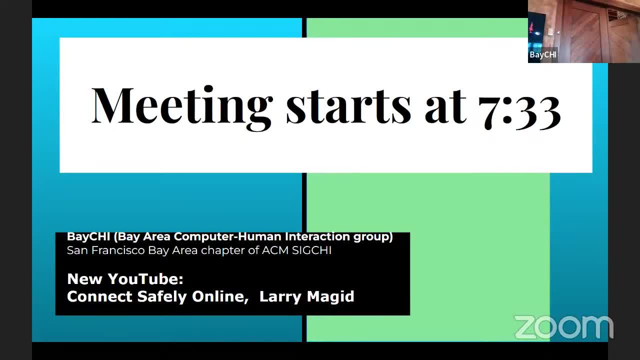 Thank you, Thank you, Thank you. I would have said the same thing. It's not that I don't care, because I only like the fact that I have an Excel spreadsheet. No, I don't like it that people can come into the room. 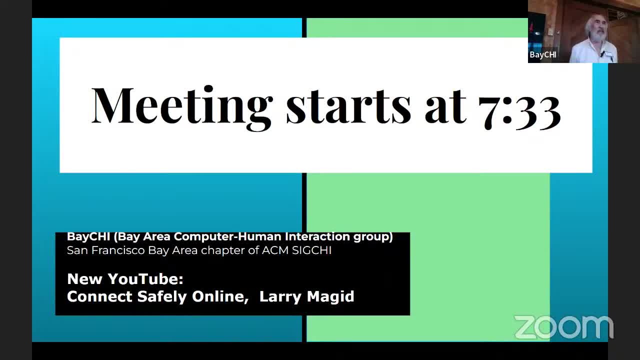 and I don't live in there, So I like to be able to see the staircase and see the projects and things in the room, And I like the screens or whatever. The light behind me and the air is very much, so high. I used to have one. 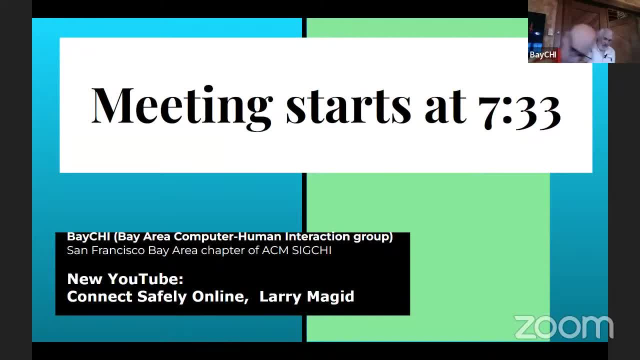 that was like I worked here and then this was the Instagram. Okay, you're going to sit down for a moment, Which worked okay, except that you're staring at a certain thing. You want me to pay attention to this. I didn't talk. 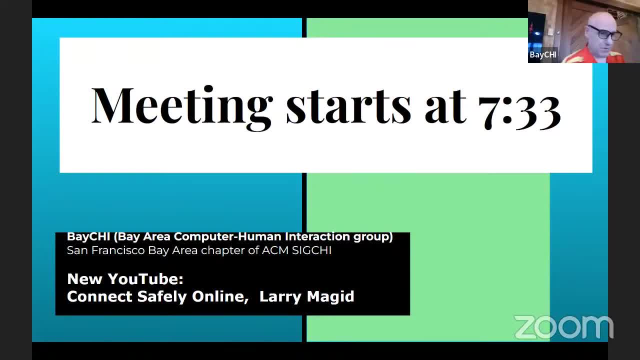 We tried something new every few months. I don't know You could have gotten on. Here's the Zoom of your talk. Ed, do you want that third camera to be active? Steve's asking for the third camera. I think I might be able to. 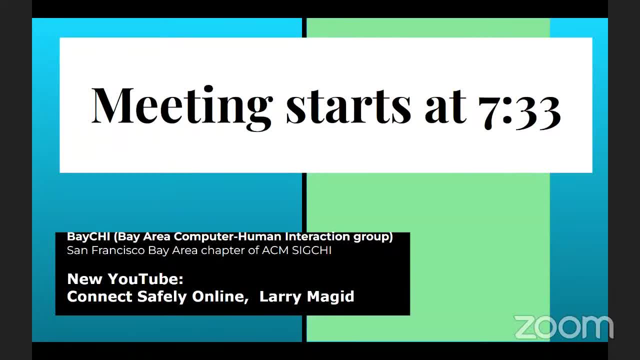 I don't want to be camera-less. Can you make sure that this camera's turned off? I can simply do that on YouTube too. Now we're going to be quiet on set for a moment. Okay, One of them is named Zooey. 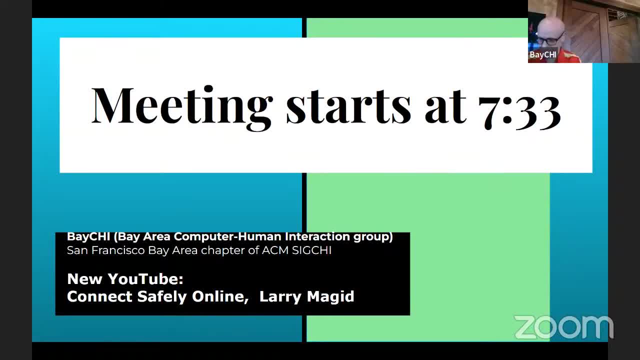 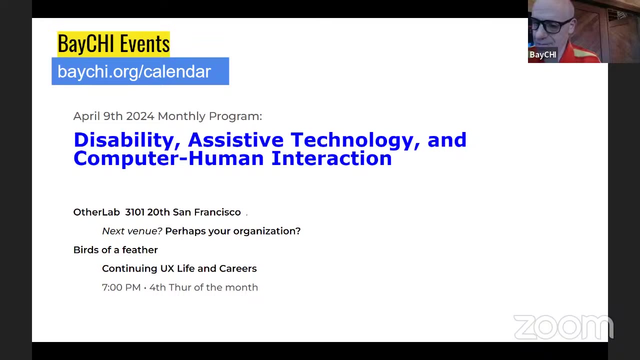 Sounds too much like Siri. So many of the things that have popped with me very sharply saying his name have been transcribed as a text message. Nikki, you're admitting people? Yes, Yeah, we can watch another movie Turning this on. 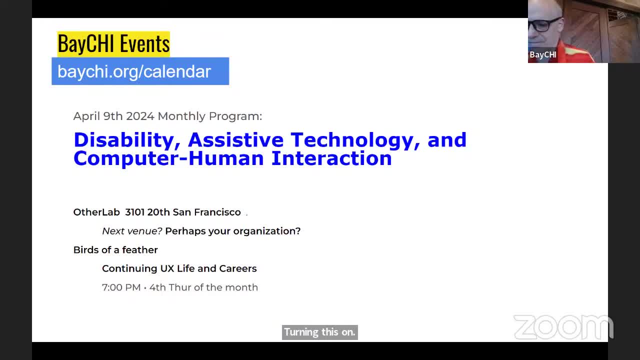 No audio, Ted. No audio, Ted. Can you hear me now? Yeah, me now. Yes, Okay, Something went wrong with that microphone. We'll try the other one Because it's a backup. We have a backup. I don't understand why, but the blue light. 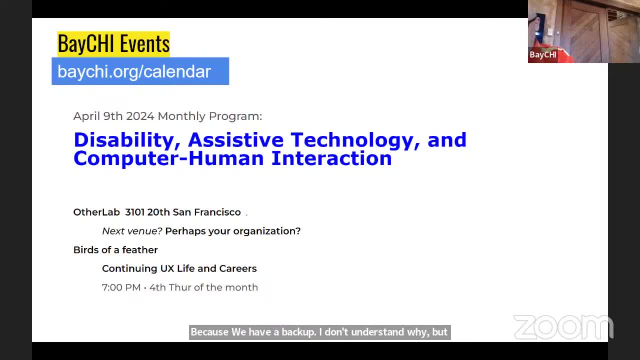 yeah, this is the first time I've used this one, So we'll see if it works, But it might be time. Okay, Can you hear this? Yep- All right, That's working. Yep 2A: 1B- this one's off. Okay, Let's take yours off. Let's change it. 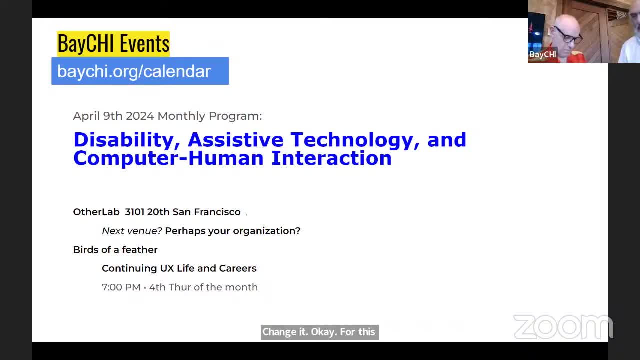 For this one, The current. the current display on the on the ignition screen is the abstract of the picture in picture. Okay, All right. Well, good evening everyone. We are at Bay Chi, where we are at Other Lab, And you can see this 120-year-old or something door behind me. 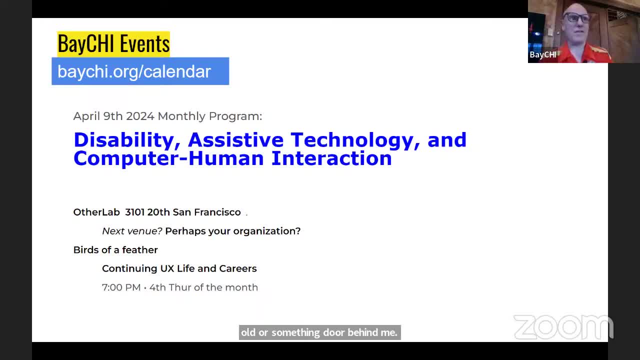 We're in a fully functioning invention lab That that Saul Griffith and Jim McBride founded, And we are not only here, but you'll, if you look around, you'll see that there's pipe organ pipes on the wall, And these pipe organ pipes are part. 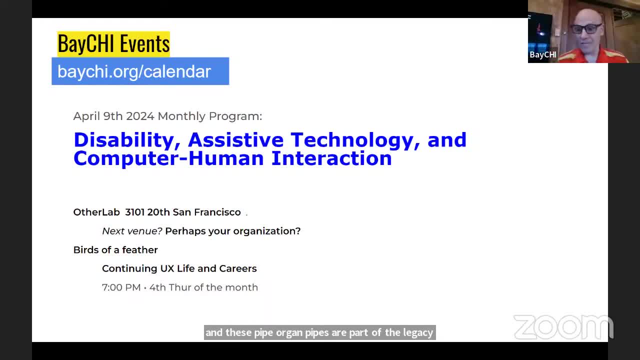 of the legacy of this being a functioning pipe organ factory until maybe five, five years ago. Maybe it's 10 now. In any case, welcome to the program tonight. And tonight we're going to talk about disability, assistive technology and computer interaction. But before we get started I will just take a. 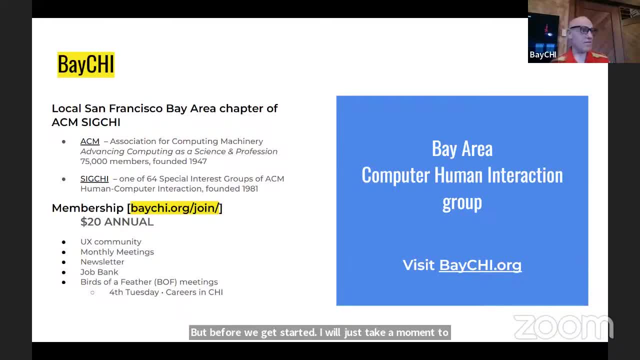 moment to to share with you that we are a part of a 75,000 person organization called Association for Computing Machinery, And SIGCHI, which is the second largest part of ACM, has its annual meeting in May in Hawaii this year- Please go, And we're going to be talking about the technology and the 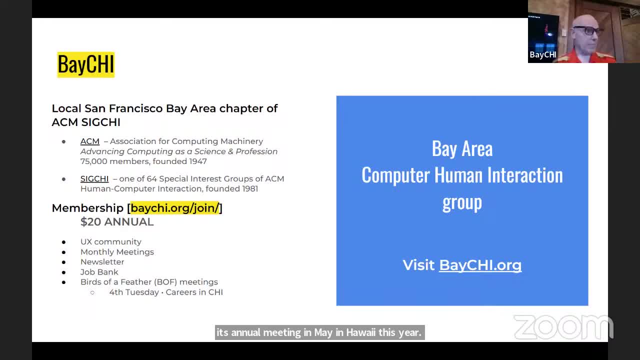 technology that we use, And we're going to be talking about the technology and the technology that we use, And we're going to be talking about the technology and the technology that we use. You can also go virtually online, But we are Bay Chi. Bay Chi is part of that And we are for the Bay Area. we have a 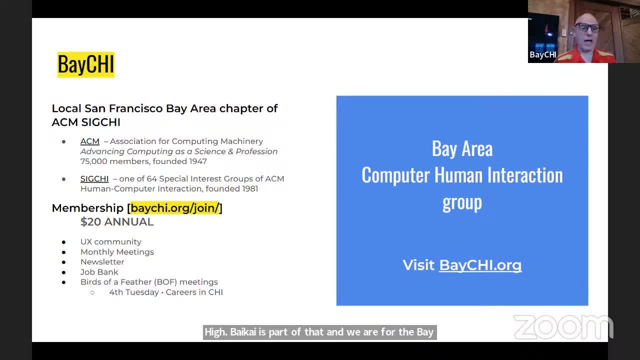 program every every month. We have other things that we do And we really welcome people to join. The most important thing, of course, is the monthly meetings, But but we have steering meetings, which is anybody that's interested in being part of Bay Chi can come to these meetings. 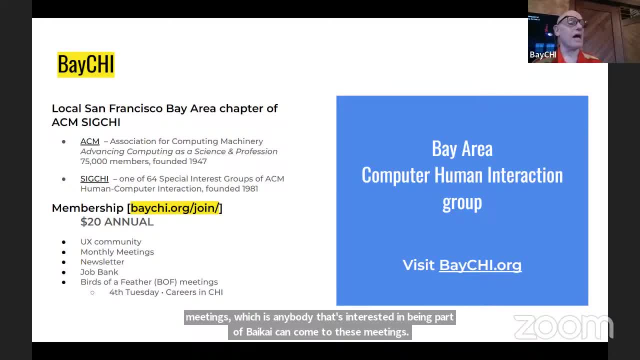 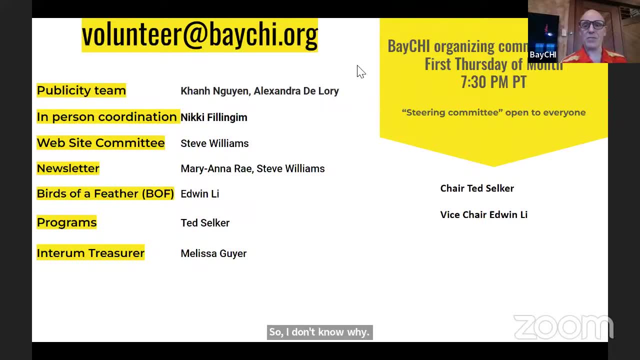 tell us a little bit about what they're doing, but help us also think about what Bay Chi is and how we do it. So I don't know why. Okay, Somebody else should be admitting these people a little bit. So we have, we like people. Oh, it is not. How do I get these slides up there? 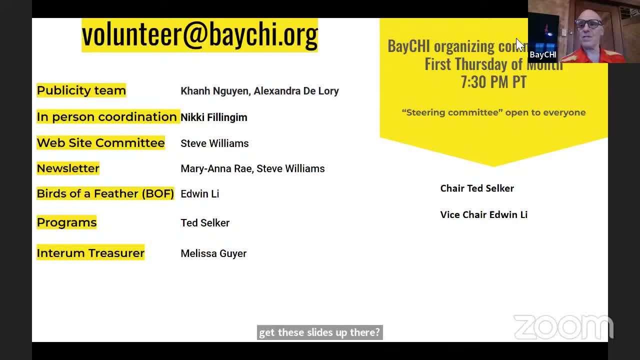 I'm not giving the slides over there. Share, I am sharing. I just I guess people do see these online, They just don't see them over here. How do I put them over here? How do I mirror? Well, I'll just talk to you guys in this room. 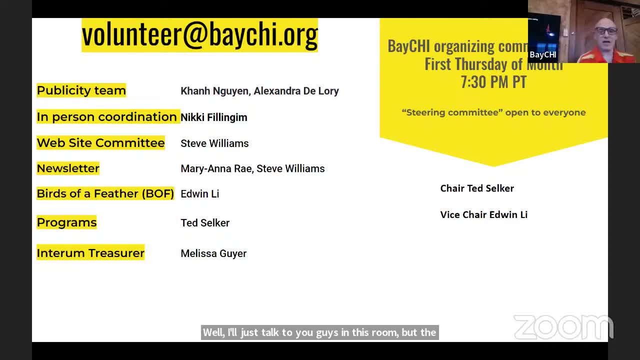 but the rest of the world sees that we're talking about a publicity team that has Con Nguyen And we have Alexander Delory helping. We have Nikki Philman, our very own, who brings, who helps, in-person coordination. This evening it had a lot to do with ice cream and pizza and 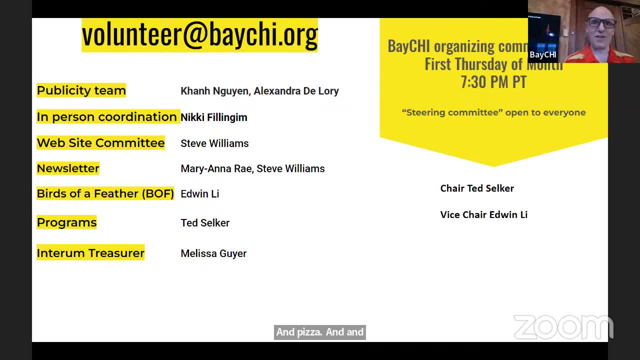 also some other, some other nice things. So thank you so much for joining us. Thank you very much. The newsletter: we have Marianne Ray and Steve Williams putting that out monthly and we are starting to do a better job of getting it out a little earlier, I hope. 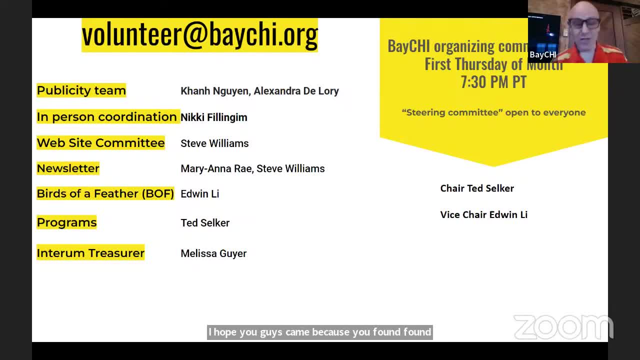 you guys came because you found found us on in your newsletter or found us on Facebook or Twitter or I don't know. it isn't called Twitter anymore. Various LinkedIn. There's a birds of a feather meeting that Edwin Lee runs on the 4th. 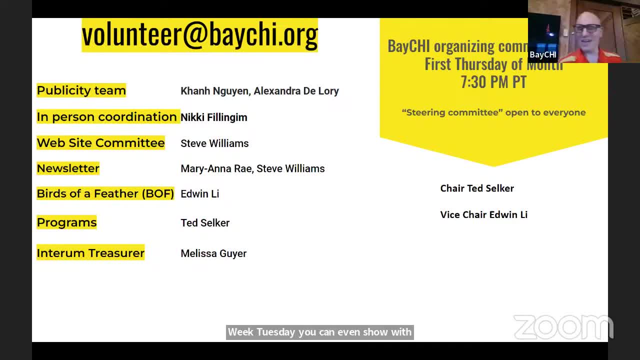 Week Tuesday you can even show with the video, And it is for people that are interested in talking about their careers and what they, what they're trying to do in HCI, And but there's also a working group every week And that is what night. 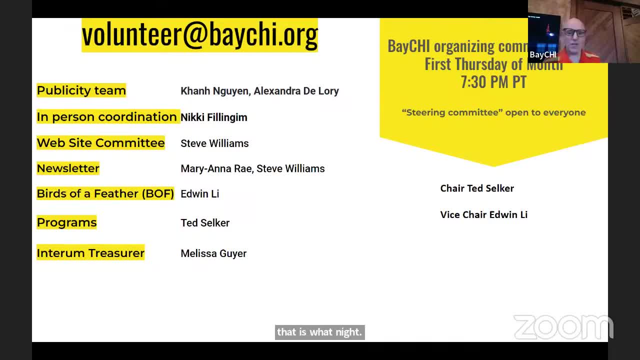 Wednesday afternoon- What time That. that also Edwin runs, And this is a vital thing for people that are looking for work or want somebody to look at their, their work, And then it's kind of, you know, it's kind of a just a working group, just a bunch of us, us kids, And then I'm 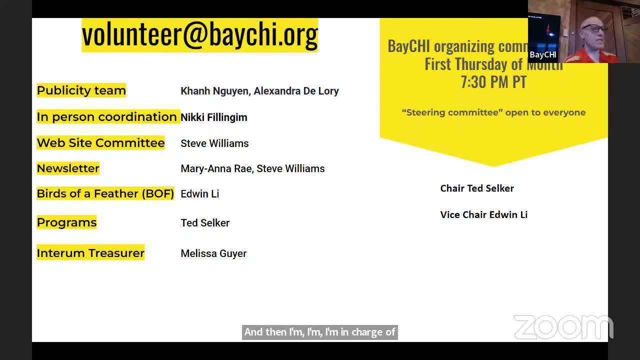 I'm I'm in charge of programs and we have various things on the roster. It's not clear what next month's will be. It might be a visit to a VR company where they use glass beads for reflection And it's very unusual approach to VR. That's a five, five, something, five. 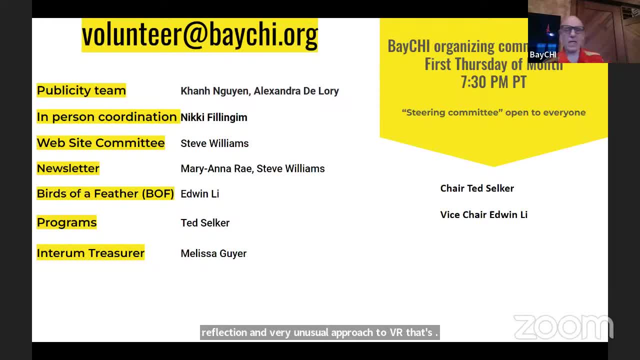 Switch five is the name of the company. Wonderful CEO, Jerry Ellsworth, fantastic speaker, And then on in June we will have Victoria Bellotti, who's a famous, well-published anthropologist that thinks about HCI and was at Park till recently. We have a new. we have a new treasurer. 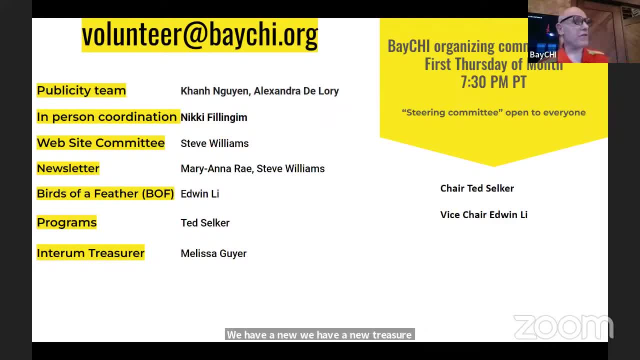 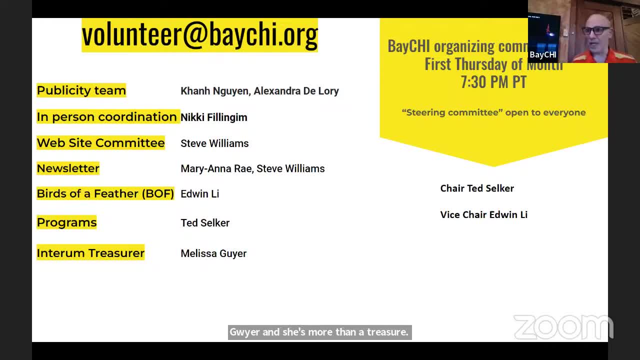 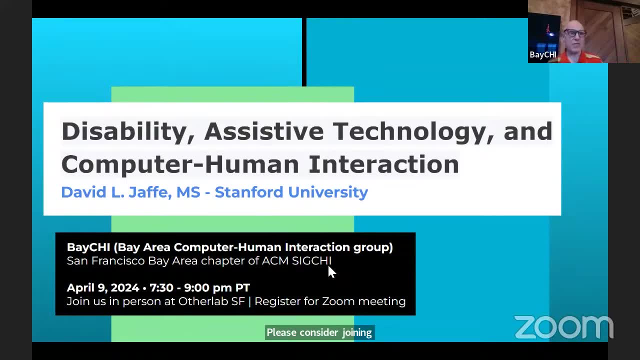 she's diving in and getting interested in lots of different things about, about Bay Chi. So that's kind of what's going on. Please consider joining in. We have many, many other things that we can do. For example, tonight we have Evan Selker who has been doing the editing of all the 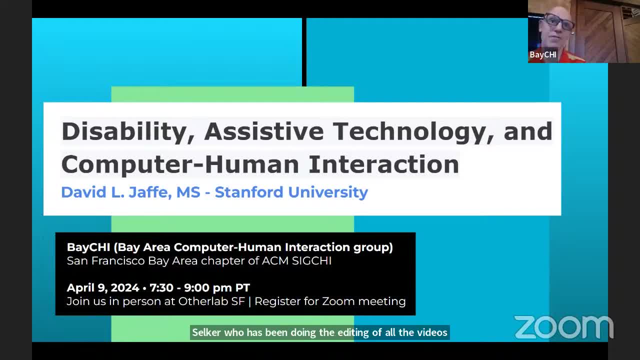 videos And I would love if somebody worked with him to review them because, being related, I shouldn't be reviewing his videos, but also we should be announcing. for example, last week we had, last month we had Larry Magan, very famous writer. He's been writing about technology for 45 years. 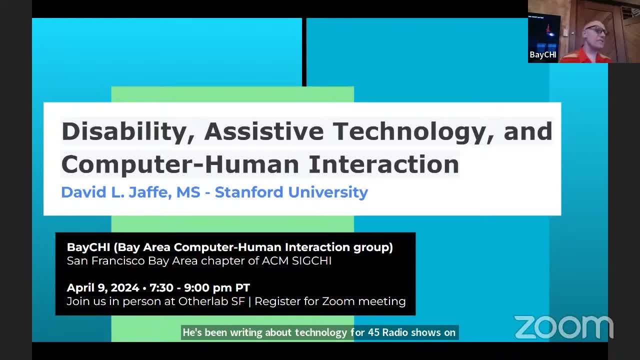 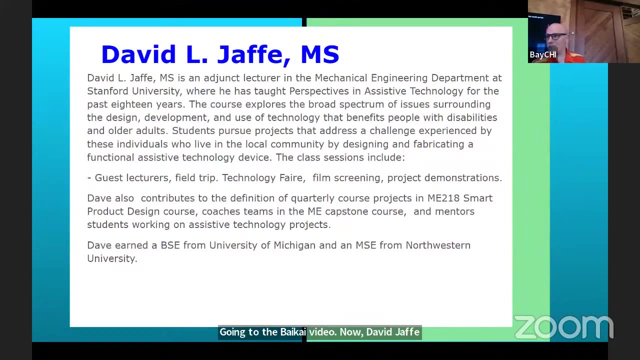 Radio shows on CBS for 25 of those years. Amazing, amazing speaker, I thought, And the video just went up on YouTube. So that's something that you guys should look forward to doing. going to the Bay Chi video Now: David Jaffe, I've known since. yes, Okay, David Jaffe, I've known for. 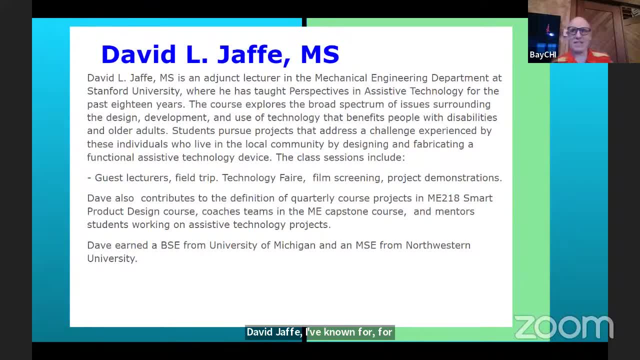 for I don't know 40 years. I think I met him in 1980.. He worked at the VA Rehab R&D Lab. Worked What Worked, I got it, I got it Okay, Okay And, and the lab survived for a long time. Now it's part of a lot of development that goes. 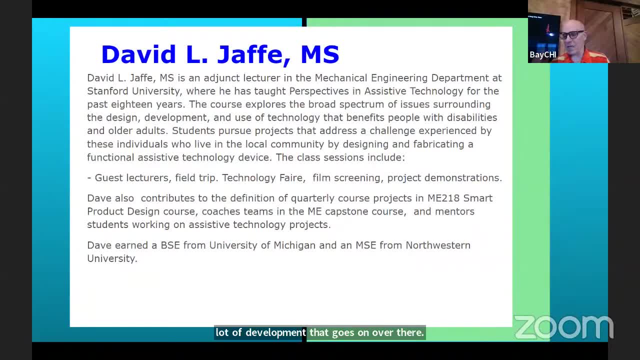 on over there, But the what he worked on was many disabilities things. You'll see some of some of them with him in a wheelchair using just a head to control the wheelchair long, long ago, And it's very interesting that you can use your head to have gestures with other people. 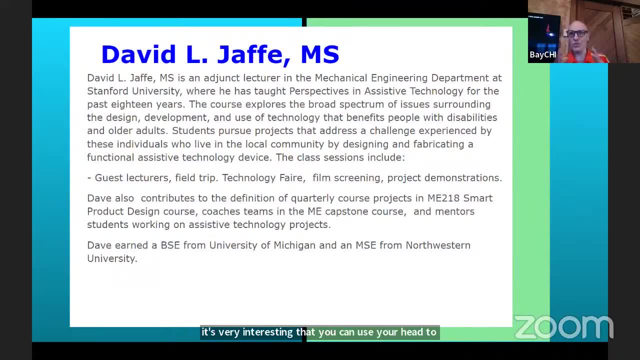 and still control, decouple what you do to to work with a wheelchair. So very innovative guy Now. he's been teaching for for decades now at Stanford And, as in that in that role he he puts on a disabilities class that has projects You'll hear lots more about. 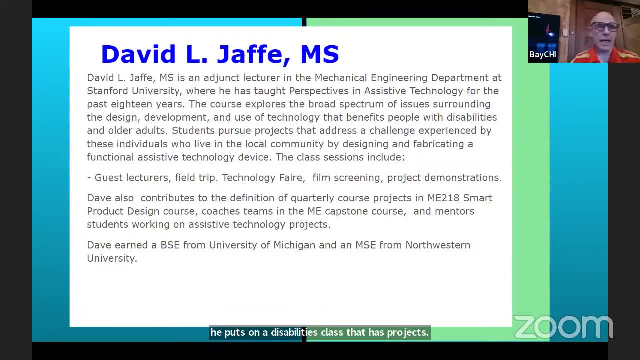 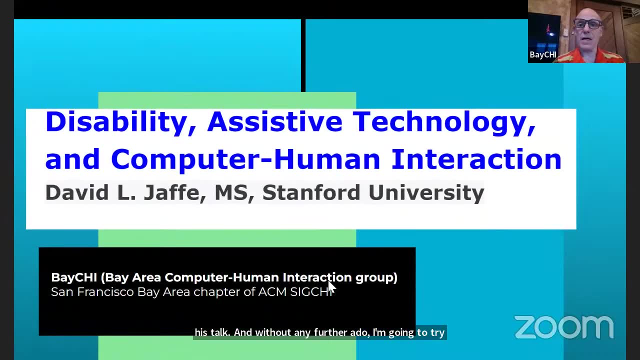 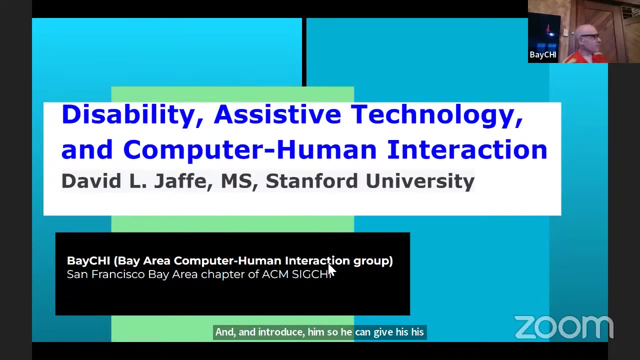 about all of these things during his talk And, without any further ado, I'm going to try to switch over to his slides and and introduce him so he can give his his talk, And I think you know what to do from here. So, David, please come to the podium. 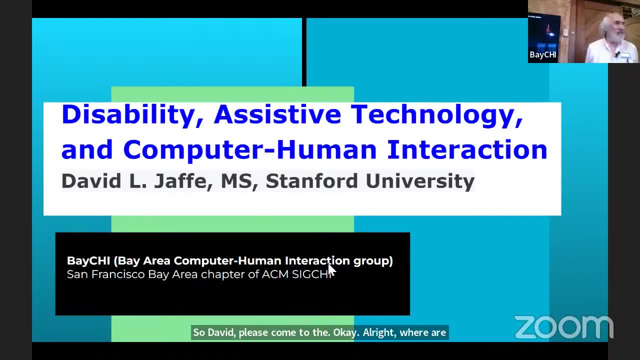 Okay, All right, Here I am. Oh, and one last, one, last thing is: Edwin wanted me to mention that in June we have elections for treasurer, vice president, vice chair, chair and chair, And we're open to losing our jobs. Please take our jobs away from us. 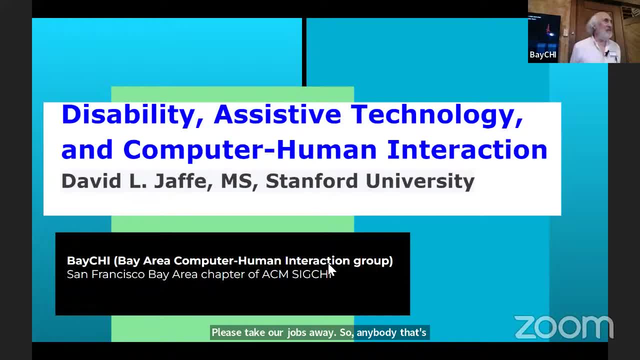 So anybody that's interested, think about taking on more responsibility in Bekai. We're happy. Okay, Thanks, Ted. I want to. I want to thank Ted Selker for inviting me, because I think this is the closest I'll get to a real Ted talk. 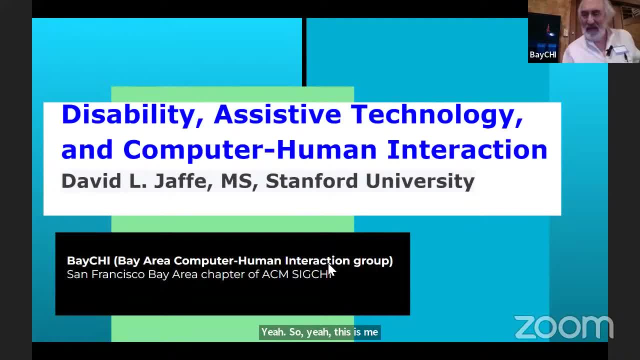 So, yeah, this is me And uh, next slide I'll come What? Just use the arrow keys. Oh, Oh, these down here. No, these are the arrow keys. No, it didn't work. Look over there, Let's see. 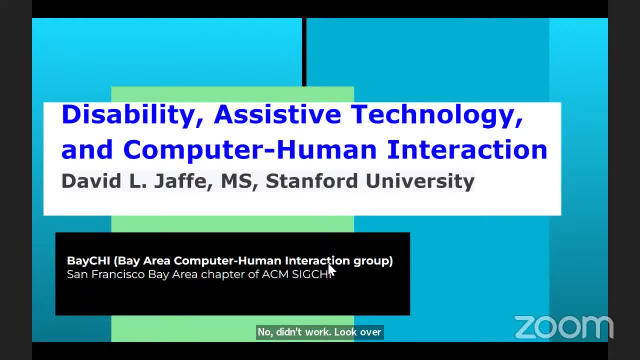 Okay, Ed, on Zoom. we still see your slides Here, I guess. um, that's working now. Okay, Sorry, are you seeing my slides? now You're seeing? Yes, we are, Thank you, Okay, Okay. 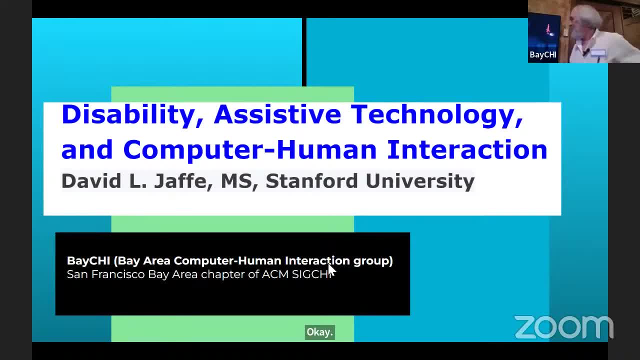 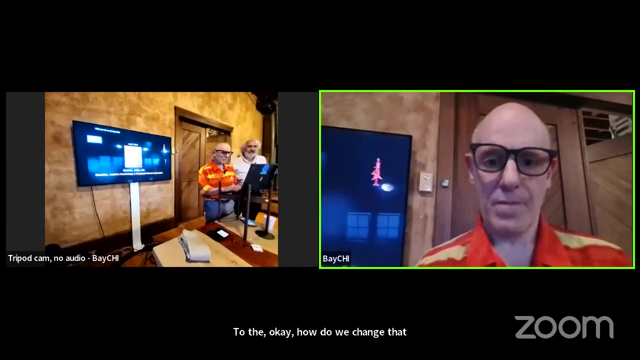 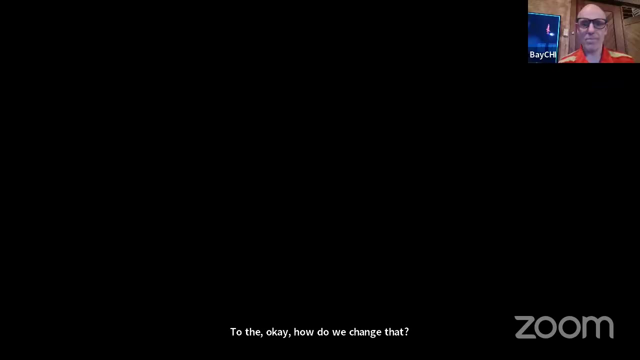 Okay, Do you see? you see David Jaffe's slides? right, Yes, we do, All right. Okay, What, Oh, I uh, okay, How do we change that? Share something There it is. How about now? 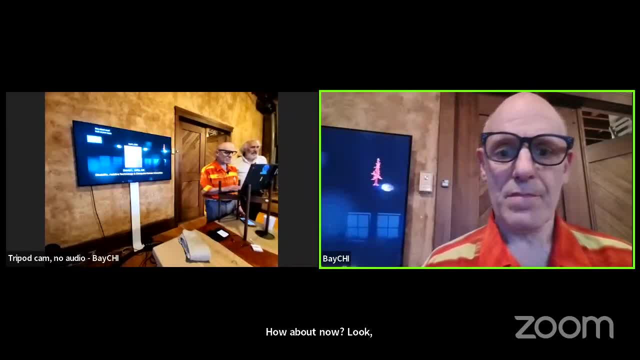 Look, look, how you're in Zoom. Oh, um, at this point now we're just, oh, we seem to be cycling through various video streams. Um, now it's, uh, now it's both pictures of the, of the live video, which I don't think we want. 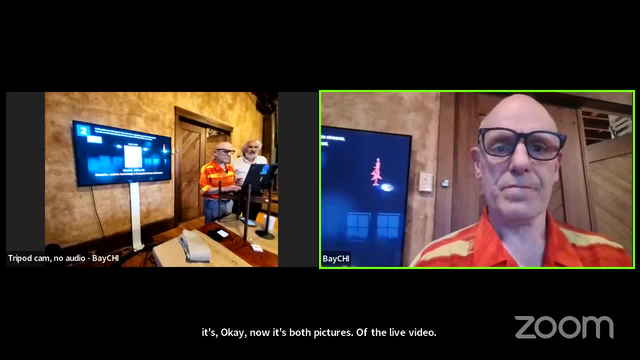 Just just, Ugh, I don't know if you can hear me. I don't know if you can hear me. There we go, There we go. Okay, Forgive me. Um, I think we are at. I use those arrow keys. 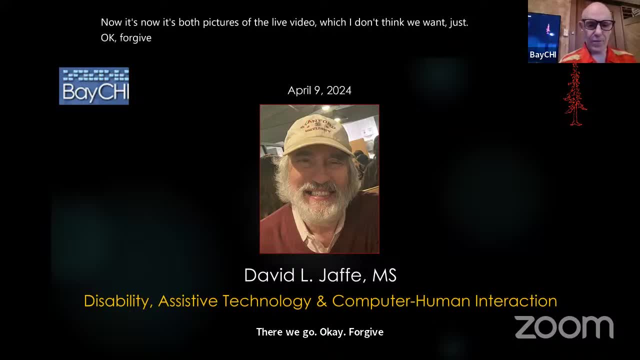 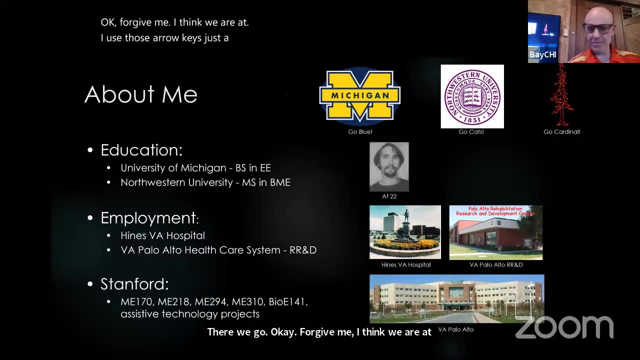 Just a moment. Okay, Now you can use these. Okay, Great, Okay, I'm always so glad when the technology works. Um, so let's get going here. Okay, Okay, Okay, Okay, Okay, Okay, Okay. 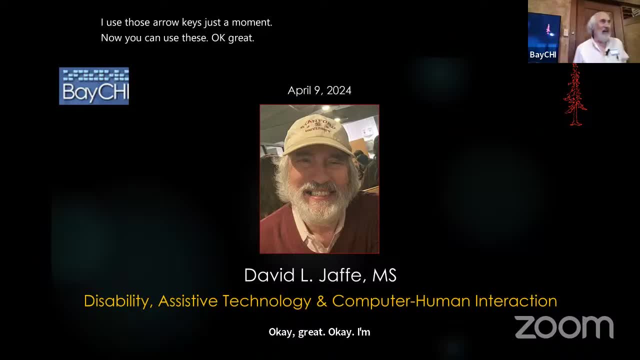 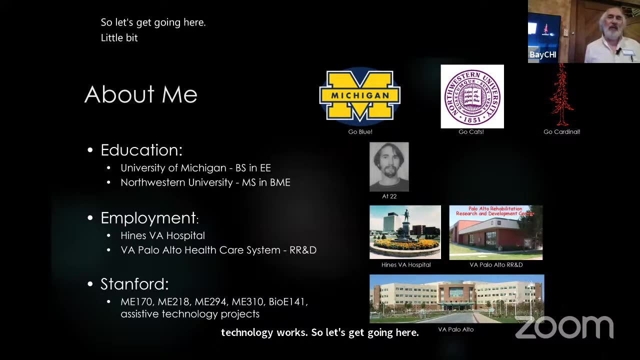 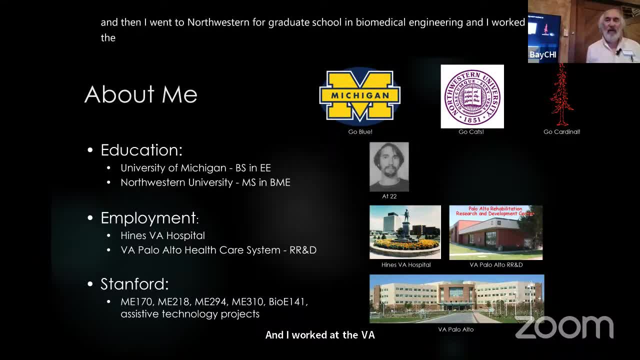 And I worked at the? uh, a VA hospital outside Chicago, uh, for a number of years before coming out to California, uh, working at the VA hospital, uh there, uh, we had a uh center called the rehabilitation research and development center. 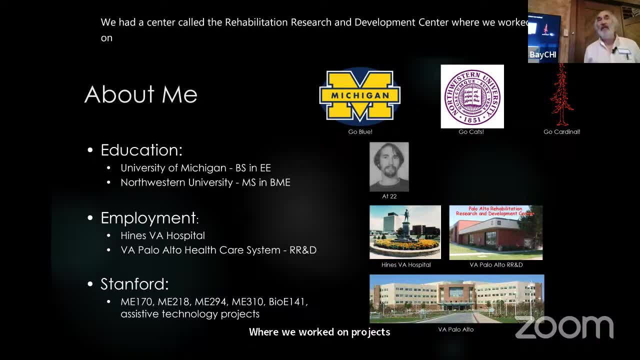 where we worked on projects to benefit veterans with disabilities, including those with spinal cord injury, which is the clinic right across the street. And in 2007, I moved over to Stanford and started teaching my course, And I've been not only teaching the course but helping out in other courses and also trying to connect with other people. 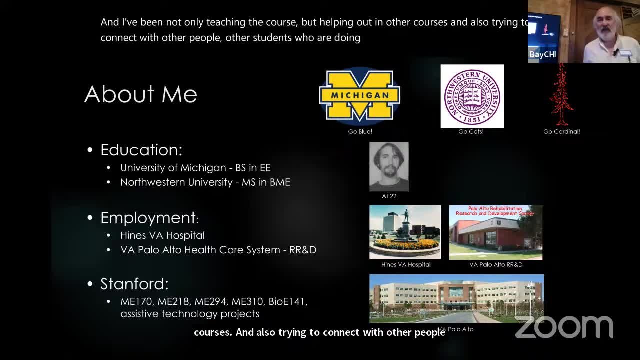 other students who are doing assistive technology projects outside of my class, And it's just interesting to see what I look like when I was 22, when I was at Northwestern, And I students really get a kick out of that. And I tell them: you know, wait, wait till you're my age, you know. 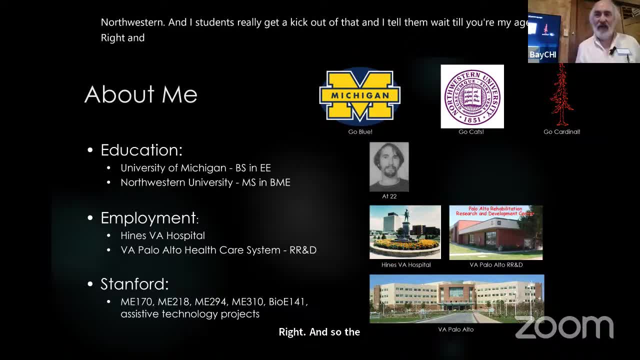 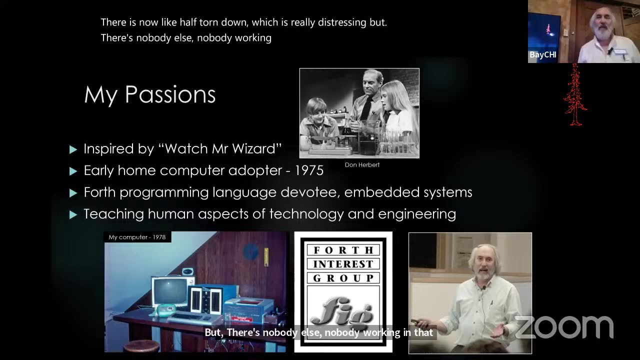 Right, And so the the center that you see there is now like half torn down, which is really distressing, But there's nobody out, nobody working in that center anymore. So my, my background. I remember growing up and being inspired by Watch Mr Wizard. 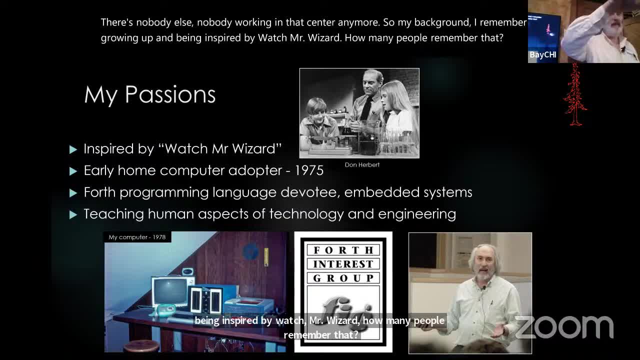 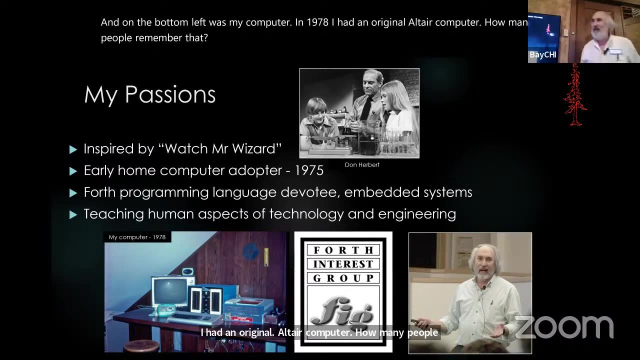 How many people remember that? All right, Just the old people, Thanks. And on the bottom left was my computer. in 1978. I had an original Altair computer. How many people remember that? OK, And so I remember a meeting we had in Chicago of all the people in the Chicago area who had a home computer. 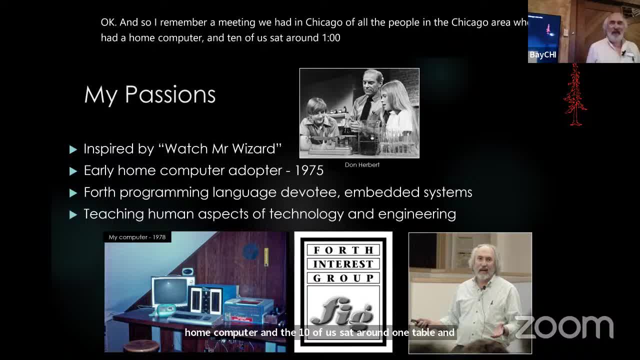 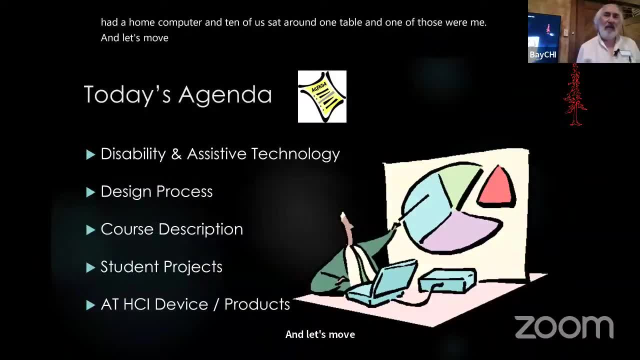 And the 10 of us sat around one table, and one of those were me, And let's move on. So I'm going to be talking about, you know, five topic areas about disability and assistive technology design process that the students use in my course. 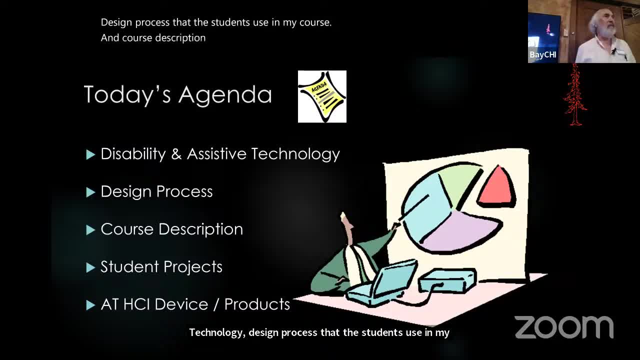 I'm going to do a quick overview, maybe two or three times, and then I'll be able to get out of the way. But I know that what I said is it was going to be about disability and course description, some of the student projects and some devices and products that are you know. 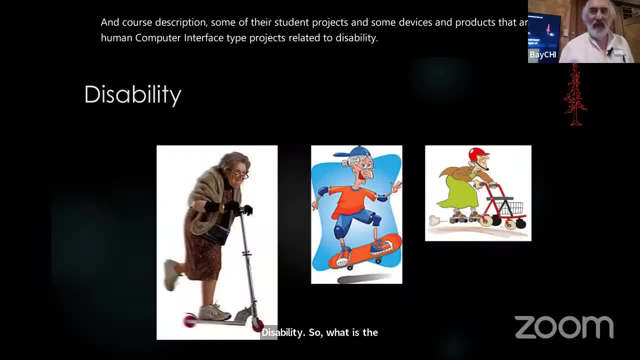 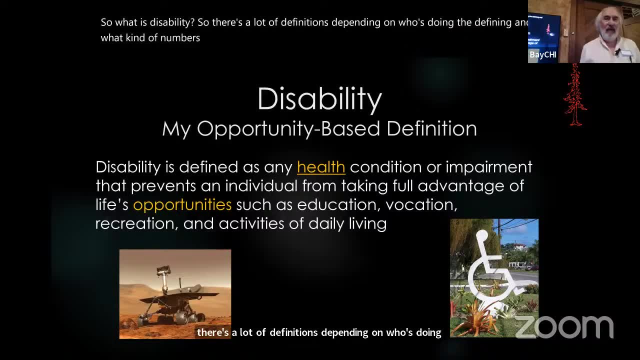 human computer interface type projects related to disability. So so you know there's a lot of definitions depending on who's doing defining and what kind of numbers they want. But you know my opportunity-based definition, that defined as any health condition or impairment that prevents an. 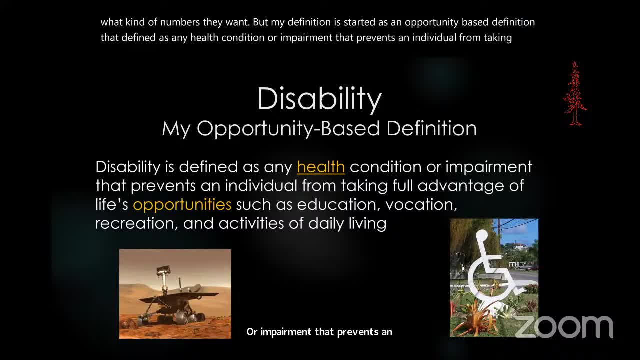 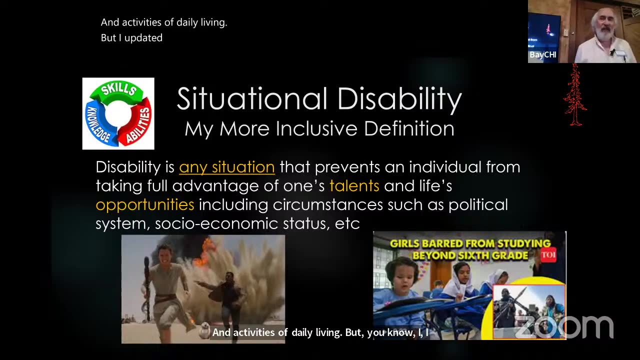 individual from taking full advantage of life's opportunities such as education, vocation, recreation and activities of daily living. But you know, I updated my definition of disability to not just a health condition but any condition that prevents any individual from taking full advantage of one's talents and life's opportunities. 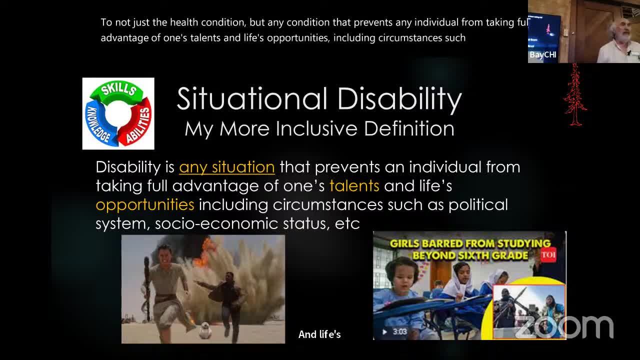 including circumstances such as the political environment and socioeconomic status. You know, for example, if you're on a planet that's under attack by the empire, right, you know your talent as a- You know a classical pianist. you know may not come into play, But you know closer. 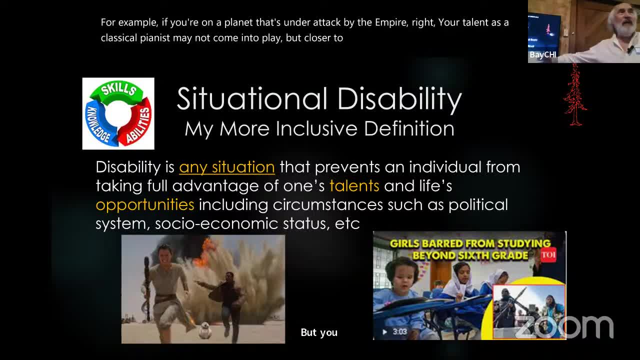 to reality. you know, in Iran, you know girls don't go to school after sixth grade. You know they're barred from school. So just being a female gets you out of school. So there's being a female. Is that a disability there? I would say so, But a more inclusive. 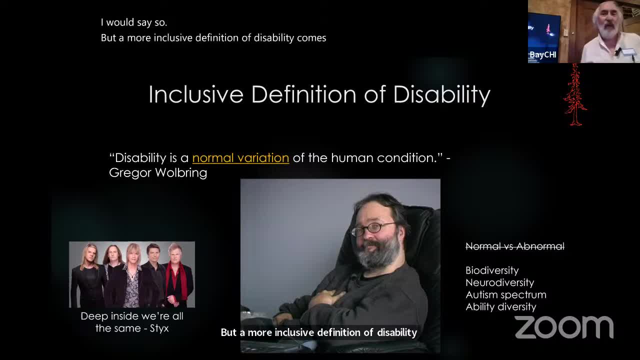 definition of disability comes from my colleague Gregor up in Up in Canada, And he says that disability is a normal variation of the human condition. Well, why should that be the case? Well, there's so many people with a disability and you'll see. 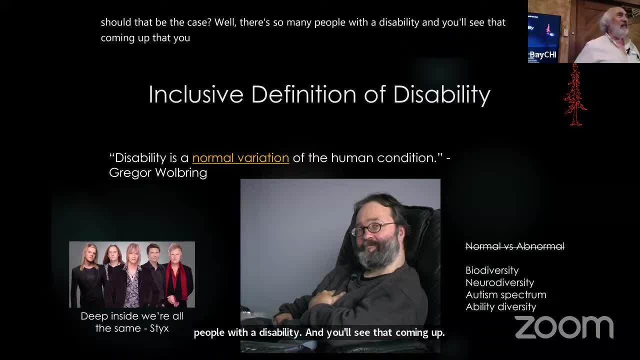 that coming up, that you know you can't, They're not a minority anymore. So this idea of you know, this binary difference between able-bodied and disabled, you know doesn't exist. So there is nothing, you know, akin to normal versus average, And I think that's a. 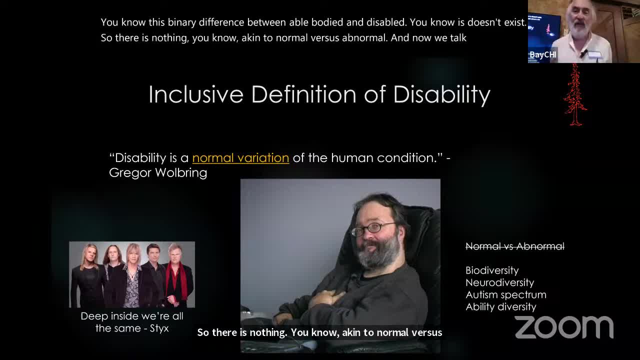 normal. And now we talk about a lot about biodiversity, neurodiversity, the spectrum of autism And also, you know, maybe there's a thing called ability diversity. that goes along with this as well. And as the rock group, All right, All right, I hope you can hear me. All right, Well now? no, I can't. 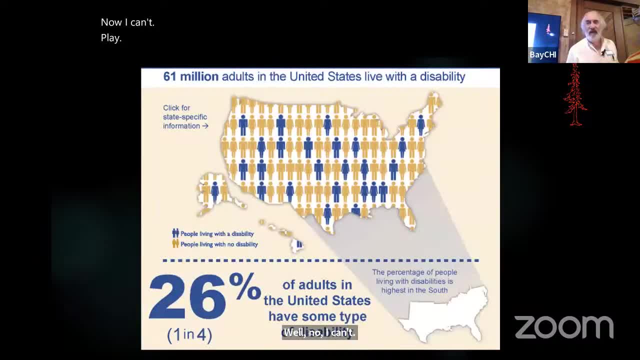 Okay, All right. So you know, here's a map of the US And according to this data, there's 61 million adults in the US with a disability, which is like 26%, So that's one in four. So that's hardly a minority. There are some, you know, people with some kind of disability. 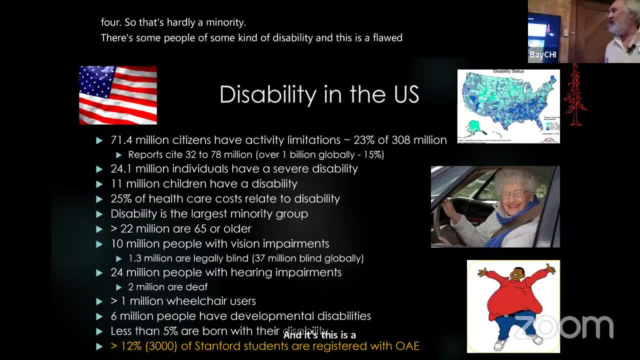 And this is a slide that I use in class. So, depending on how you count, there's millions of people in the US And there's a lot of people in the US, And there's a lot of people in the US. 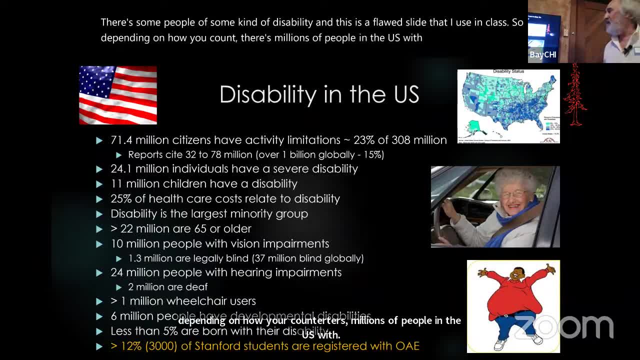 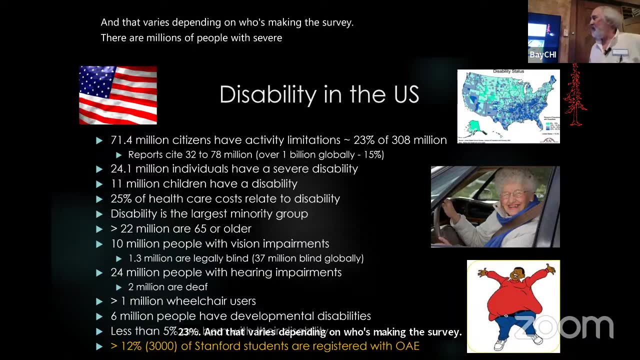 with activity limitations, which is, according to this, 23%, And that varies depending on who's making the survey. There are millions of people with severe disabilities. Children have disabilities. Health care costs related to disability is pretty high. Disability is the 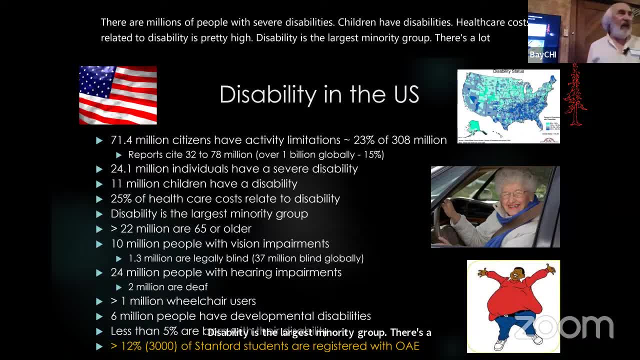 largest minority group. There's a lot of people that are over 65, including myself, that might have a disability. There's people with vision impairments, hearing impairments, There are wheelchair users and people with developmental disabilities, But less than 5% of people are born. 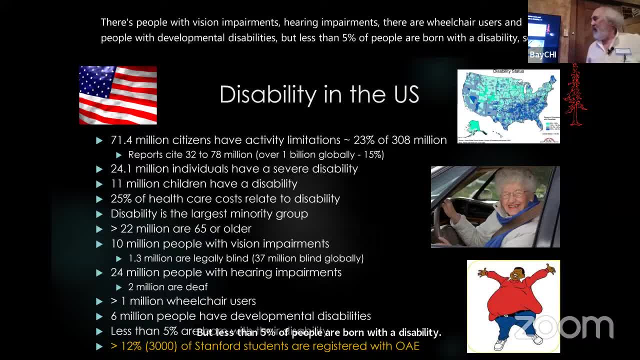 with a disability, So it's acquired after birth. And when I have this slide at Stanford, I note that 12% of the Stanford students are registered with the Office of Accessible Education with some kind of disability, And that's a lot of people. So that's a lot of people. So that's a lot of. 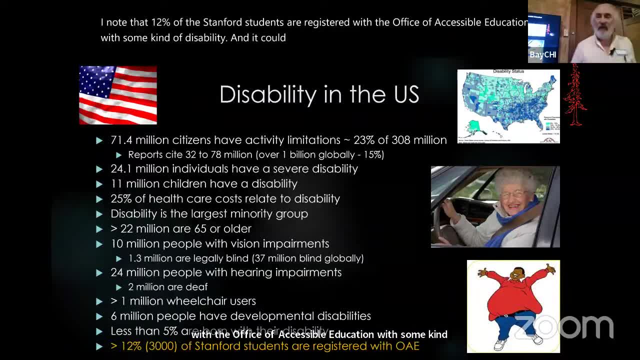 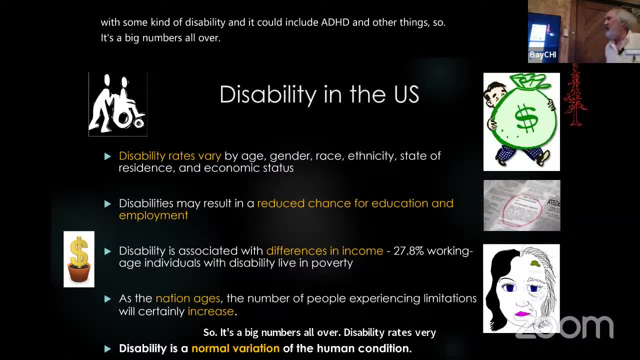 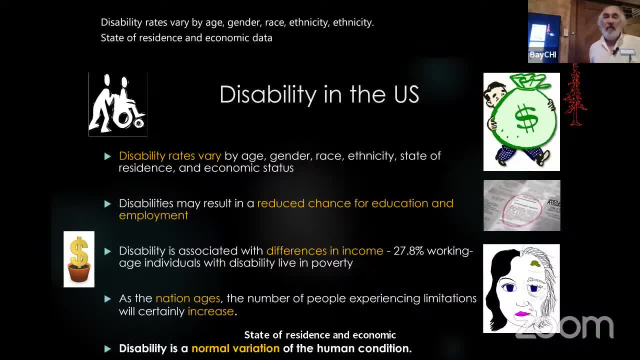 status. So a person with a disability may have reduced chance for education and employment, And that's really critical because if you don't have an education, you can't get a job. Some of your kids are at, You know, Israel, Yeah. 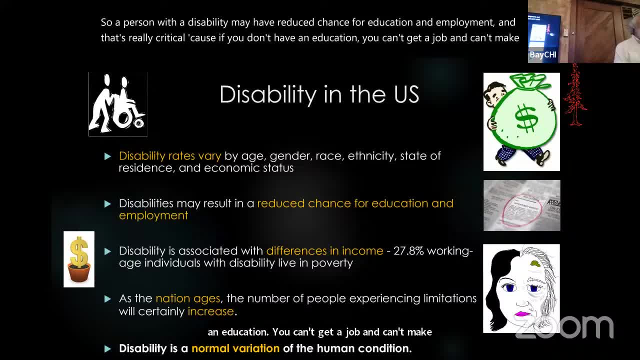 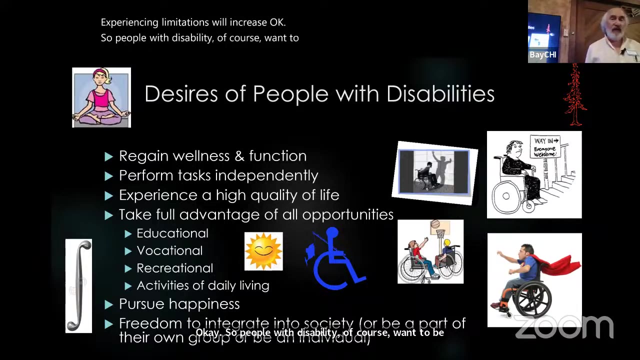 job and can't make money, And so you're living in poverty, and that's not good at all. And as people age, the number of people experiencing limitations will increase. Okay, So people with disability, of course, want to be well and be fully functional. They want to. 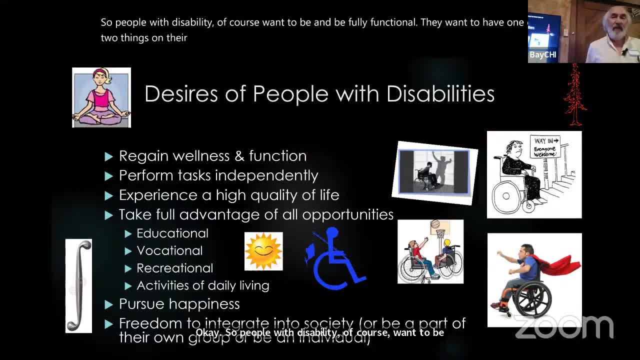 have want to do things on their own, have be independent, have a high quality of life and take full advantage of all of life's opportunities And, of course, pursue happiness and have the freedom to integrate, you know, fully into society or be a part of their own little group. It's 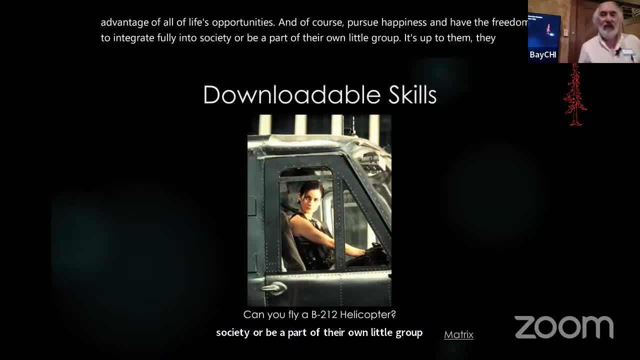 it's up to them. They have the freedom to do that. So I bring up this slide, and everybody remember Matrix, Remember this scene where they said: you know, can you fly a B-212? Helicopter? And what do they do? They stuck a probe back in in the guy's head And within. 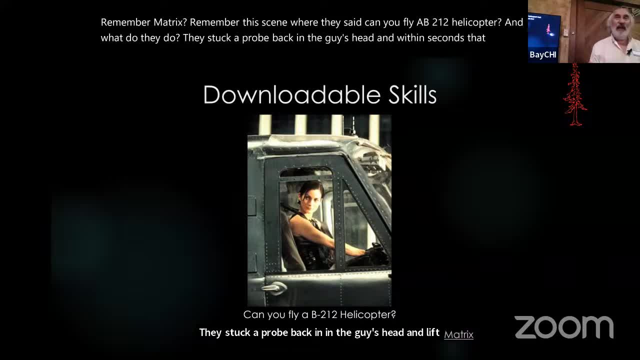 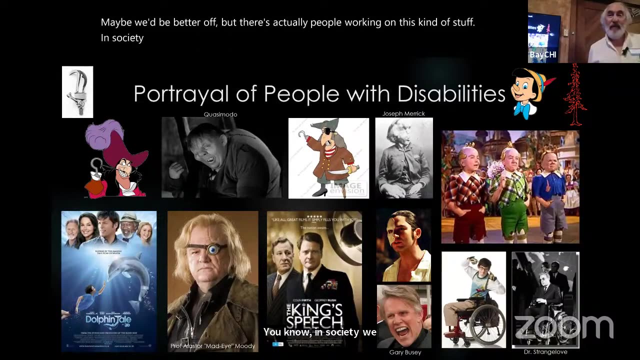 seconds. that information, that skill was transferred to that individual. If we can only do that now, maybe we'd be better off, but there's actually people working on on this, this kind of stuff. You know, in society we had there's a lot of people with disabilities and 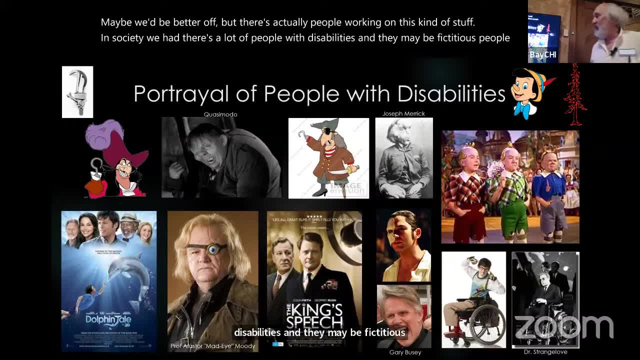 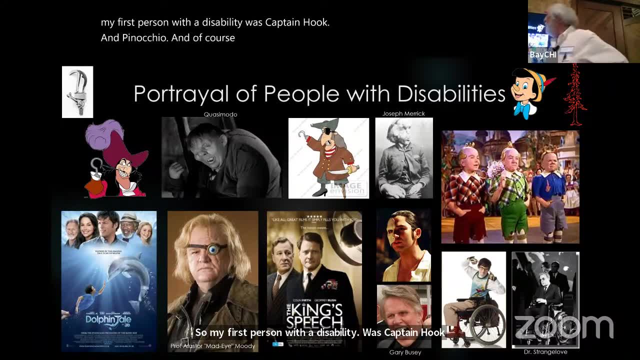 they may be fictitious people. So my first person with a disability was Captain Hook And Pinocchio, And of course you have Quasimodo from the movies. You know he went to Notre Dame, you know, which is in South Bend, Indiana, Right And, and I guess, being a pirate, you know. 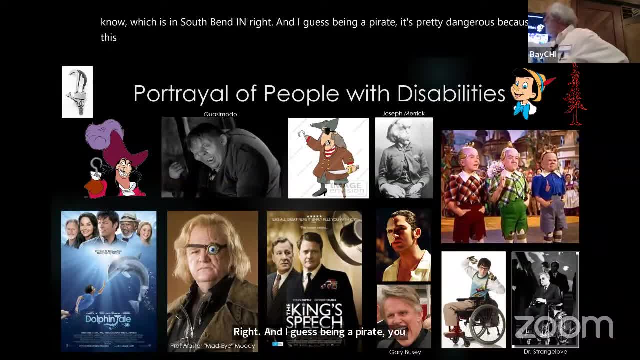 is pretty dangerous because this, this guy has a hook and a peg leg and an eye patch. So that's, that's tough. And Joseph Merrick, what? what was his name? The Elephant Man Right, And what was his? 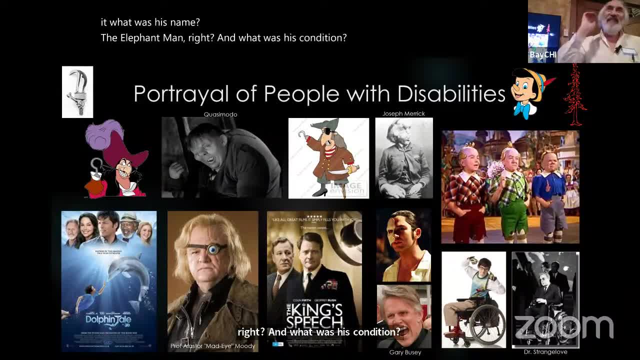 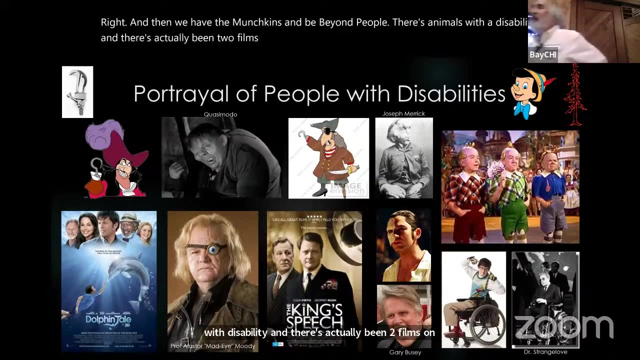 Condition. It's elephantitis, Right, And then we have the, the munchkins, and you know, beyond people, you know there's animals with a disability and there's actually been two films on this dolphin that they made a prosthetic. 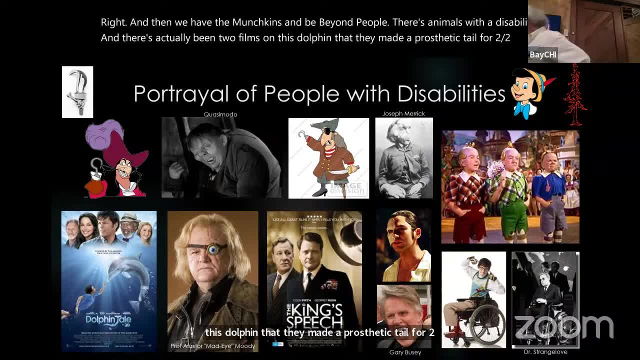 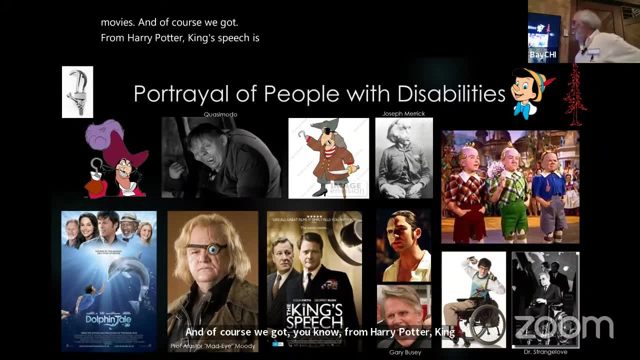 tail for Two, two movies. And of course we got you know from: Harry Potter King's Speech is a real movie about a person. Yeah, Yeah, Harry Potter King's Speech is a real movie about a person who died in the war, who was murdered by a猴 and the eagle. Yeah, It's really good. I love it. It's good And you know I love. I love the title. The elephantman is about nothing. It's a beautiful抱ie, Yeah. 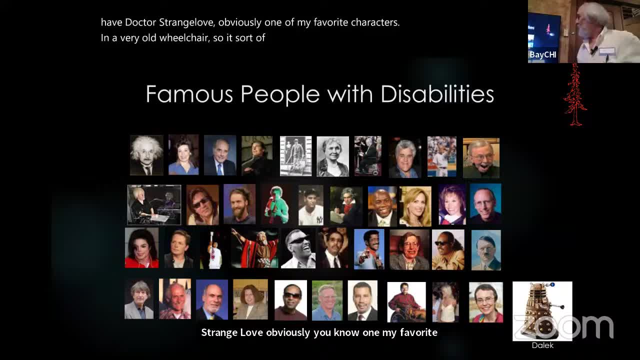 It's good. Yeah, Yeah, It's great. It's a beautiful book. It sort of permeates society. You know, here's some more people, And every year I add more to this list. So we got: we got Moses here, We got Helen Keller, We got Jay Leno. We have Hitler, We have. 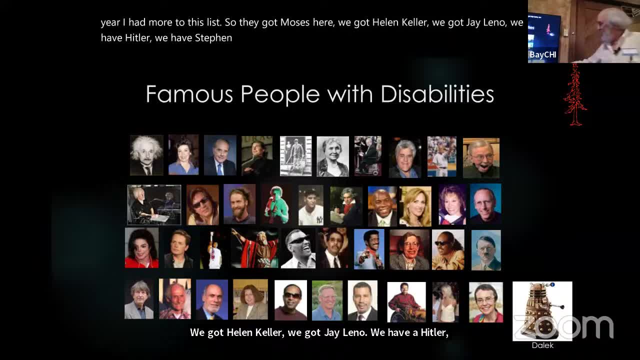 Stephen Hawking, And, of course, you know the, the, the Daleks, you know from Doctor Who, you recall, you know this is, this is a, an alien who, uh, needs protection. he can't, you know, walk outside, so they created an exoskeleton, you know, before him, and an exoskeleton is assistive technology. okay, 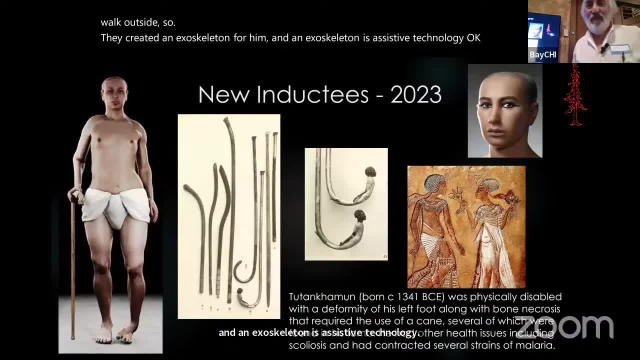 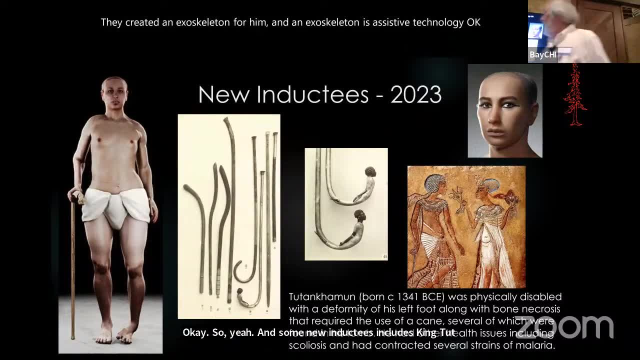 so yeah, and some new inductees includes uh king tut, who um was. they did a scan of him and they found that he had um deformity of his left foot, and in this tomb they found all sorts of canes and there's even even carvings of him, and here's the recreation of them. so disability goes, goes. 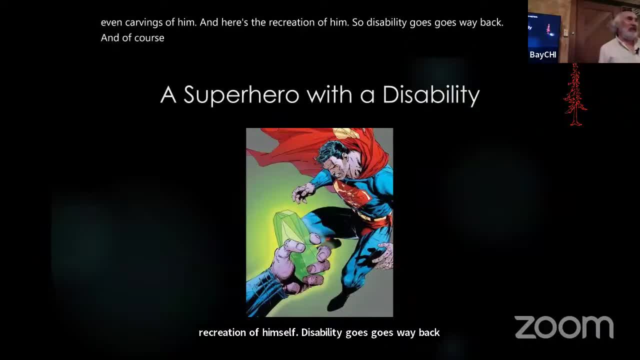 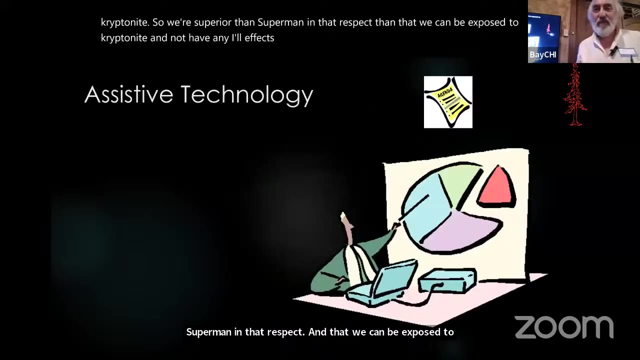 way back. and, of course, even super superheroes have a disability, as you know, superman and exposed to kryptonite. so we're superior than superman in that respect, and that we can be exposed to kryptonite and not have any ill effects. right? so let's talk a little bit about assistive technology. 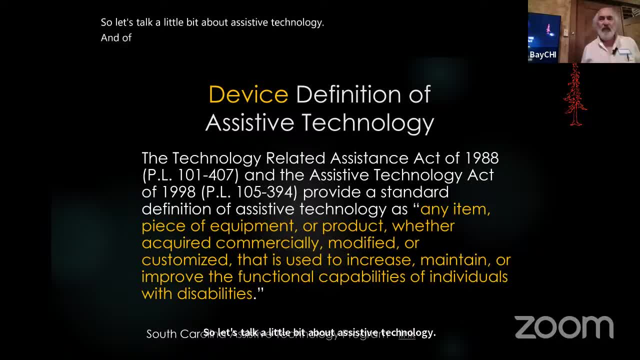 and of course, the definition is the first thing. so people usually think of assistive technology as a device oriented- uh definition where it's um- as any piece of equipment or product, whether acquired or commercially available, or modified or customized, that can be used to increase, maintain or improve the functional capabilities of individuals with with disabilities. 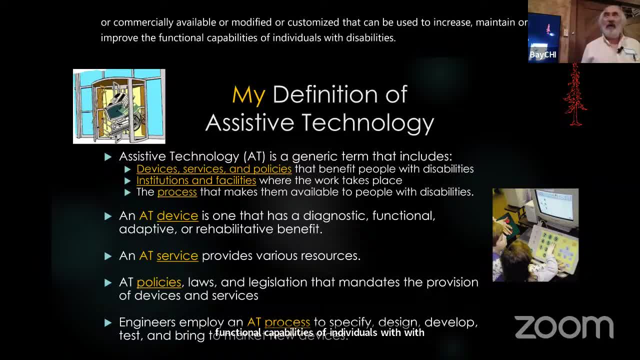 but my definition is obviously broader, which includes not only devices, but services and policies that benefit people with disabilities, and institutions and facilities, um, uh, where, where that work takes place and the process that makes it happen. um, so, an assistive technology device is one that has a benefit, which could be a diagnostic benefit, a functional benefit or a rehab benefit and an at. 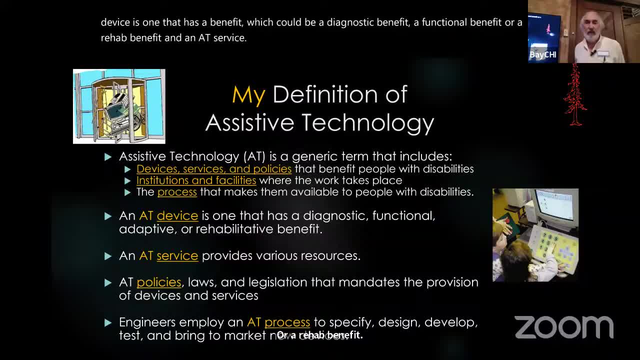 service, um, but the benefit is that it provides various resources to people with disabilities. and, of course, at policies, laws and legislation, you know um are things that mandate the provision of these devices and services. okay, and engineers employ um an assistive technology process to specify, design, develop, test and bring to market these new devices. so um. so eight assistive technology devices, then. 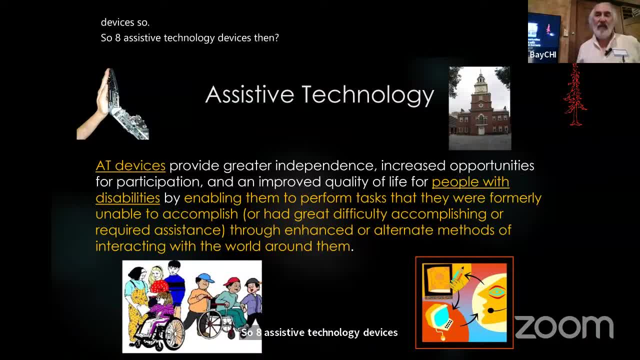 um improve the quality of life and independence of people with disabilities by enabling them to perform tasks that they were formerly unable to accomplish or had a great deal of difficulty accomplishing, or required assistance, through an enhanced, alternate method of interacting with the world around them. That's pretty straightforward, But I realized that the devices that we use 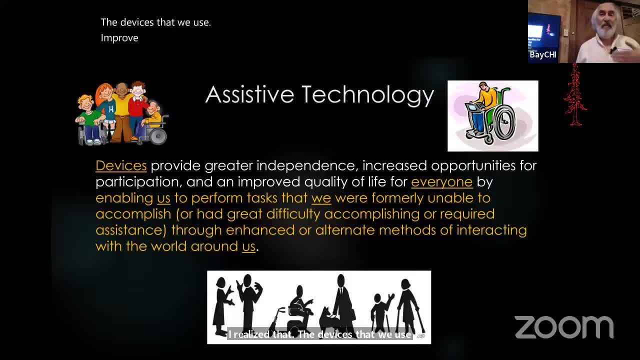 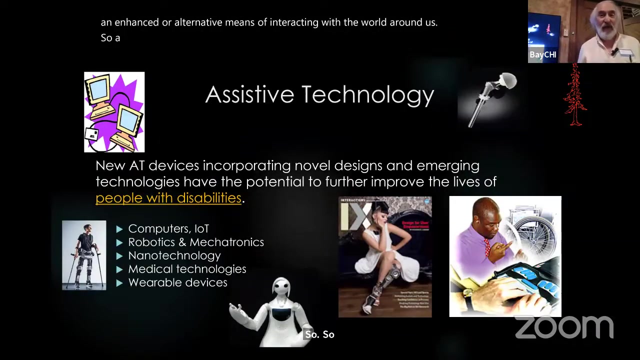 improve our quality of life in the same reasonings, by enabling us to perform tasks that we were formerly unable to accomplish or had difficulty accomplishing, or required assistance through an enhanced or alternate means of interacting with the world around us. So a couple more things before I get to the point here. So there is new devices being developed, all. 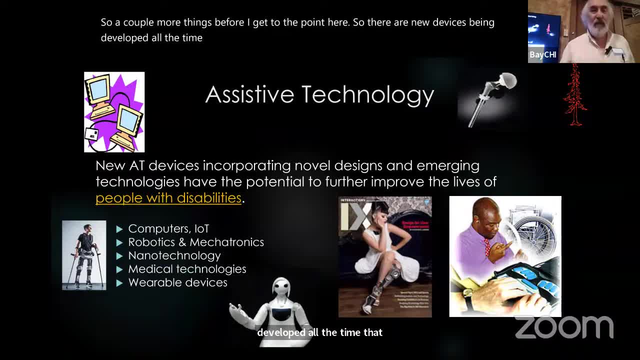 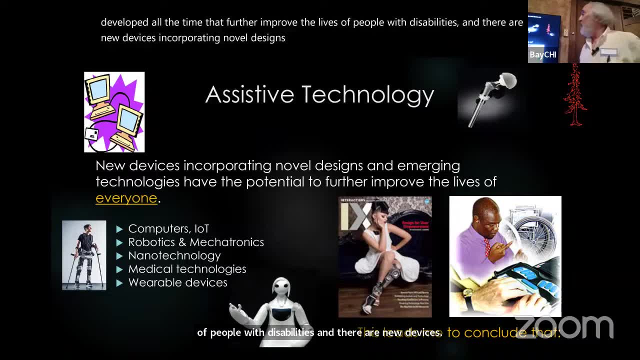 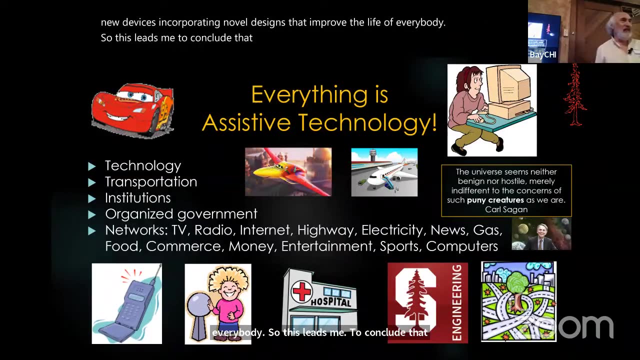 the time that Further improve the lives of people with disabilities, And there are new devices incorporating novel designs that improve the life of everybody. So this leads me to conclude that everything is assistive technology. okay, Because I mean we're okay. we're like cavemen, you know. 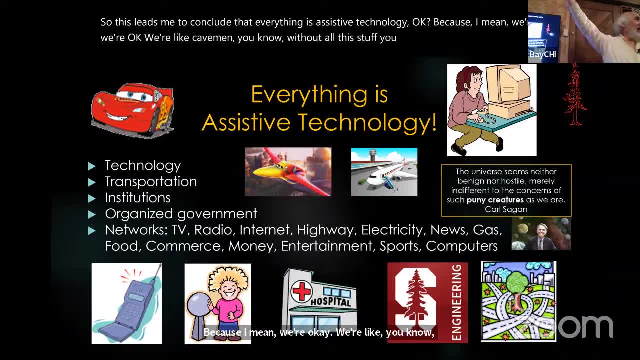 without all this stuff. you know we're pretty disabled, right. And so I mentioned, you know, computers and cars and airplanes And phones and electricity, hospitals and roads and stuff. And I asked my students what's the most awesome piece of assistive technology? And the answer is Stanford University. Now, when I'm 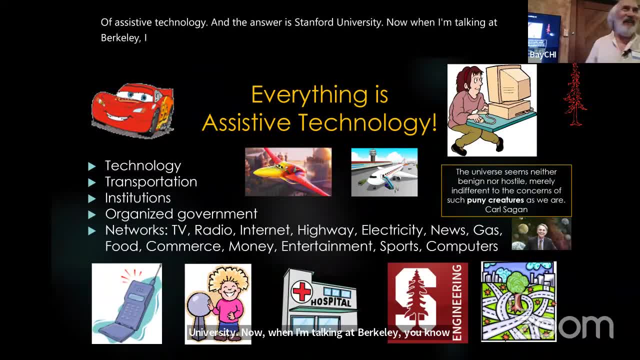 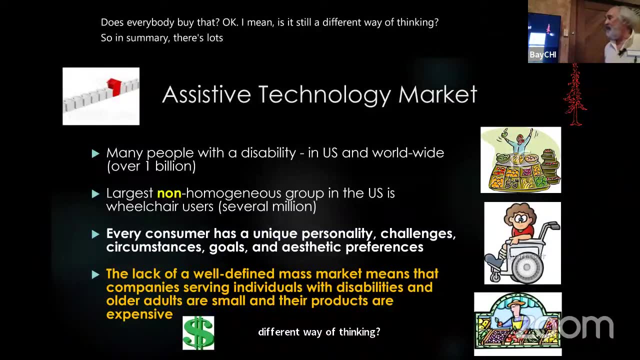 talking at Berkeley. you know, I substitute, you know their logo in there, because I don't want to get into too much trouble. okay, Does everybody buy that? okay, I mean, it's just a different way of thinking. So, in summary, there's lots of people in the US and worldwide- over a billion, you know- with a 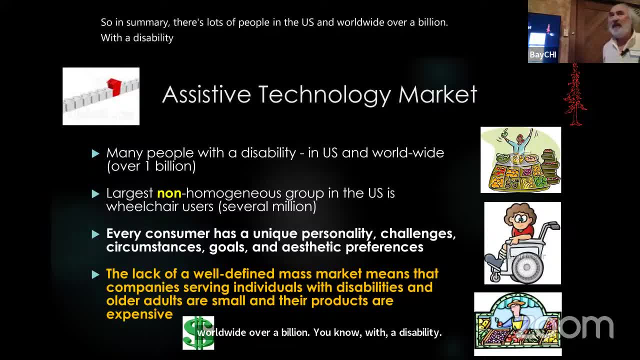 disability And wheelchair users. you might think, there being several million, might be a homogeneous group of people because they all use wheelchairs, But it's not because every wheelchair user in in that I've seen you know have has different requirements, needs for their 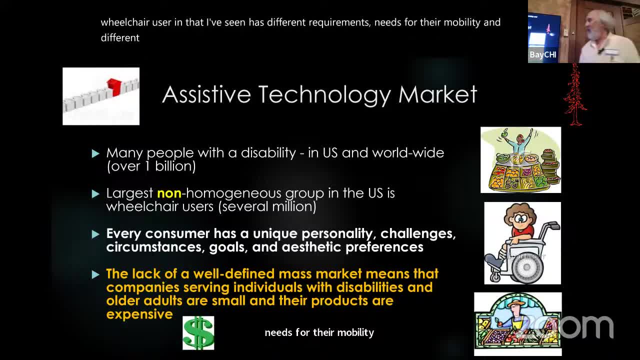 mobility and so on, And so you know, I think there's a lot of people in the US and worldwide, you know, with a disability and different preferences, goals in life and aesthetic preferences and different challenges. So so what I'm trying to say here is that, even though 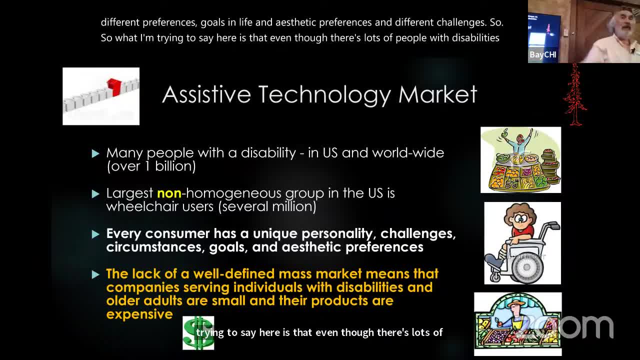 there's lots of people with disabilities and you might think that's a huge market to address. it's actually fragmented down to the individual And this was what makes provision of you know products- assistive technology, project products- expensive and the companies that produce. 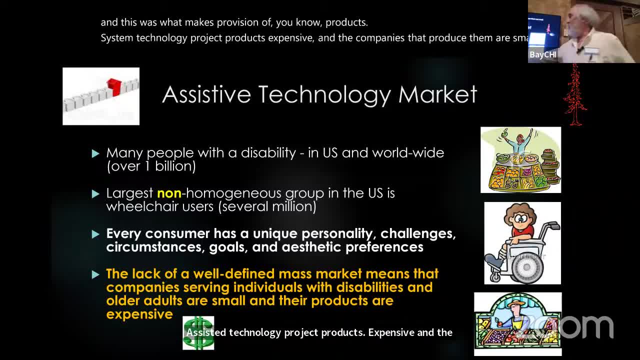 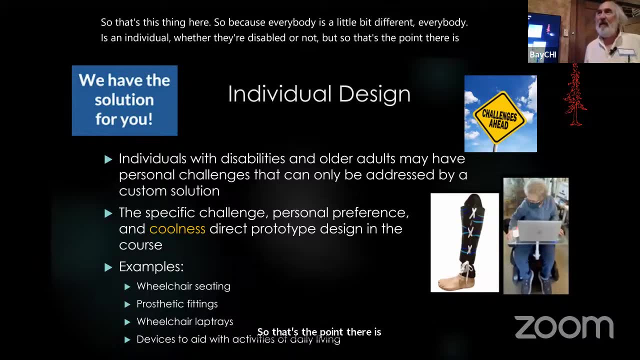 them are small. So so that's this thing here. So you know, because everybody is a little bit different, Everybody is an individual, whether they're disabled or not. But so that's the point. there is that it's hard to address this market because everybody has a little bit different. 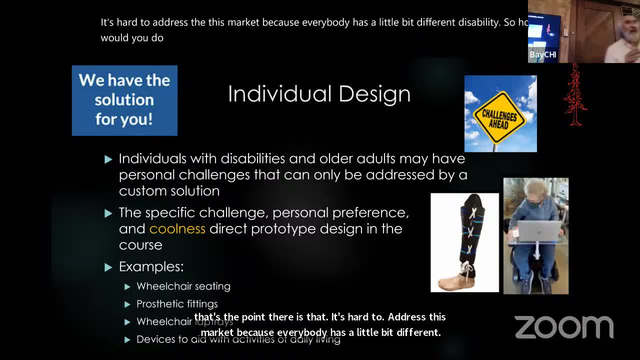 disability. So how do you, how would you do that? So I brought, I created this concept called individual design. So because individuals with disability have their own personal challenge that may only be addressed by a custom solution. So some of that- examples of that are, you know. 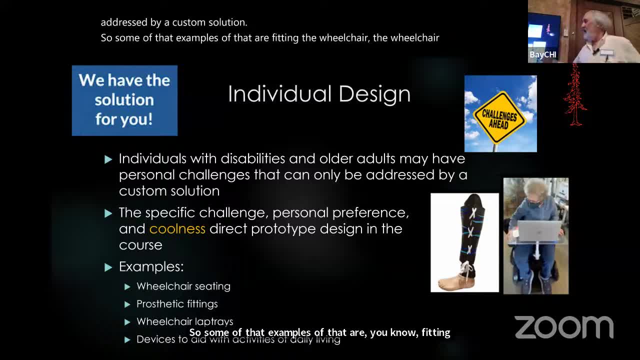 fitting the wheelchair, the wheelchair seating, prosthetics, lap trays and devices to aid people with in activities of daily living. And, of course, a big thing that people have is the sense of coolness of something Everybody. there are so many decisions that people make unknowingly that you know, for our clothes and 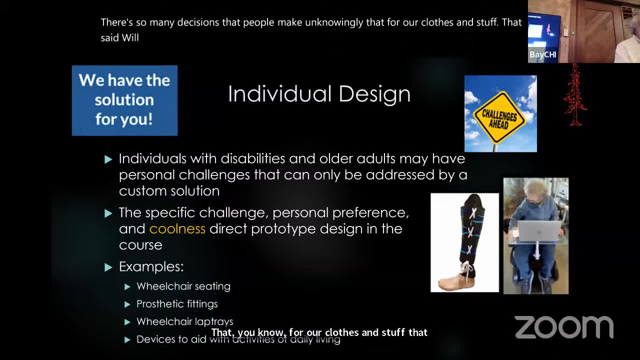 stuff that said: you know, will this look cool? you know, for me do I like this color on my car, Do I like this car because it looks cool, and stuff like that. Everybody makes these decisions every day, So the coolness factor is actually a pretty important thing, not only in assistive 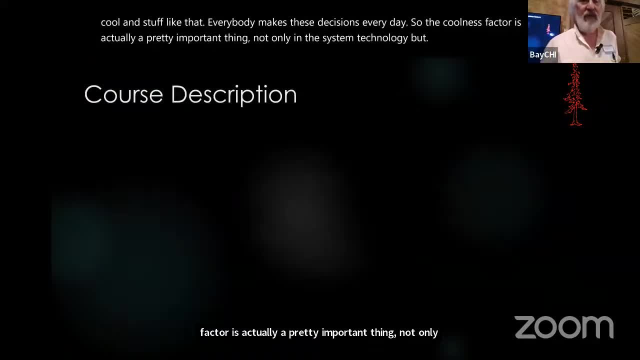 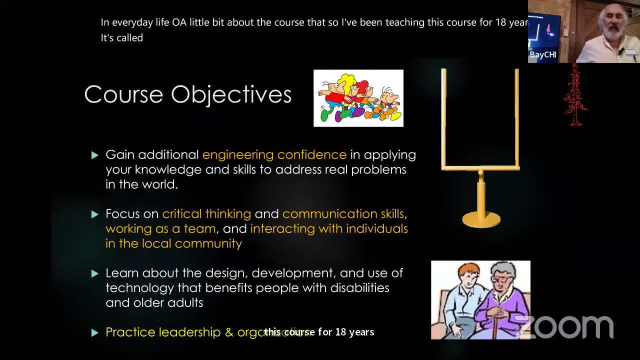 technology, but in everyday life. So a little bit about the course that. so I've been teaching this course for 18 years. it's called Perspectives in Assistive Technology, And so the objectives for the students is for them to gain additional engineering confidence applying the knowledge. 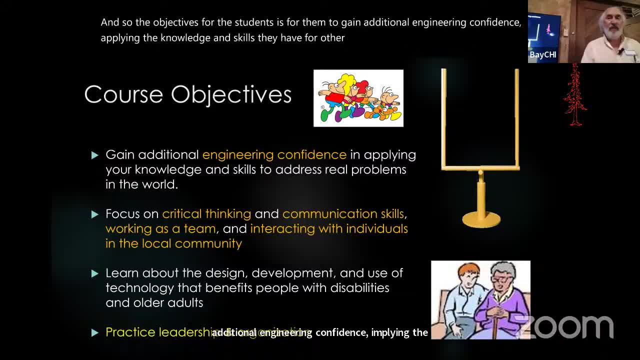 and skills they have for other courses in addressing problems that people with disabilities experience. So I try to focus on having the students do critical thinking and enhancing their communication skills, working as a team, interacting with individuals- and, you know, individuals in the local community- And these are things that everybody needs to do. These 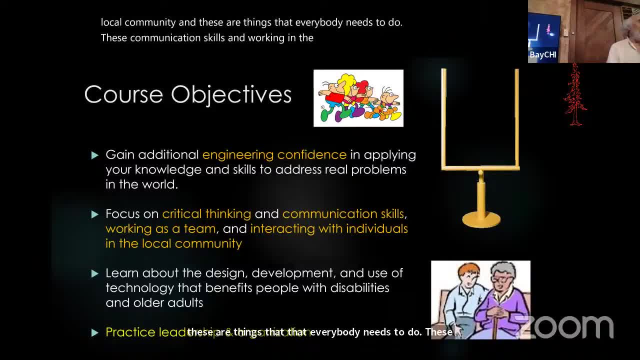 communication skills and working in a team and solving problems are things that everybody does on their job, right, So I try to give them these kinds of skills in this class. They certainly learn about the design, development and use of technology that benefits people. 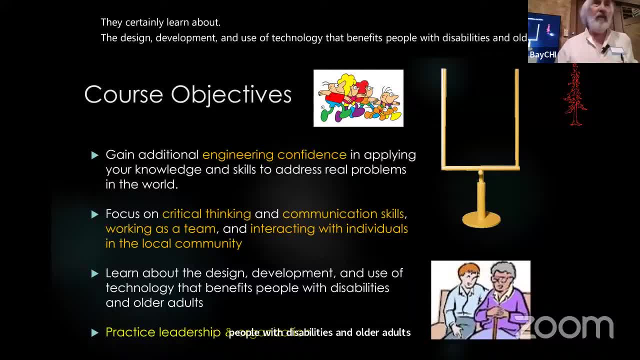 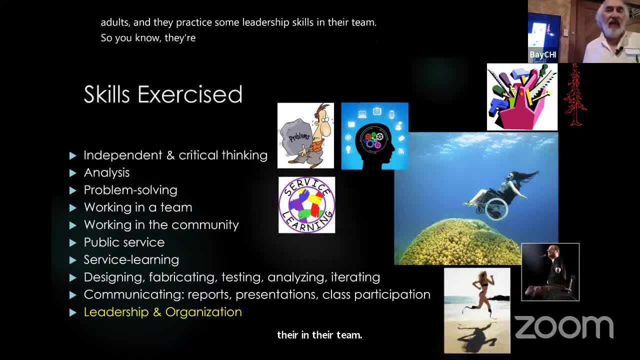 with disabilities and older adults And they've practiced, you know they've practiced, you know some leadership skills in their team. So you know they're given a problem, they have to analyze it, they have to do problem-solving, they have to work in a team. they're working. 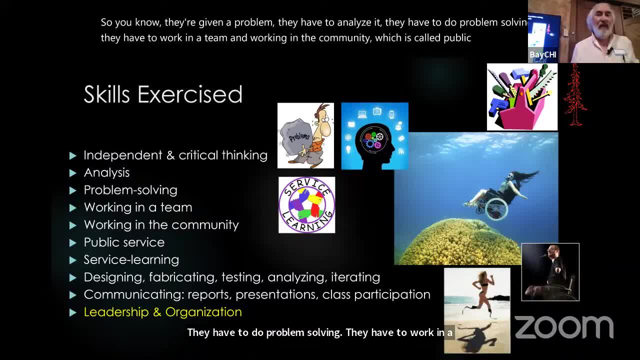 in the community, which is called public service and it's also called service learning, And they go through a design process which includes designing, fabricating, testing, analyzing and iterating until meeting, until they meet all of the design goals. 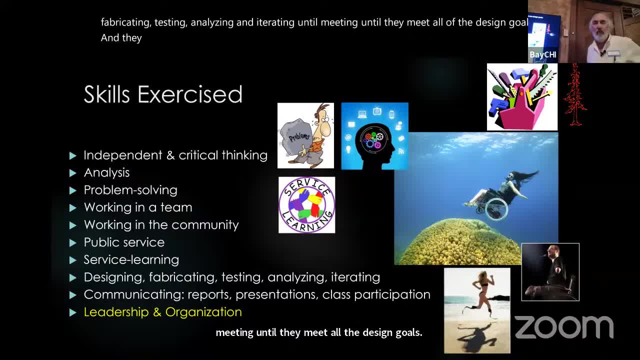 And they enhance their communication through reports, presentations and class participation. because nobody told me, as an engineer when I went to school that communication skills were important, right? Did any of your instructors tell you that when you went to school? So I mean, what did you think? That you, as an engineer, you know, wouldn't have to do things? 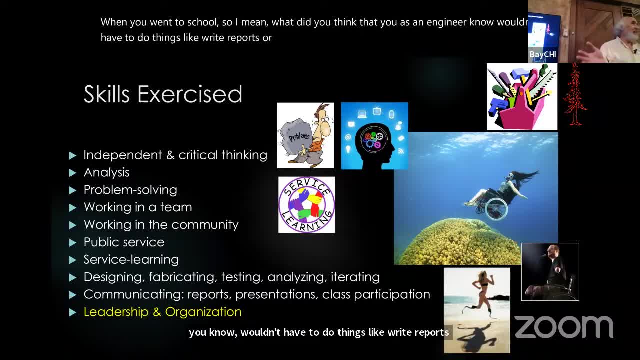 like write reports or doing presentations Or talking at bake high. You know they didn't know right. So I mean it's really important, So I mean I focus on that in my class And, of course you know, going having leadership. 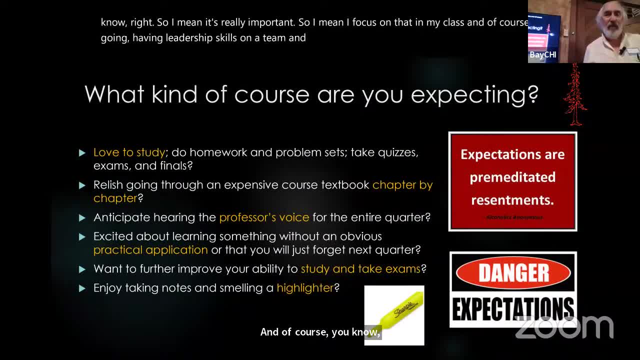 skills on a team and organizing their project is really important. So my course is a little bit different. There's no studying involved, There's no quizzes, no problem sets, no exams and finals or finals. So the students get graded. 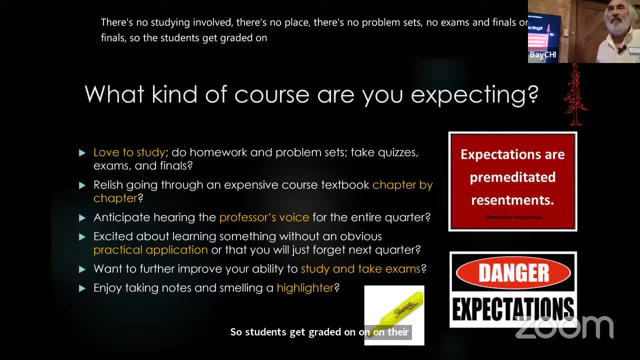 On their reports, their presentations and their project. So we don't. there's no textbook. So remember when you were in school you bought a textbook and say: today we're going to do chapter three And on the back of the chapter we're going to do these problems. 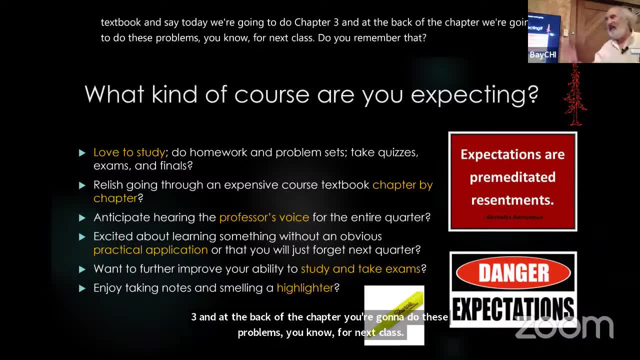 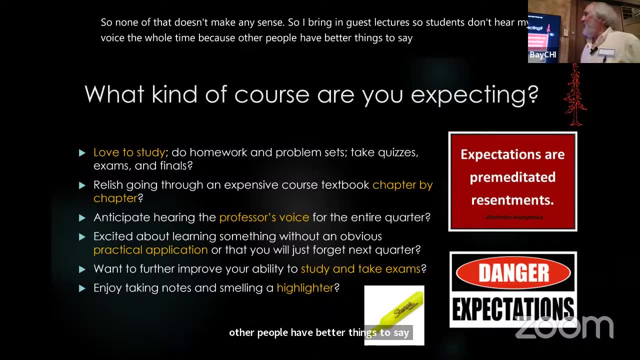 you know for next class, You remember that. So none of that. That doesn't make any sense. So I bring in guest lecturers so students don't hear my voice the whole time, Because other people have better things to say And I want to get students excited about. 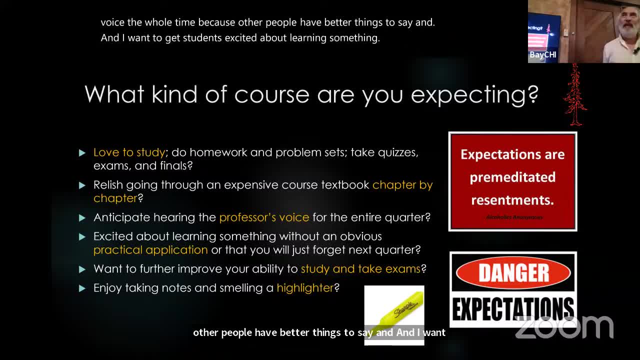 learning something that may have a more practical application than some of the courses that you took. I mean, think about all the courses that you took that you've never used anything from them. That's a lot of stuff, right, Never used. okay, Students don't need to, you know. 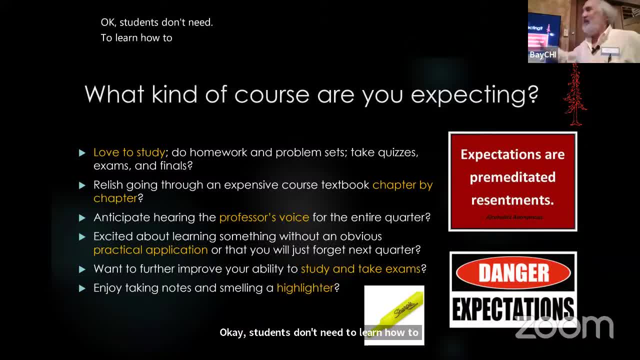 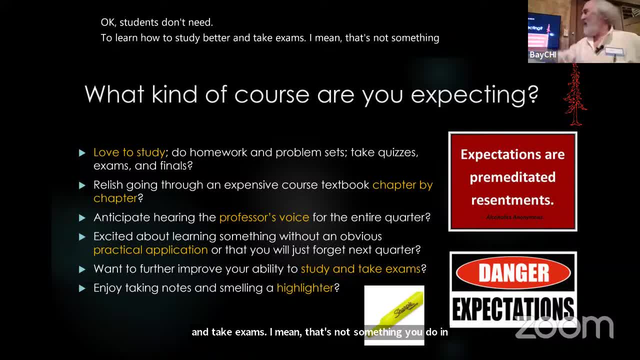 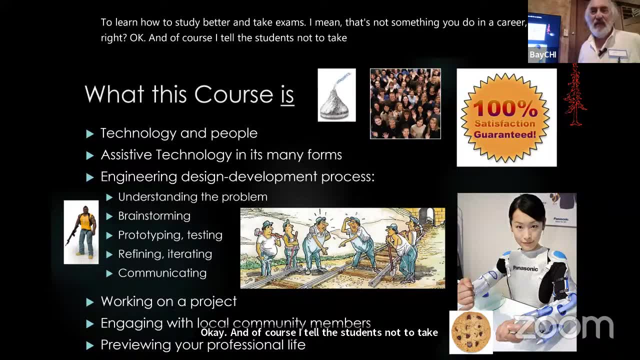 I mean, that's not something you do in a career, right, Okay? And of course, I tell the students not to take notes, Just to be attentive. So the course is about technology and people, assistive technology in many forms, and going through this design development process. I'll. 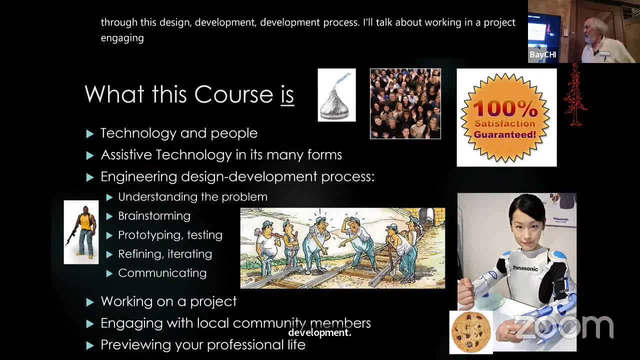 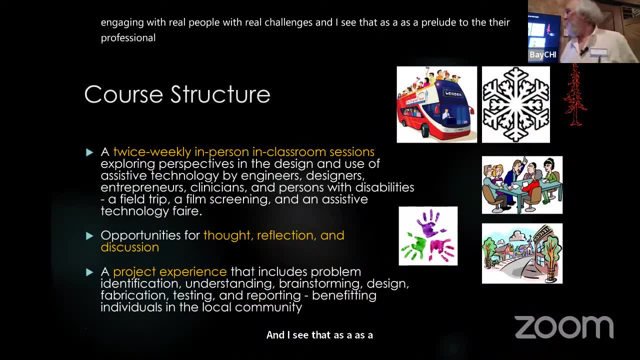 talk about working on a project, engaging with real people with real challenges, And I see that as a project that I'm working on to build the course And I see as a project as a prelude to the their professional life. okay, so the course structure: it meets twice a week. 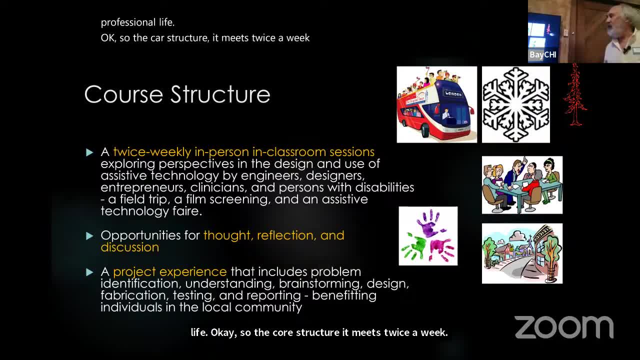 and I bring in guest lecturers to talk about various things. I'll talk about that a little bit later. there's opportunities for thought, reflection and discussion, and there's a project experience, which includes identifying a challenge, understanding it, brainstorming solutions, designing prototypes, testing them, reporting and things that that benefit a real 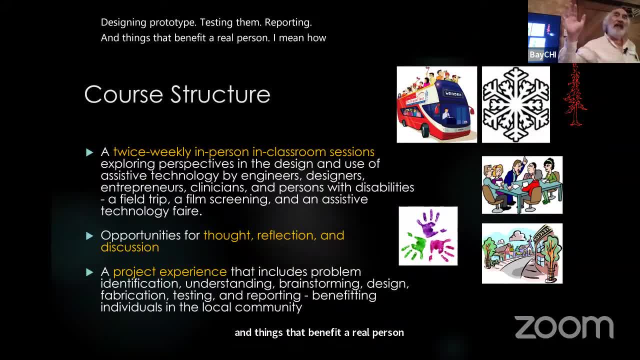 person. I mean, how many? how many courses did you take that involve real people from the community? probably anybody have any courses like that. okay, so the students really like the course because of this, because it you know it makes sense. they're doing something that's of obvious benefit to a real person and that makes it all you know, real world rather than you know. 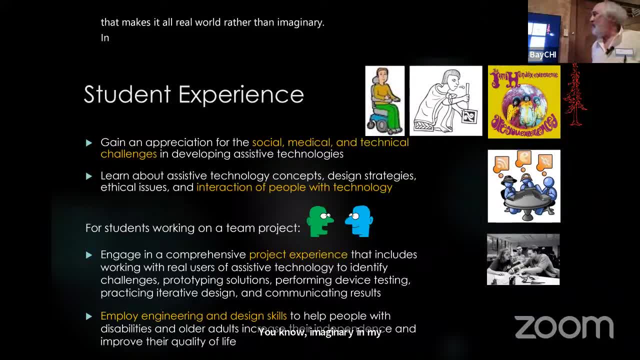 imaginary in my mind. so, uh, i talked about the project experience. that includes working with a person in the community, um, and prototyping solutions and testing it with them to make sure that it works, and going through the iterative cycle till they get to the end of the course. 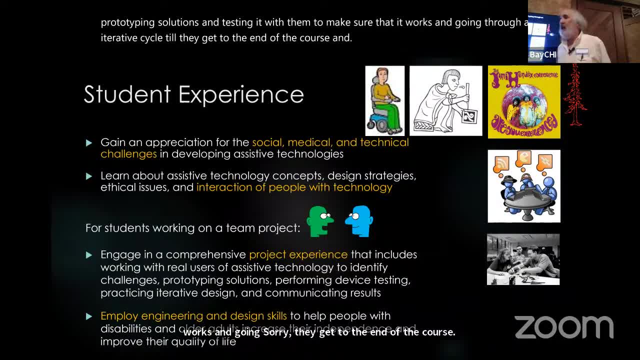 and um, and we have uh, midterm and end of term reports and presentations and at the very end we have project demonstrations that i'll show you some pictures from. so the students have an opportunity to employ the skills that they already have, and some of the students in the class 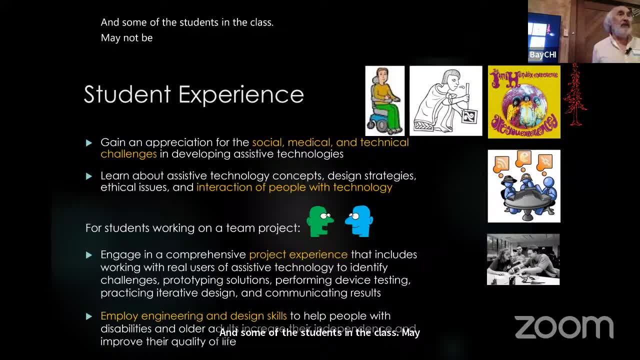 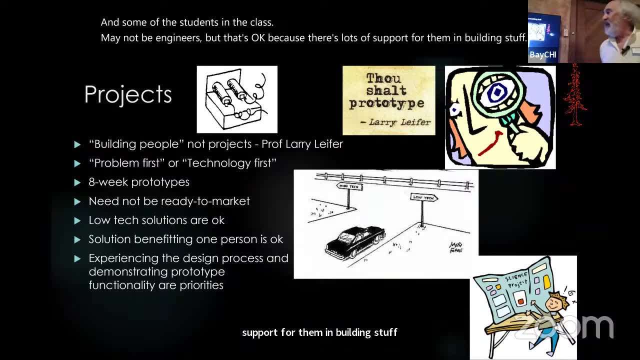 um may not be engineers, but that's okay because there's lots of support for them, uh in building stuff. so projects, uh are not just about you know building things, it's building people, building character, um, and you can um sometimes attack a challenge by um by starting with the challenge. 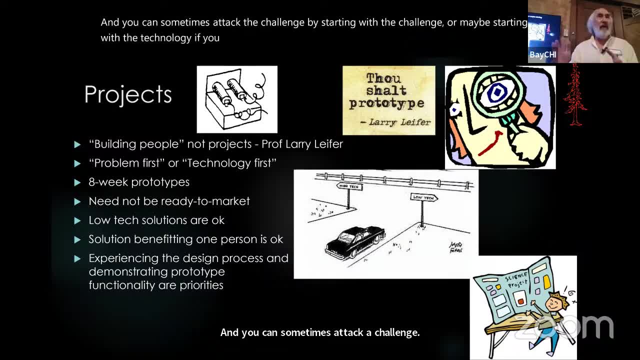 or maybe starting with the technology. if you have a new technology, you can say, hey, you know, this might really work, you know, solving this other problem. or maybe, before you even start, you can start by trying new things to solve a problem. or maybe i'd like to start with this particular problem. 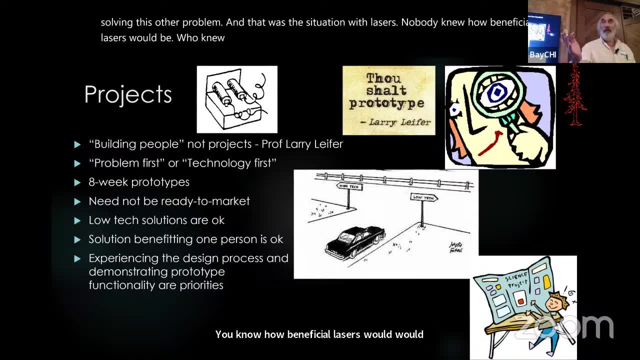 that was the situation with lasers. you know, nobody knew, you know, how beneficial lasers would would be. who knew that you can play music with lasers, right? so it's really important. so, um, i, i focus on, um, you know, a 10-week project. uh, so that what the students come up with is a 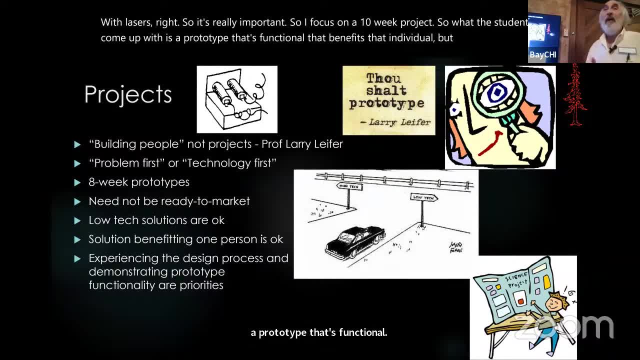 prototype that's functional, that benefits that individual. but i don't focus at all on We're working with one person and a solution for that one person may not extrapolate into a solution for other people because, like I said, everybody is different. So going through this design process is really important. 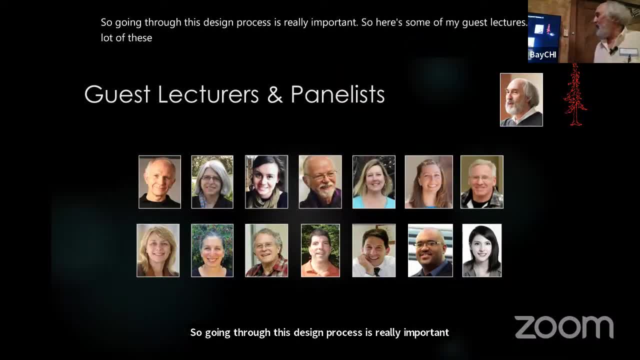 So here are some of my guest lecturers. A lot of these people I work with are from Stanford: a PhD candidate that's doing brain-computer interface, an occupational therapist and a design person. and a student who actually commercialized. She commercialized her student project way back when. 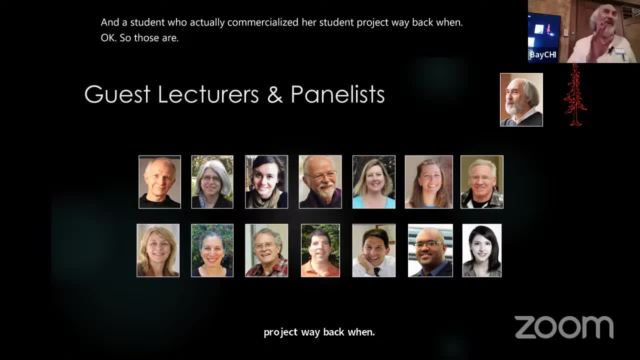 So I model each class session after the Tonight Show with Johnny Carson. So I get up and I do my monologue for like 10 or 15 minutes and then we have a little break and then the guest lecturer comes on and talks about these interesting topics. 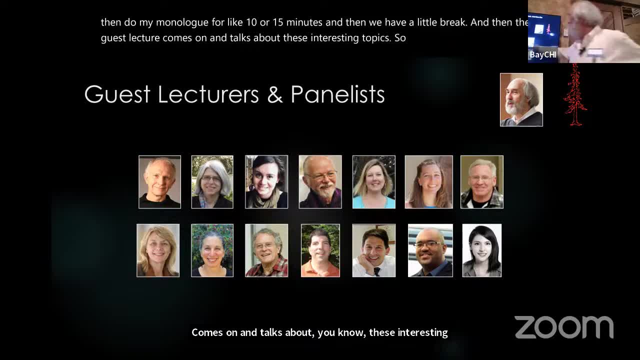 So yeah. So Peter here is. He's a person who's a wheelchair user and it turns out he was the first full-time student at Stanford who used a wheelchair, And so he's done some fantastic things in the area of disability, adaptive sports and stuff. 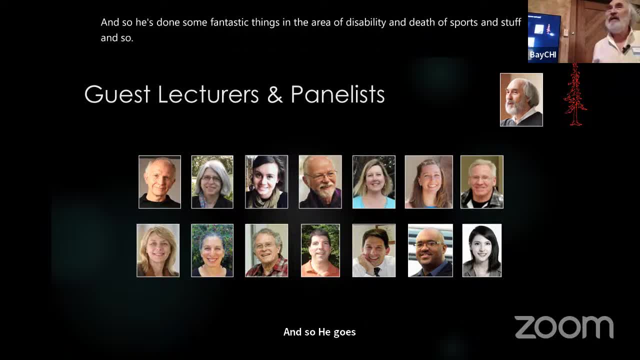 And so he goes through like 200 slides in an hour, And because I have him every year, he became so proficient at doing this. So I bring back the same guest lecturers because they get better every year, Although sometimes I have new people. 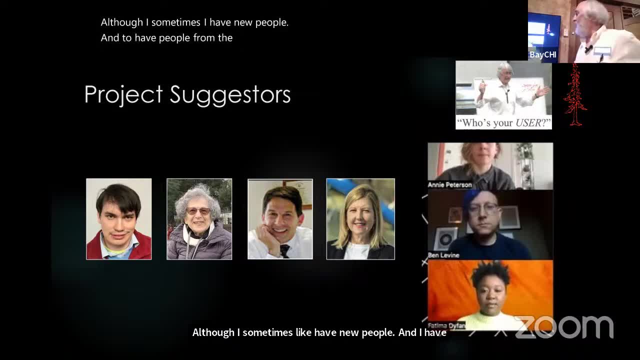 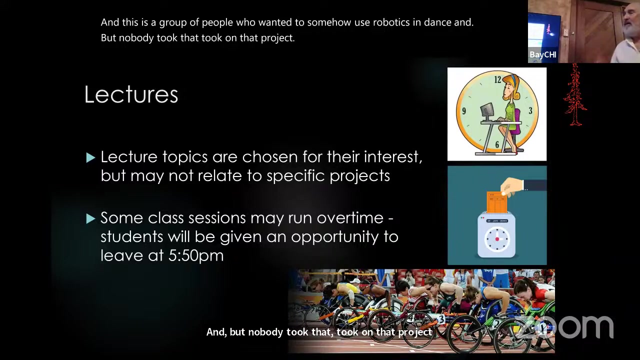 And I have people from the community who suggest projects either for themselves or their clients, And this is a group of people who wanted to somehow use robotics in dance, But nobody took on that. Nobody took on that project. Extra topics are meant to be interesting. 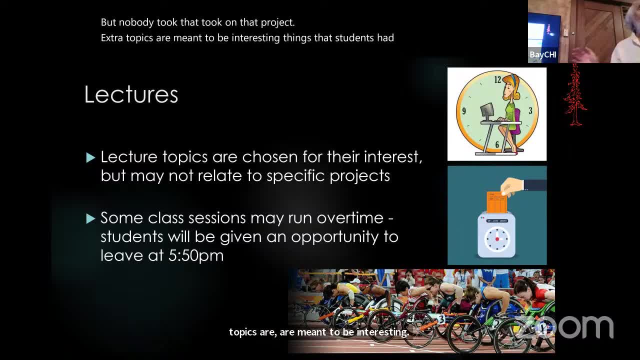 Things that students had never heard about before, like brain-computer interfaces, like exoskeletons, like prosthetics, like adaptive sports, like low-tech assistive technology, stuff like that. So it's all. I hope it's interesting to the students. 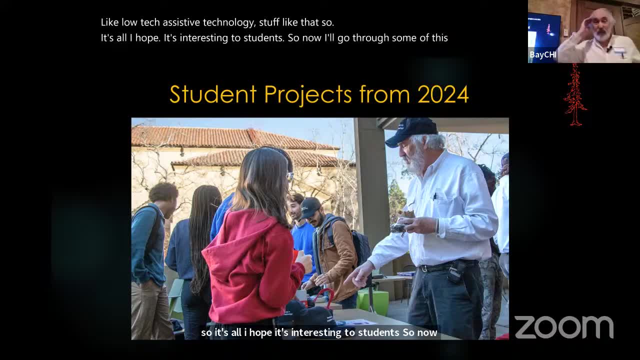 So now I'll go through some of this project, And this is from about three weeks ago. This is at the last class session where the students are given a table outside and set up their projects And I go around with my course assistant and we evaluate the functionality of every device. 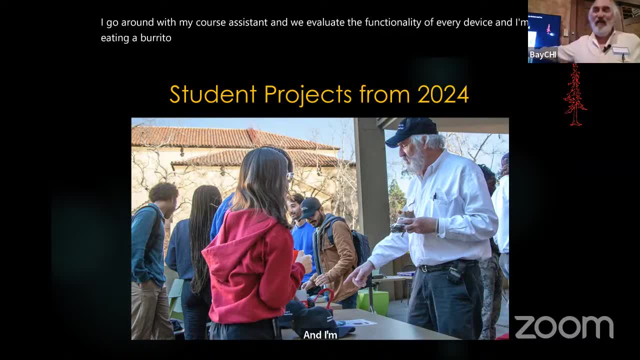 And I'm eating a burrito here. I bring in burritos for everybody, So it's a very low-key trade show. So it's a very low-key trade show-like atmosphere And the students get to see the other projects and get to ask questions. 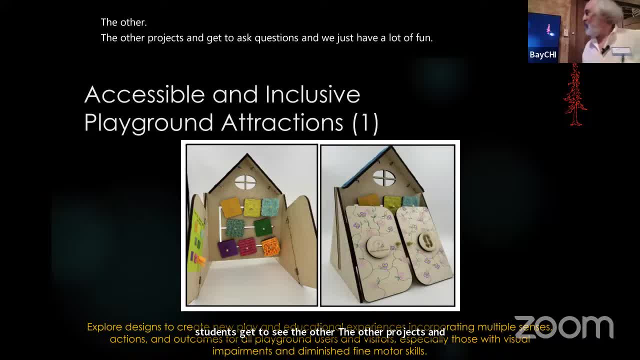 And we just have a lot of fun. And here's some of the things they worked on. So we work with the Magical Bridge Playground And they're always looking for new additions to their park. The Magical Bridge Playground is a playground that was designed from the bottom up to be accessible and inclusive. 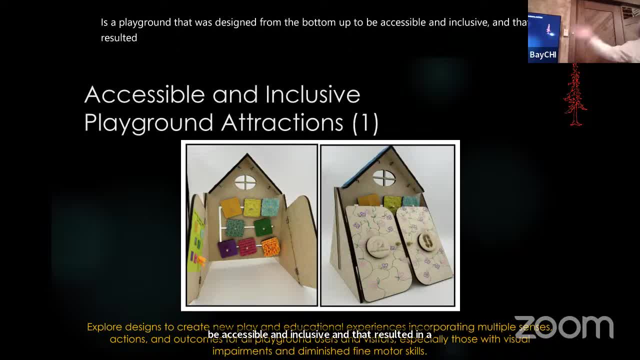 And that resulted. And that resulted in a playground that is so totally different than an ADA-compliant playground. So it's actually set a new standard by just wiping out what everybody else has done. So students are imagining other devices in there, including a device that they can open up and feel the textures, move things around. 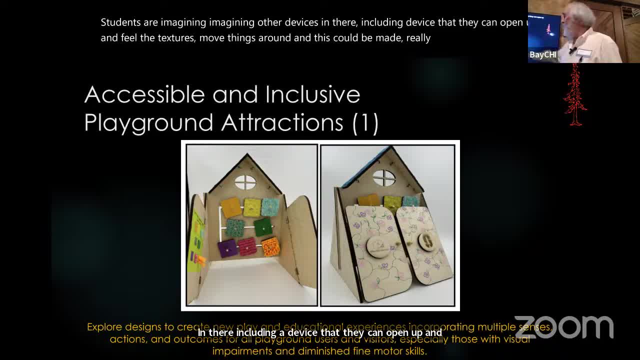 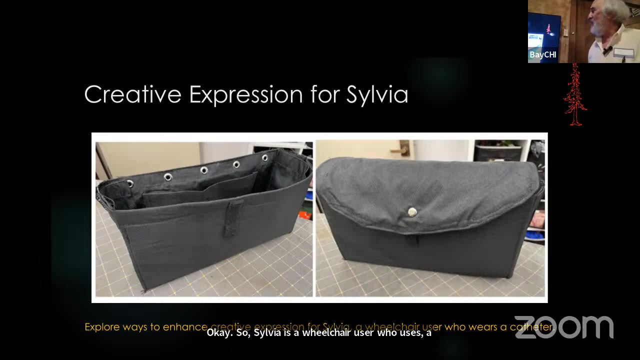 And this could be made really big and may provide shelter. And at the bottom of the slide is a wheelchair user who uses a catheter to start off their project. Okay, So Sylvia is a wheelchair user who uses a catheter, And so the students want to make a custom bag for her that looked aesthetically good. 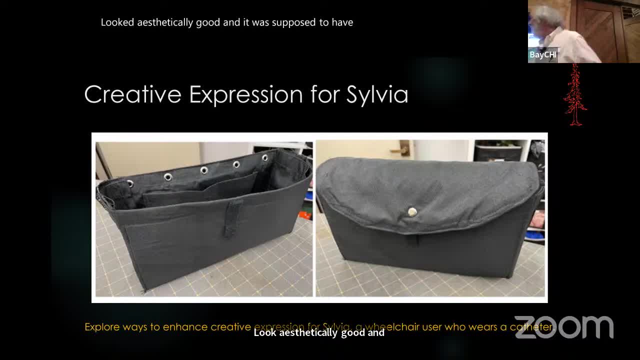 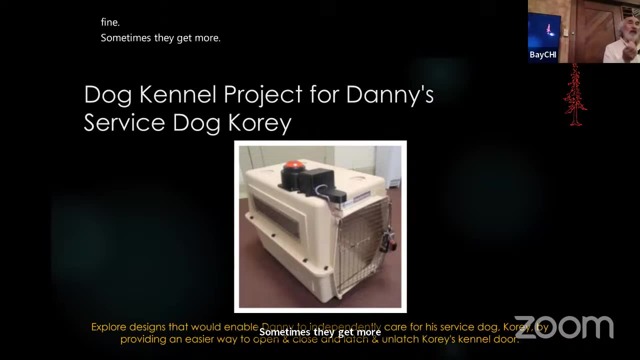 And it was supposed to have artistic expression on it And that didn't happen really well And the students had a tough job sewing it, but it worked out fine. Sometimes they get more benefit from working with the person than actually coming up with their device. 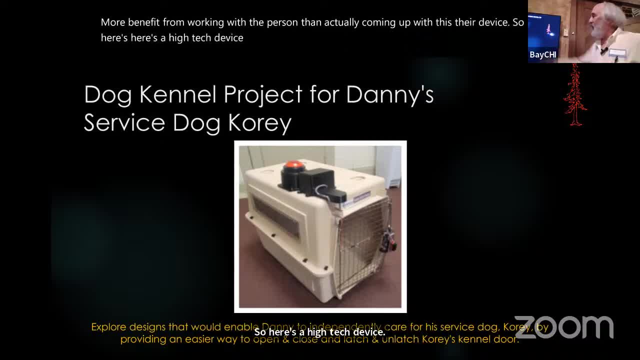 So here's a high-tech device. So this is for Danny, who has a service dog, And Danny is a person who's a wheelchair user. He has limited, He has vision and grasp and has cerebral palsy, And the service dog sleeps in this kennel at night but he has a problem, you know, unlatching the door and opening it up so it doesn't interfere with his wheelchair. 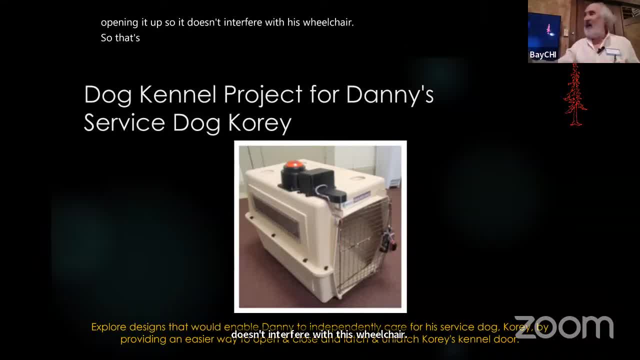 So that's a challenge that I identified, And so the students came up with a device that they hit this button. There's a computer in here that unlatches, that has a servo motor that unlatches the latch And a stepper motor that opens the door, and it just works perfectly. 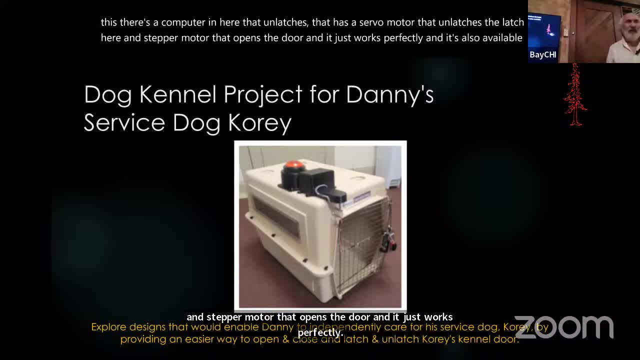 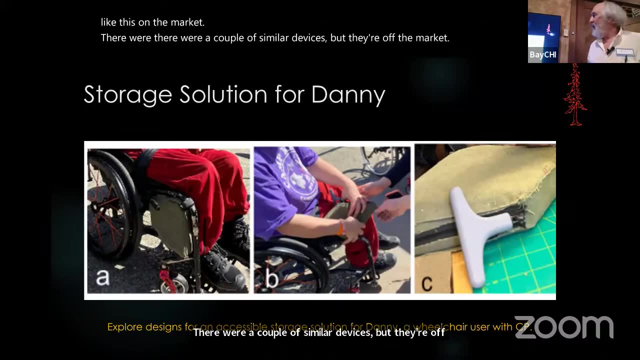 And it's also available through Alexa so we can command it by voice to open. So I mean there's no device like this on the market. There were a couple of similar devices, but they're off the market. And here's another solution for Danny. 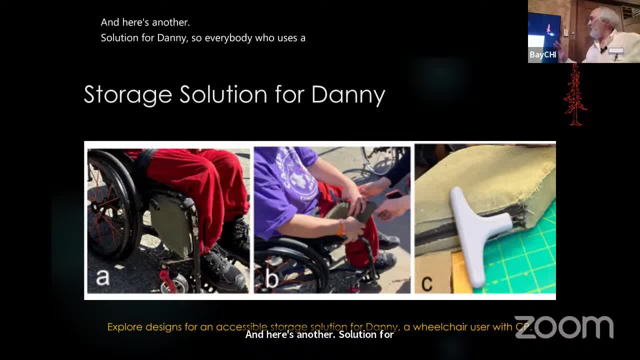 So everybody who uses a wheelchair has problems with storage. You know where to put things, And so this team worked on a bag that fits on the side of the wheelchair, that's easily accessible, And since Danny has a problem, you know, grabbing a zipper, they use this adaptive opening device so he can easily work it. 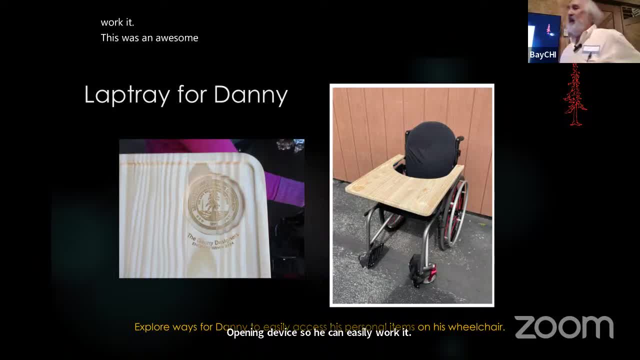 This was an awesome lap tray that students made. Every person who uses a wheelchair needs to have a surface, you know, to put their stuff on, Whether it's a laptop or, you know, food or laundry in this case- And this turned out to be really good. 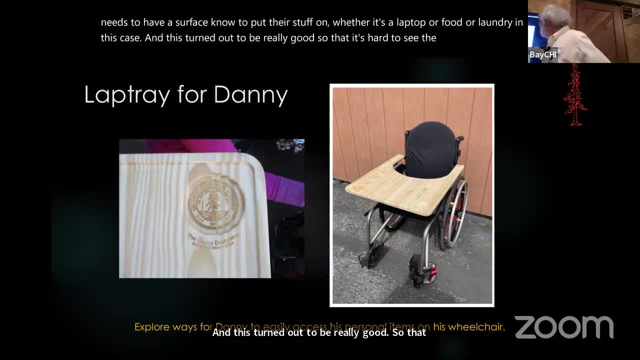 So it's hard to see the details. but this lap tray splits in the middle and it sort of folds in on itself And so it opens. it's able to be removed once you fold it up And once you put it in it has clamps along the side that clamp against the armrests. 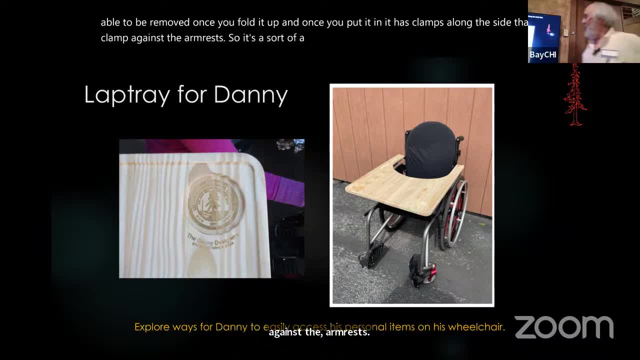 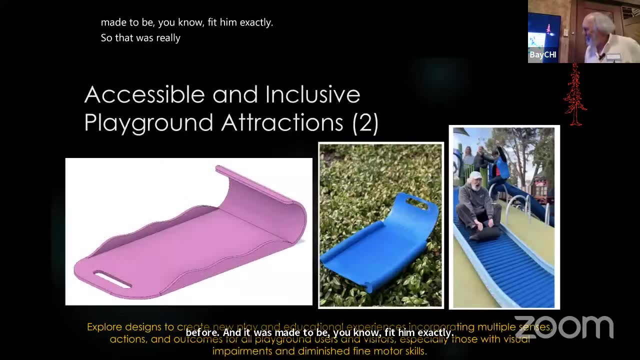 So it's sort of a new design that I've never seen before And it was made to be, you know, fit him exactly, So that was really good. So this is the other project for the Magical Bridge Playground, And the students went there and they saw the playground littered with cardboard. 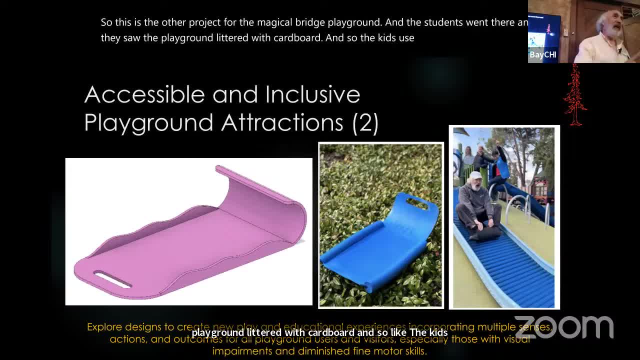 And so the kids use cardboard to go down the slide faster or down the hill that the slide is on. And so they did that from day one. And so the students said, oh, there's got to be a better way of doing this. 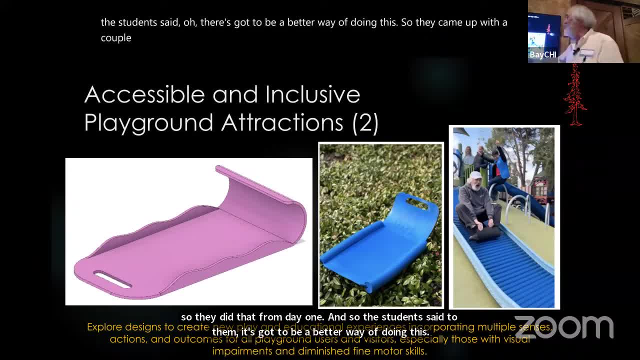 So they came up with a couple of designs for the sleds. And here's me on there And I'm telling you: you know, going down the slide when you're older is very scary, as you can see, as you can see here. 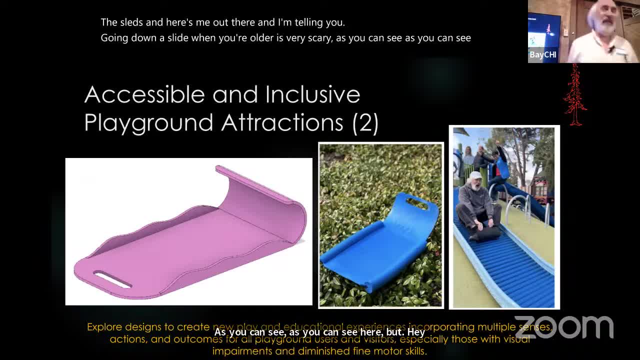 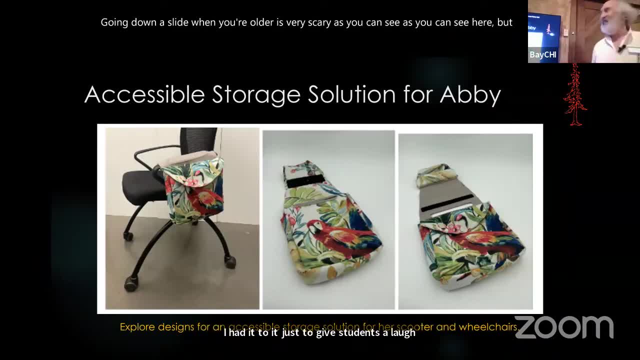 But that's it, And you know, I had to do it just to give students a laugh. Sorry, The slide sled, Slide sled- OK, that's a good name for it. So a storage solution for Abby, who's a wheelchair user. 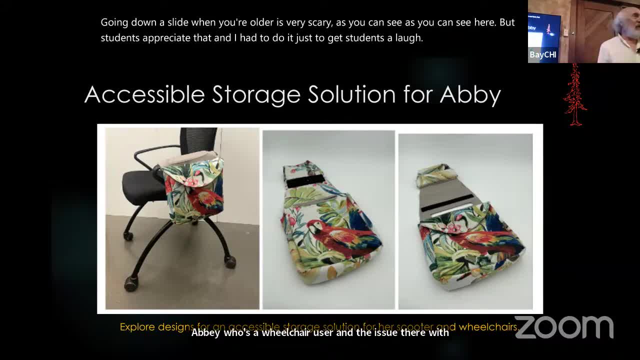 And the issue there with her is that she has multiple wheelchairs, And so to make a storage system that only fits on one, you know, wouldn't, you know, it wouldn't be good. So they came up with a design with two pieces. 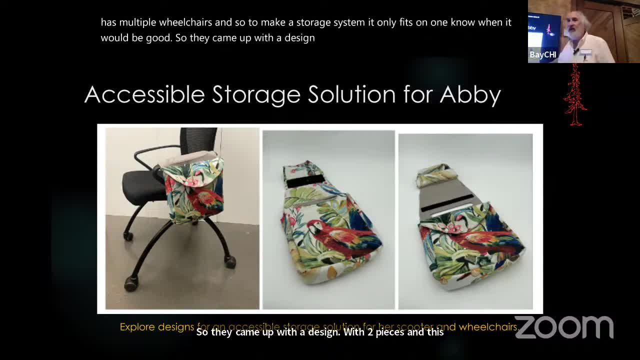 And this piece folds into the slot here on the other side And that is around the armrest. So that works for three wheelchairs and two scooters. So that was a good design, And they picked out some very colorful material and sewed it up. 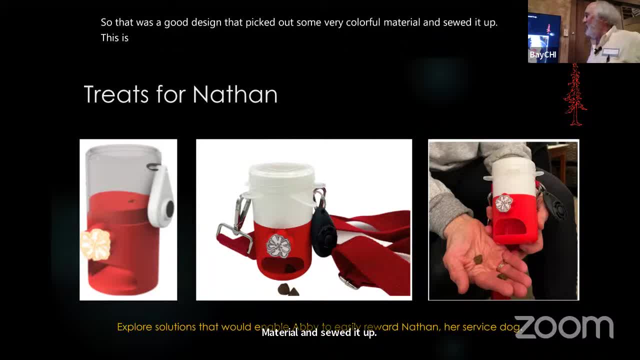 This is for Abby's service dog, Nathan, And anybody that has a dog that they train knows that when the dog does something good, you're supposed to give them a treat immediately. Well, for Abby, she has the treats in her backpack on the back of the wheelchair. 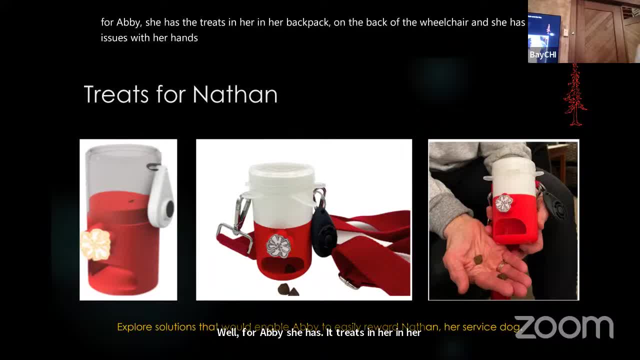 And she has issues with her hands And it takes a while for her To get the treats out and provide it. So the students 3D printed this device And all she has to do is rotate this knob and treats will come out. 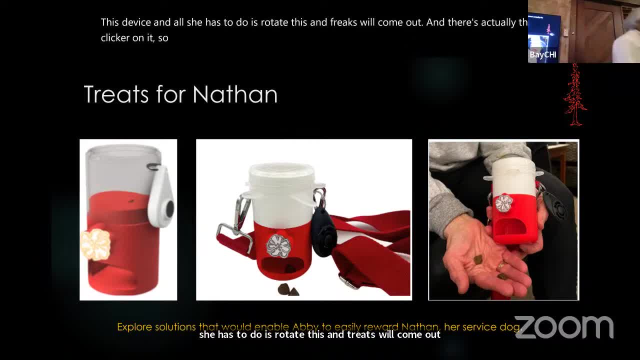 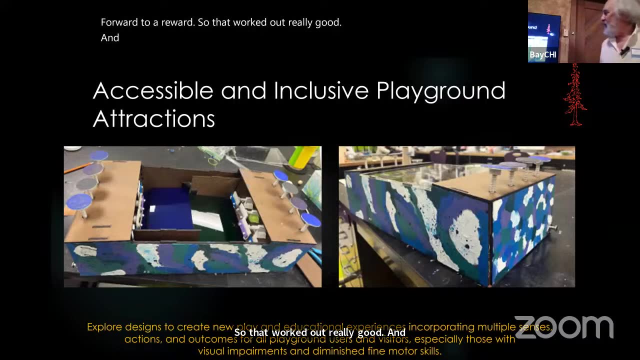 And there's actually the clicker on it. So the clicker indicates to the dog that to expect a reward. So they start salivating and looking forward to a reward. So that worked out really good. And from last year Students made this sort of pinball machine for the playground. 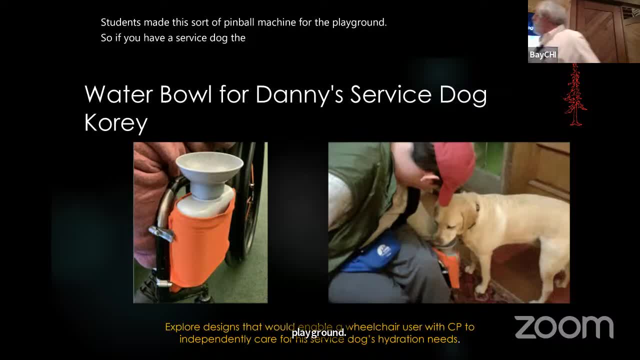 So if you have a service dog, the dog needs to be fed and hydrated. So this year we worked on the design for this system. So this is a reservoir And when Danny presses the reservoir, water comes up into the bowl And the dog on the first day knew that that was water for him to drink. 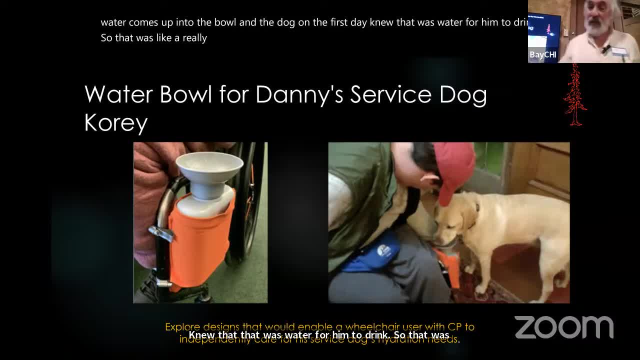 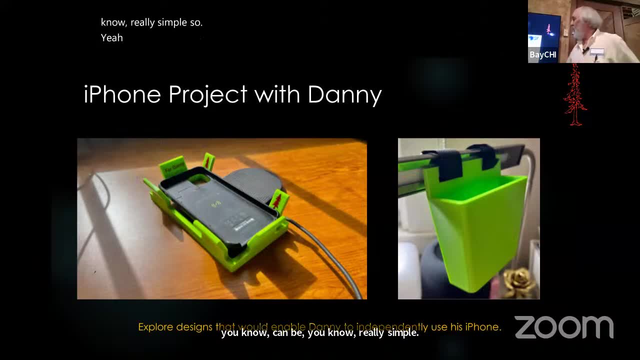 So that was like a really easy solution. A lot of these solutions You know can be, you know, really simple. So, yeah, And they also came up with a holder for him So that you know he has a hard time seeing and placing things. 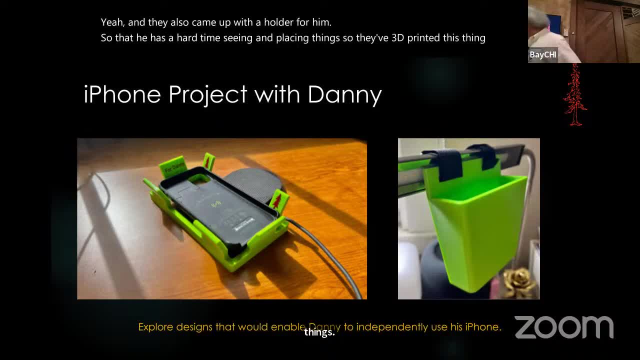 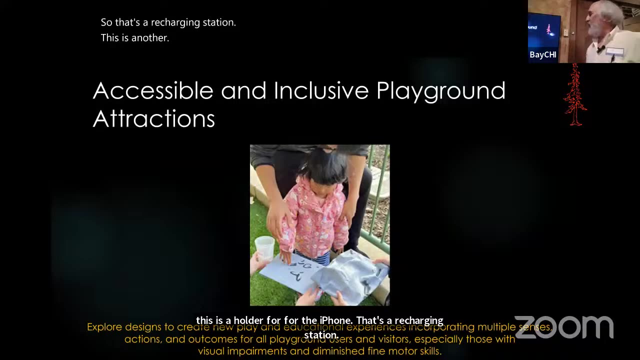 So they 3D printed this thing that would ease the iPhone into the cradle, And this is a holder for the iPhone. That's a recharging station. This is another playground And the students are using this clay material that, when wet, it produces a dark image. 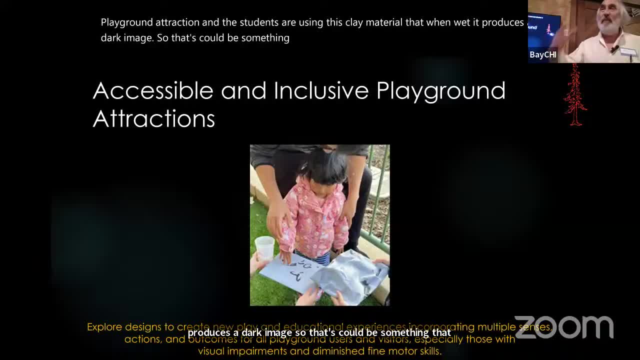 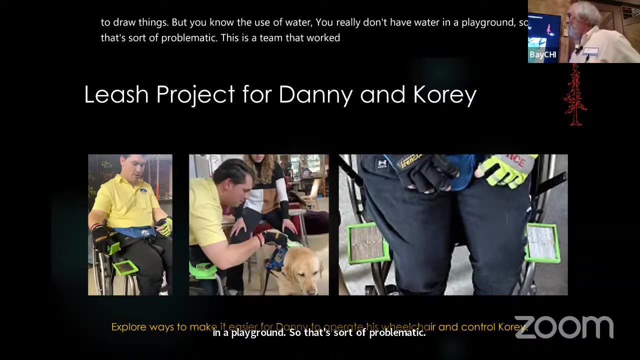 So that could be something that students can use repetitively in the playground to draw things. But you know the use of water. you really don't have water in a playground, So that's sort of problematic. This is a team that worked on a dog leash system for Corvina. 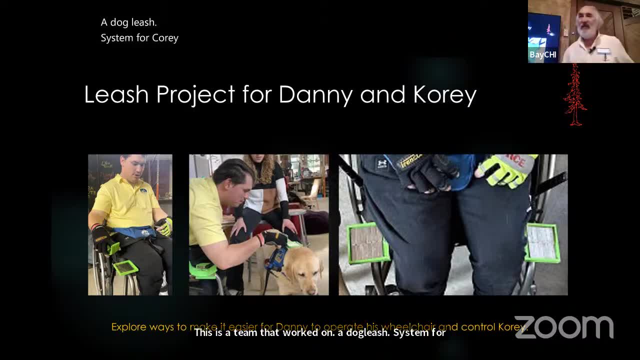 This is a team that worked on a dog leash system for Corvina. Danny again, has really trouble with his hands. He can't operate the buckle, And so the students came up with a magnetic attachment. So there's a bunch of magnets in here and on the leash and on the dog. 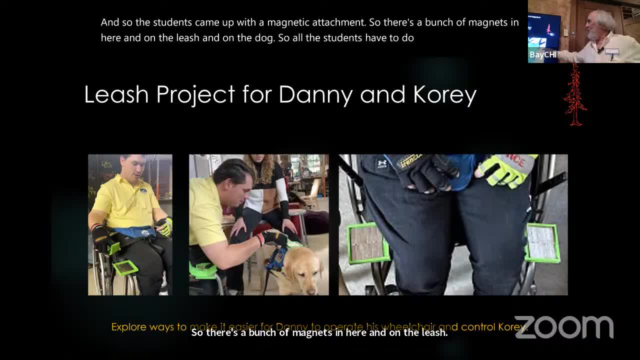 So all the students have to do is all Danny has to do is put the leash onto this and it attaches, And by sort of twisting it, it unattaches. So and that was done, And by a team of students with no engineering background at all, but they were able to do it. 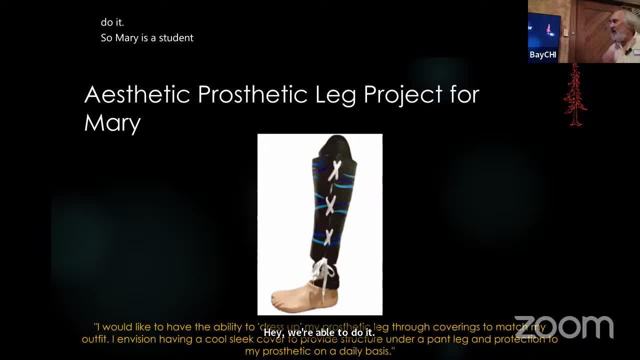 So Mary is a student who has a prosthetic leg And I always thought it would be a neat idea to, you know, dress up that prosthetic leg. I wanted to have the students work on something that, would, you know, light up as she walked or as she danced, or to the music and stuff. 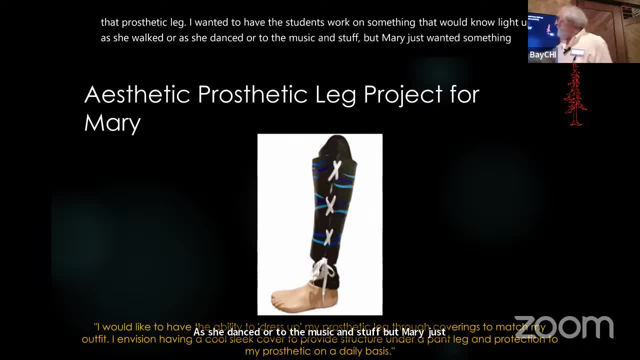 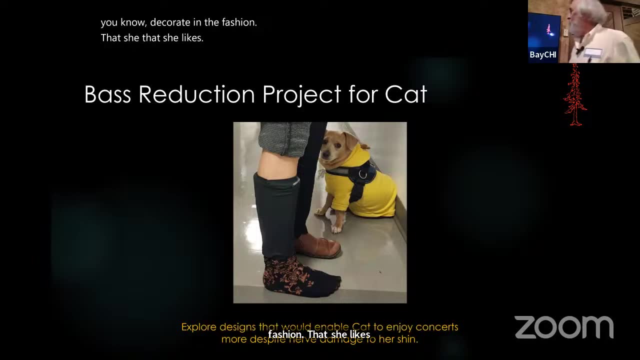 But Mary just wanted something that you know looks a little bit different. So here's something that is easy, Laced onto her prosthetic leg, that she can, you know, decorate it in a fashion that she, that she likes. So this is. this is the lower leg of Kat and her dog. 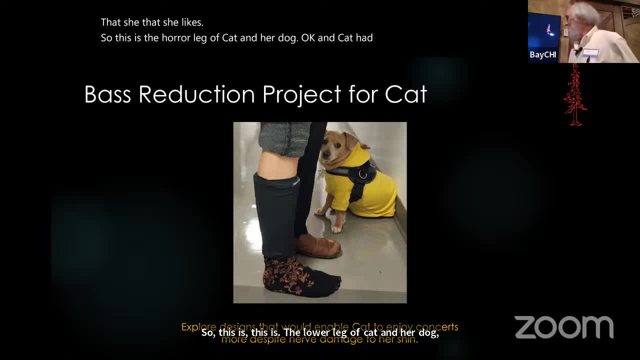 Okay, And Kat had this issue with nerve damage in her shin and she liked to go to concerts but the music caused pain. So the students were given the task, you know, find something that would attach And then you wake the sound so she wouldn't have pain. 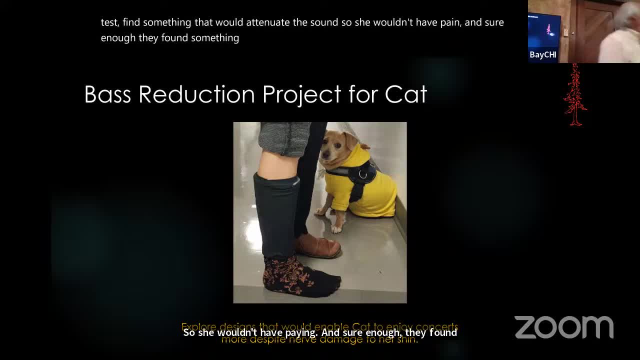 And sure enough, they found something, and it turned out to be acoustic insulator made for for cars where you have the big, you know boom box speakers in it. So they bought this thing, you know, for $15 and made it into a sleeve and it worked great. 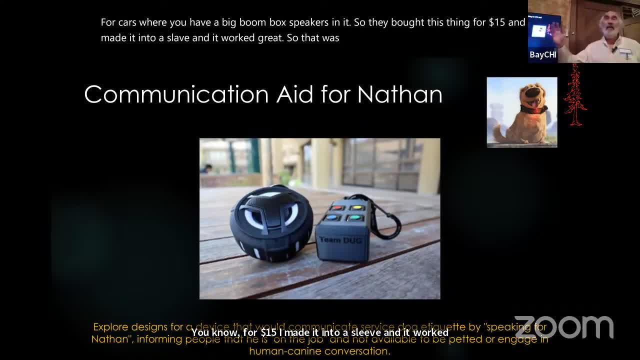 So that was, that was neat. Okay, Who remembers this? this, this dog? Okay, Okay, It's from up. And what was the dog's name? Doug, Doug, Right, So remember the collar that Doug wore. What did, what did? what did it do? 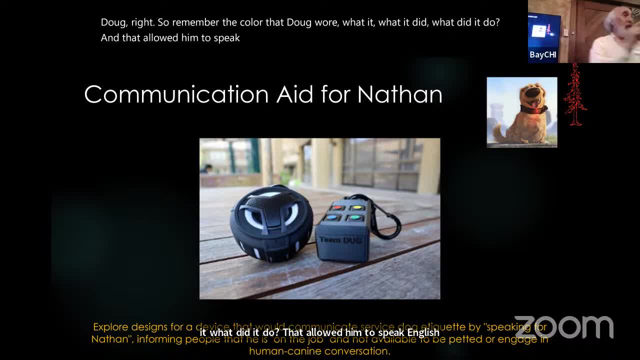 It allowed him to speak English. Yeah, So it was a brain computer interface that allowed him to vocalize what he was thinking. So we did sort of the same thing in class, but now it's not a brain computer interface. So everybody that has a service dog has this problem where people see the dog. 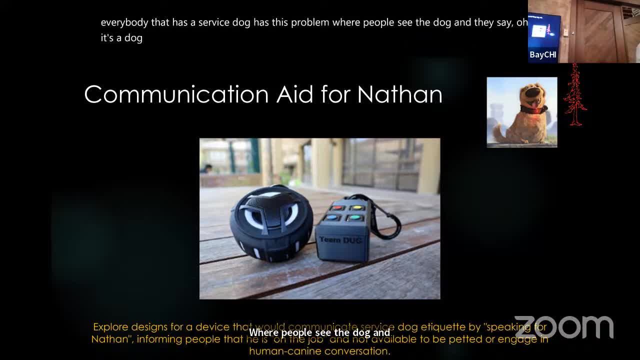 And I say, oh, it's a dog And it's. this is something I I need to get my dog fix. I need to go up to the person and say, oh, what a cute dog. You know what's his name. 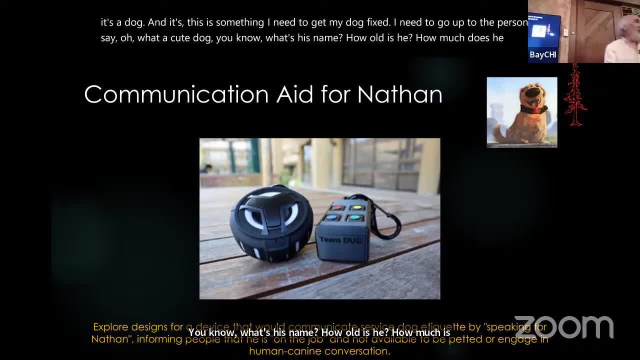 How old is he, How much does he weigh? And of course the dog- a service dog- is working, And so you're disrupting the service dogs. you know work ethic, So you know what the owner has to do is say: don't disturb the dog. 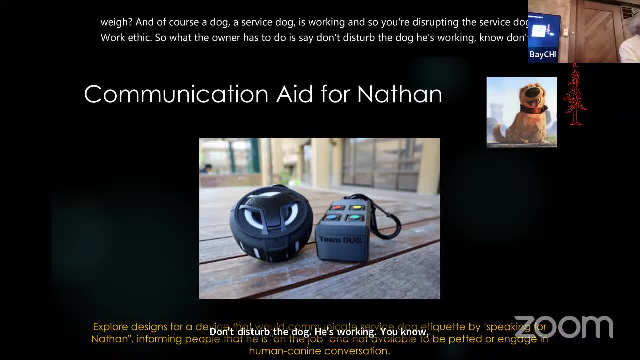 He's working, you know, don't distract him. And every time You know she's out, you know there's. you'd say it again, and, again, and again. So what this thing does? this is just a Bluetooth speaker. 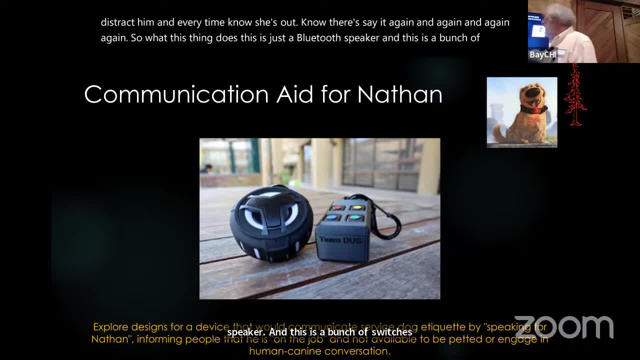 And this is a bunch of switches with a Bluetooth interface And when it does, when you press the button, it sends an MP3 over Bluetooth And so you can have the dog say anything you want. You can say it in the owner's voice or a presumed dog's voice, and stuff. 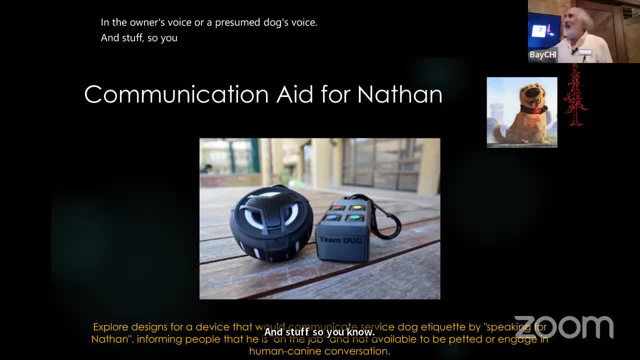 So you know, uh. so It's actually. uh was awarded second place in the student design competition this past year, So that was really yeah. But you know, I mean you have to identify these problems. So here's Abby again. 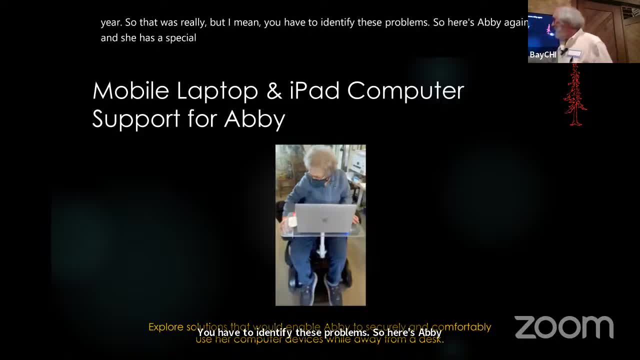 And uh, she has a special wheelchair And uh, you want it. she wanted a, a place to put her laptop, because she goes out for coffee and wants to work on her Macintosh computer and have the mouse there and have it um. 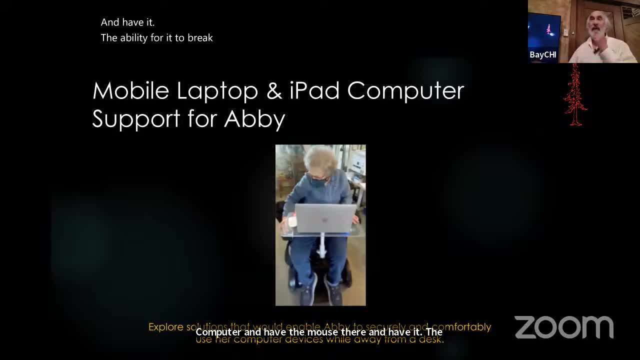 the ability for it to uh to work And uh, she had to have a breakdown so she can put it in the in the in her backpack. So those were the design criteria. So the students came up with this, this really nice piece of acrylic and some PVC piping that fits um. 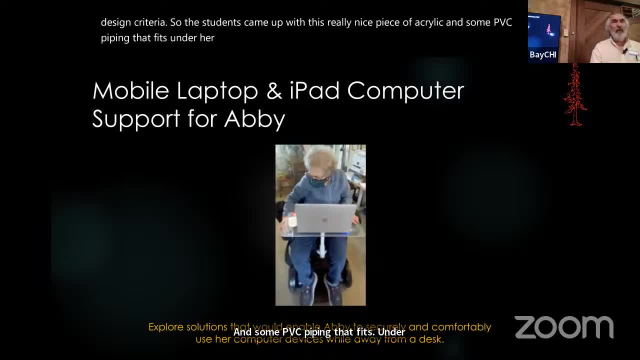 under her her cushion, um on her wheelchair, And so it's it's very easy to use And, uh, these guys that were on this team were all athletes and that's what they came up with. Um, so that was. that was really neat. 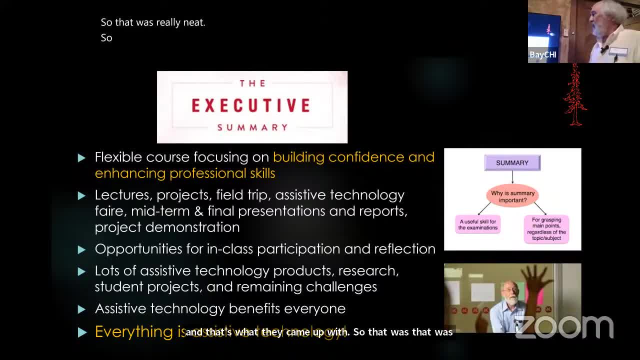 So, um, In summary, the course is one that focuses on building confidence, enhancing professional skills. You know, we go on a field trip to the Magical Bridge Playground, We have the lectures, we have the projects, I have an assistive technology fair where I bring in uh companies and services related to disability and assistive technology. 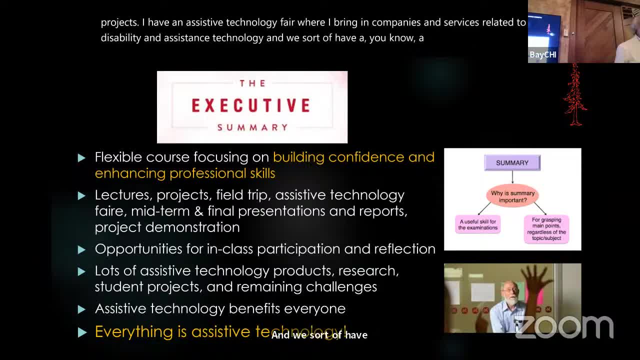 And we sort of have a, you know, a trade show atmosphere. And, um, this was actually one thing that worked really good over Zoom on COVID, Because I put each vendor in a different breakout room and the students just went from one breakout room to another. 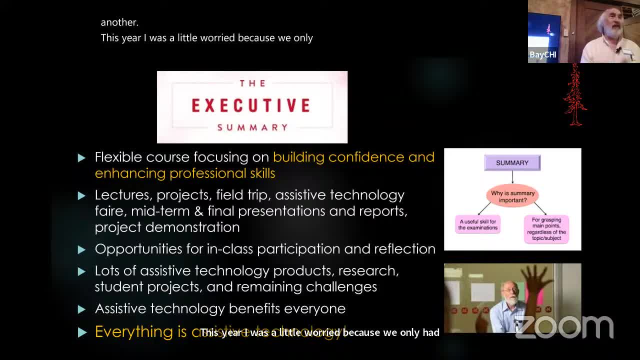 Uh, this year I was a little worried because we only had like five vendors, but that gave students a lot more time to spend at each table And it worked out really really well. Um, okay, Um, the students also reflect on their experience. 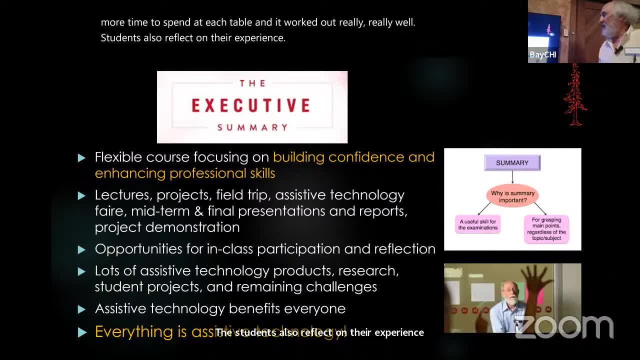 Um, And so you know again: assistive technology benefits everybody, Everybody benefits. We use assistive technology every every day. Does that mean we're disabled? Well, I mean we're not. you know, a super, a superhero like Superman would say: you know you, you guys can't even fly. you know you're you're deaf, disabled, you can't even fly. 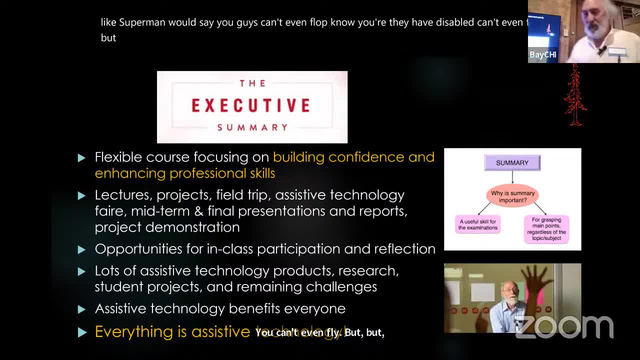 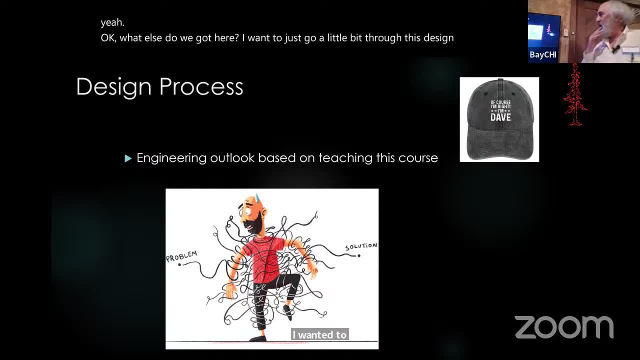 But, um, but, um, yeah, Okay, What else do we got here? Uh, I want to just go a little bit through this design process, Uh, that we use in the class And uh, you know. so these are slides that I use. 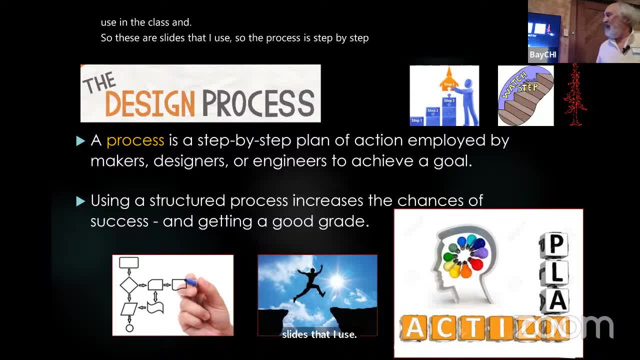 So the process is a step by step plan, plan of action, um employed by the students to achieve their goal and and and using it as a structured way increases the chances of success. And and, of course, student respond to respond to getting good grades. 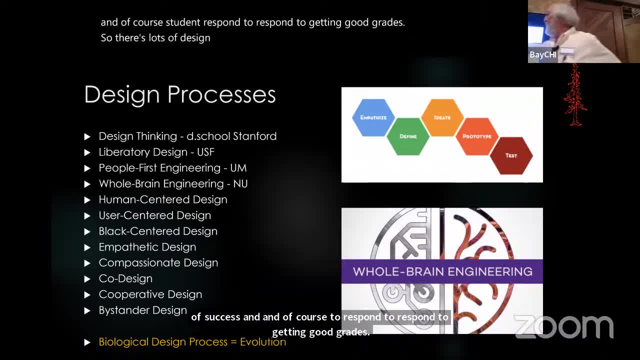 So there's lots of design processes and at Stanford the D school has um design thinking that has all these hexagons which, um you know, they promote as being um, uh, uh, a general, um design process that you can, that anybody can use in any context, but that it doesn't work in my class. 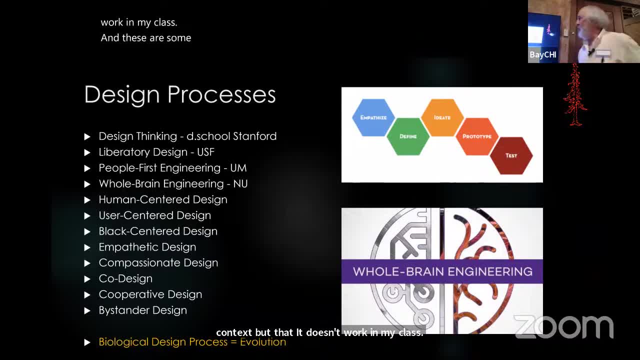 Um, and these are some other named um processes and it's at Northwestern They, their process is called whole brain engineering. So I mean that's different. So you know there's lots of activities in the design process. 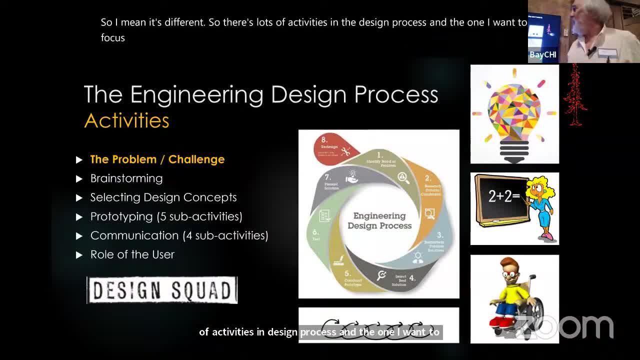 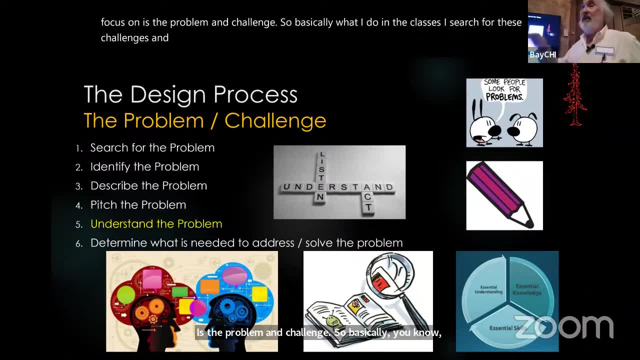 And the one I want to focus on is is the problem and challenge. So, basically, you know, what I do in the class is I search for these challenges and problems, I identify them, I describe them, I make up a description that's on the website, um and um, um, that the students can review before, um, uh, before the problems are pitched to the class on the second day of class. 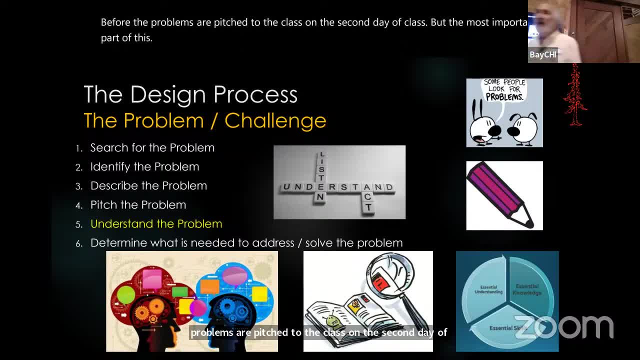 Okay, Um, but the most important part of this, which I haven't seen enunciated in any of these design process, is to understand the problem. Okay, I mean, it's just super obvious to me: The more you understand about the problem, the better the solution you'll come up with, and all these other design processes. I've never seen this mentioned. 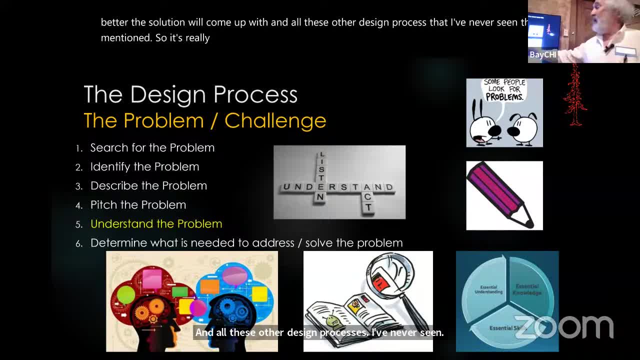 So it's it's really important. So you need to understand the problem, to determine what is needed. So you need to have this knowledge That you can use to brainstorm ideas that would solve that. I mean, to me that's, it's just so obvious. 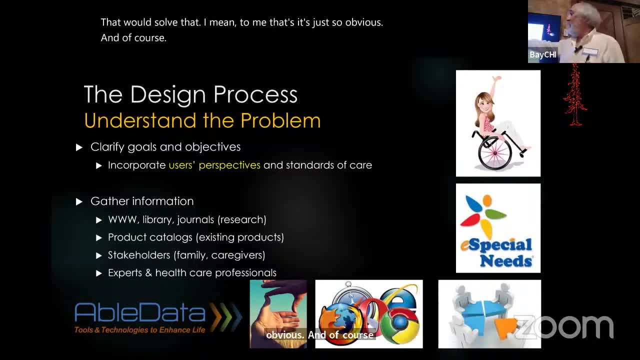 And of course, you need to understand, incorporate what the user, uh, says. And so you, the students, have to go in and interview the user, observe them, observe the, the challenge, um, you know, talk to them and see, you know, they even go to the, the um, um, the community partners. 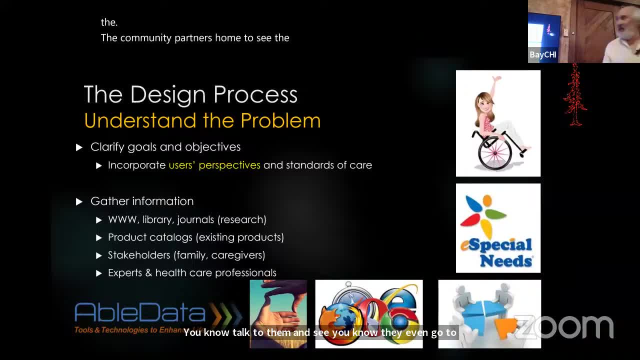 You know home To see the challenge in context. Okay, And of course you know, I encourage students to go on the internet see what else is available. Talk to experts In terms of uh- observing what? what do you think the trade-offs are in being the uh, the user? 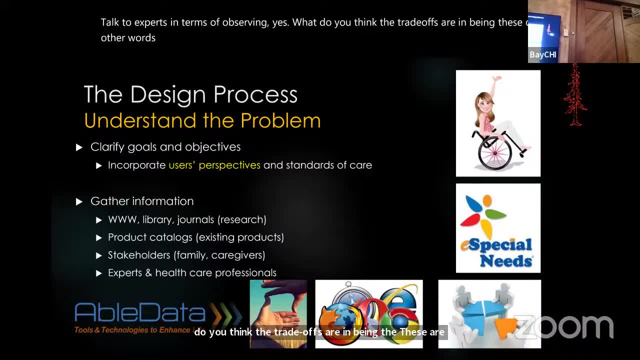 In other words, uh, being not, not, not, not, not interviewing them, not observing them as an anthropologist, but actually, uh, modeling them, being, you know, acting, you know, taking on their No, um, uh, we don't use personas in the class because personas are imaginary people and I want to make sure that they talk to a real person that has a real challenge that can be enunciated and observed, you know, through through observation and interviewed to get a sense of of the person and what their goals are, and things like that. 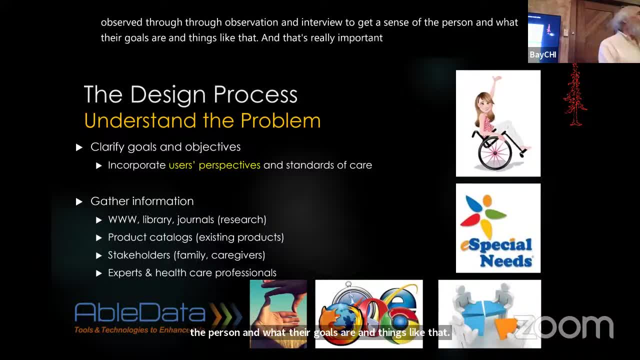 And that's that's really important, because, I mean, that's the customer And in my course, you know it's the only customer. they only work to solve the problem of that one person, because, even though there's lots of people with the disability to say, build something that will help, you know 10,000 people with this disability, how are you going to, you know, get background from 10,000 people? 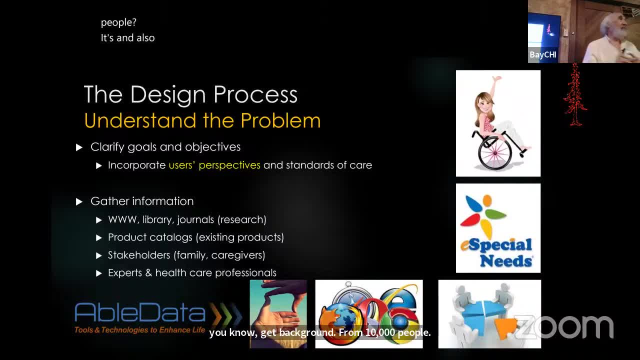 It's, and you know, also considering that everybody with a disability is pretty much an individual. So to make things simple for the student, um, you know, we would work with that one individual and I don't care about the commercialization part of it, because I couldn't fit that into a 10 week course to begin with. 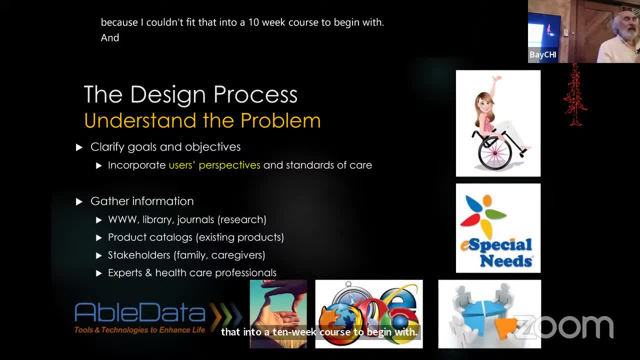 And, um, you know, making something, making a commercial product, product is something that may take years and millions of dollars And I don't have the kind of funding And I don't have the kind of funding for the class and most of the time it's not going to be successful. 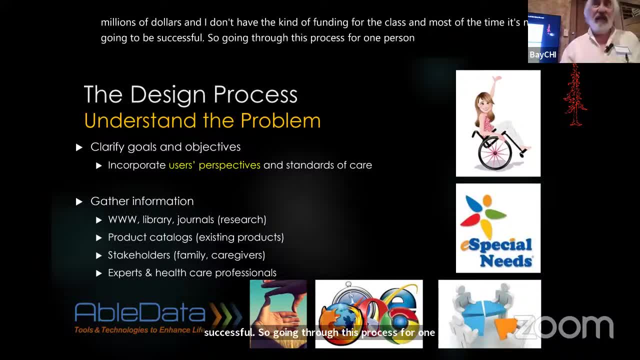 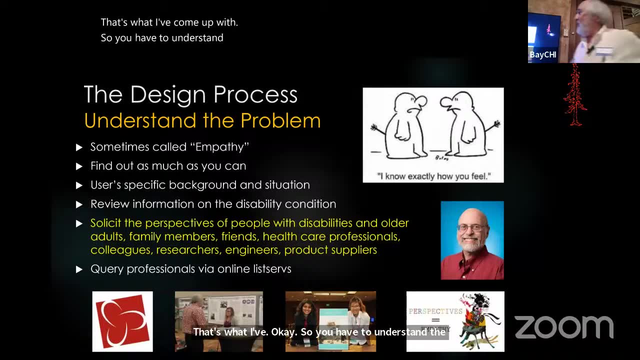 So going through this process for one person is sufficient for the class. That's what I've come up with. So you have to understand the, the, the, the person. I don't like the term empathy, because empathy is like this: knowing exactly how somebody feels. but what we want is to to um, include the desire to um, um address the problem. 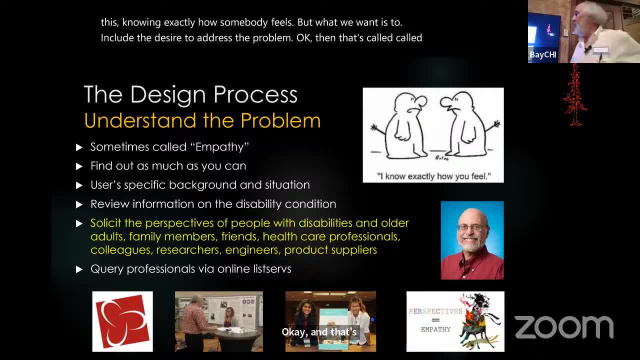 Okay, And then, And that's called called compassion. So you, the students, have to find out as much as you can about the user's background, about the disability condition And um, so we'll sit. you know, information from family members, other healthcare professionals, um and and um, um, you know, talk to other people. 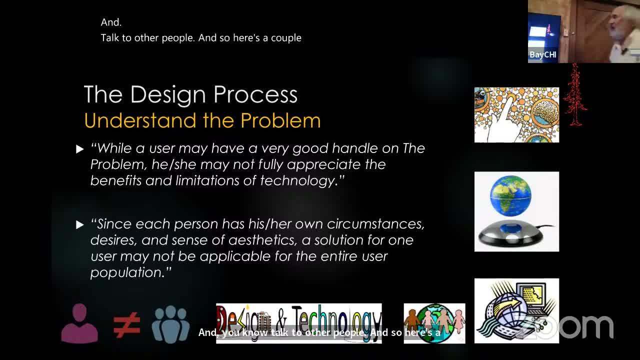 And so here's a couple of slogans I've come up with, um to describe this process. The user will have a very good Handle on what the problem is and what their challenges are, but he or she may not be a designer and engineer, so they not may not fully appreciate the benefits of limitations of technology. 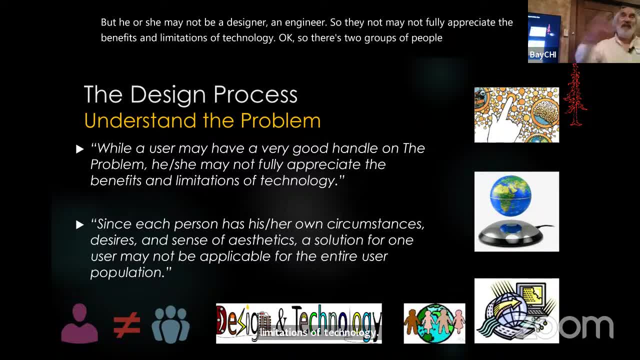 Okay, So there's two groups of people here: There's the students and then there's the user and then there's me. Okay, So everybody has a little bit different role in there. So, Since each person has their own Circumstances, desires, sense of aesthetics, 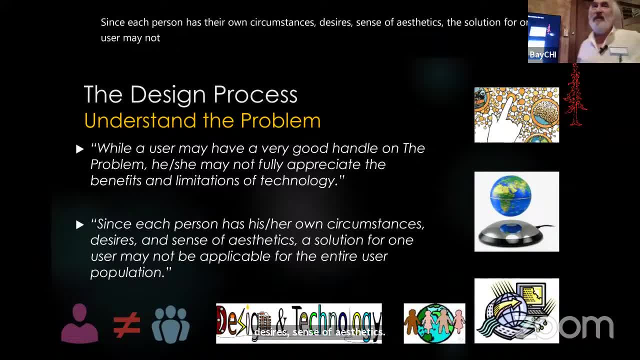 The solution for one User may not be applicable for the entire population. Now there's a slogan in assistive technology that says solve for one and extend to many, But I don't think that works in with people with disability because of these differences in, in, in in each individual. 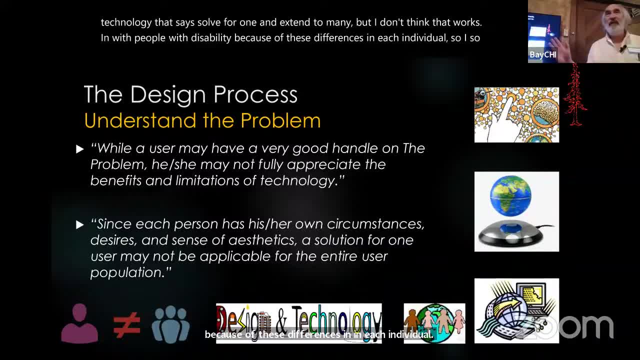 So I so again, I'm not interested in commercialization at all. Ask another question. Yes, You, you brought up that topic, That it's you designed for one person several times. Yeah, That is kind of in contrast, you might say, to the whole idea of universal design, which. 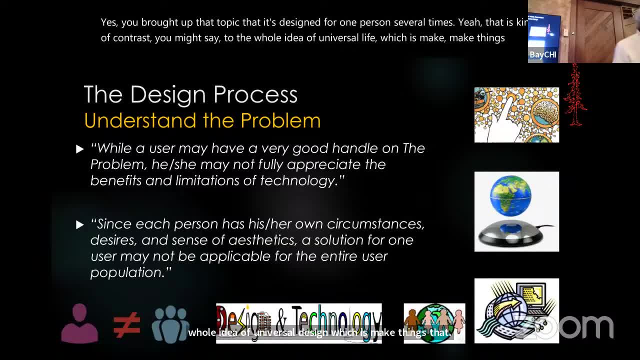 is make, make things that work for every, for disability, and will help everybody. And I can think of many examples of that. I've even made many examples of that And you're not focusing on that because you just don't believe in it or because you think. 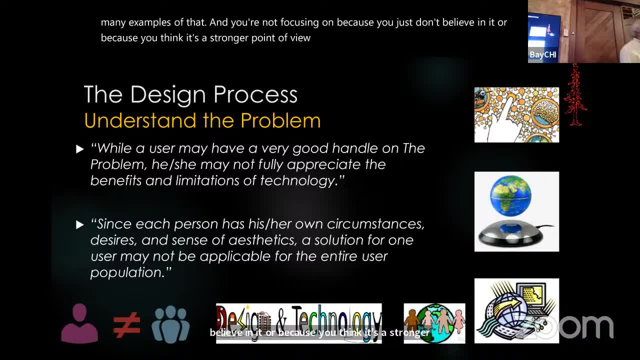 it's a stronger point of view and more helpful to your designers. Well, The issue here is: universal design is a very important concept, but it's things that best work when there's a shared resource, when there's a building that needs to be accessible. 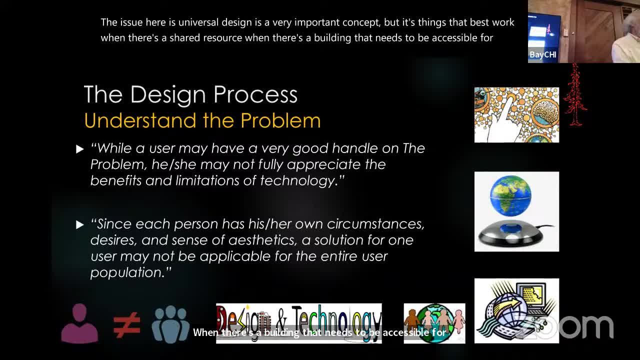 for everyone, where the internet has to be accessible, because a lot of people with disabilities use it. But when you talk about a device for an individual, something that it's, it's, it's different, Universal design isn't? it's not required. 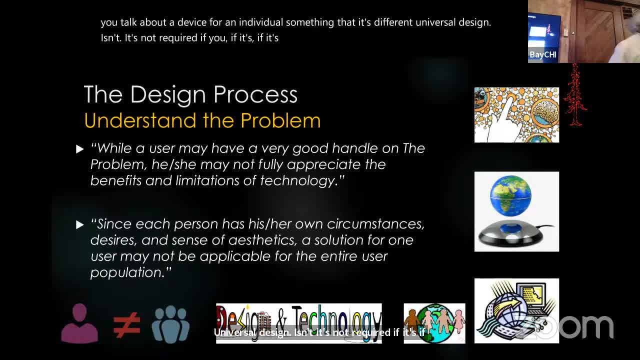 If you're, if it's, if it's something that just that one person uses, Okay, Does that answer your problem or not? I don't want to belabor it. I just want to say that a lot, of, a lot of people use. well, when Apple made a bunch. 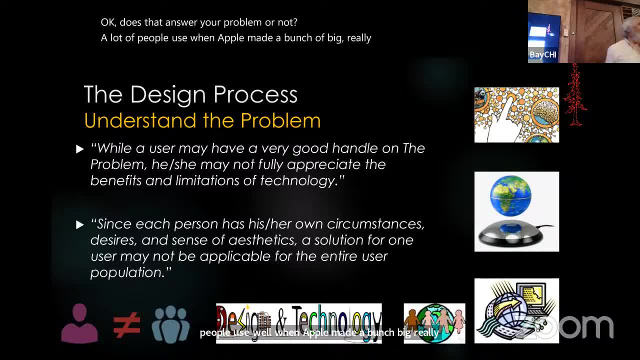 of big, really serious effort in the disability package. And I went to the, you know, American Federation for the Blind, Yeah, And they had this huge room Full of assistive devices And they said all of these are worse than this iPhone now. 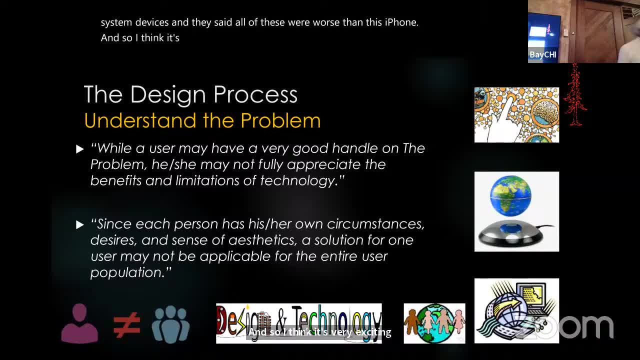 And so I think it's very exciting when people make something that's a tool that many, many people can use, And I think it's possible And so that's. you know, that doesn't mean that your your your point that working for. 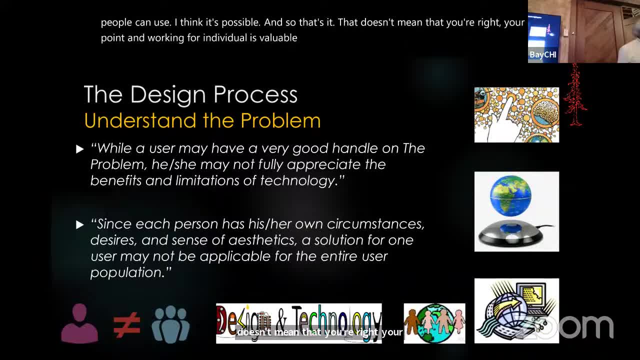 an individual isn't valuable. I just can think of places where universal design has been helpful. Yeah, For a product. you want that because that one product is going to be a shared product for lots of people. But a lot of times It doesn't work that way that a an individual may, that may not help a specific individual. 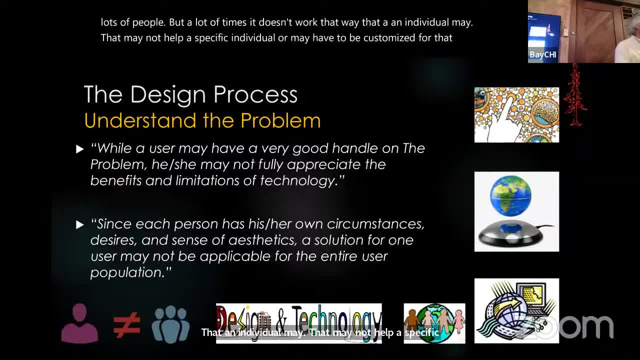 or may have to be customized for that individual. So just to blow my own horn, the track point is useful in many, many different ways for people with disabilities that I hadn't anticipated Right, And you know I could go into that in detail. 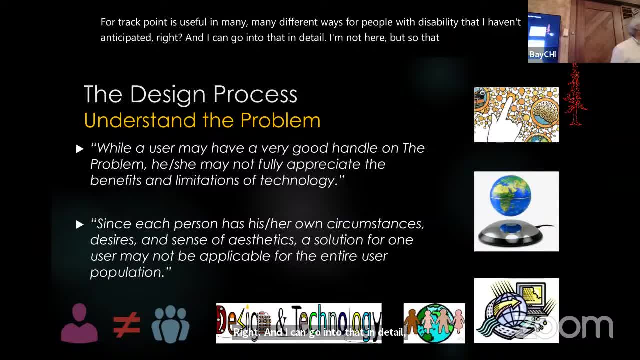 I'm not here, but so that that's kind of exciting when you make something that that actually can can, is flexible enough And powerful enough in its own ways that it gets used by many people. Right, Okay, I I'll, I'll agree with that. 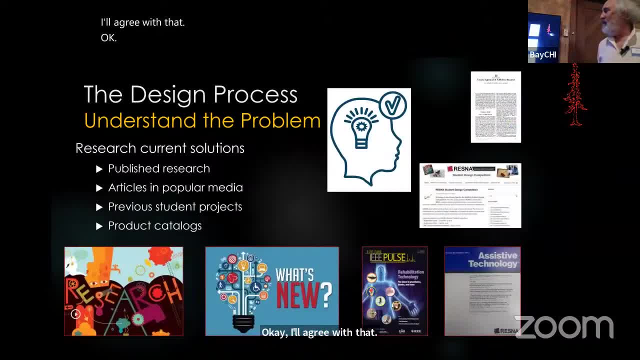 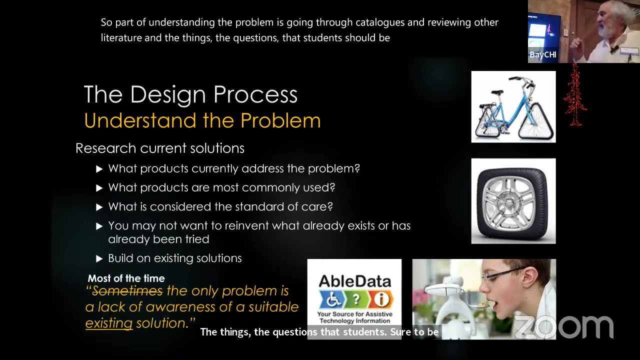 Okay, Oh, so part of understanding the problem is going through catalogs and reviewing other literature and the things. the questions that students should be asking is: are there products on the market already That sort of address this problem And, if there are, you know what are the most commonly used? which one are commonly used? 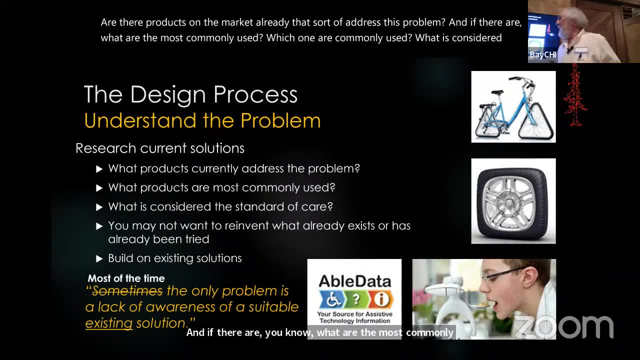 What is considered standard. You know and and sometimes is you know, why aren't the products that are on the market solutions? Why do people still need something? So those are all questions to ask. So you build on the, on existing solutions, but- and this is my top level slogan- 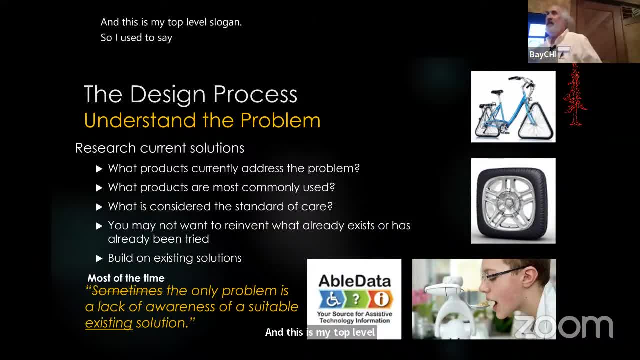 So I used to say sometimes the only problem is a lack of awareness of a suitable existing solution, But now I say most of the time. So if you're a person with a disability, you may. you probably don't know what's out there. 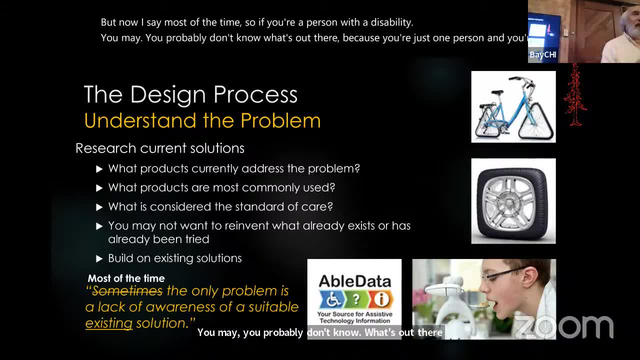 because you're just one person and you're not on the internet. but you know, occupational therapist or a rehab engineer might have a broader view And when, when somebody approaches me with a challenge, the first thing I'll do is I'll go online. 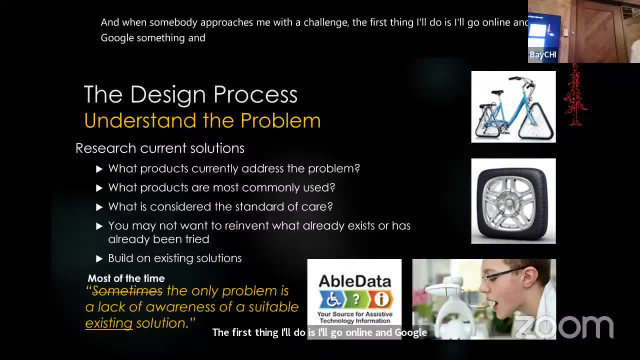 and Google something And most of the time I get pages and pages of possible solutions And to me it's it's it's terrible to copy something that's already available. It's a waste- waste of time and money. So I I always make sure that these challenges are heavy. 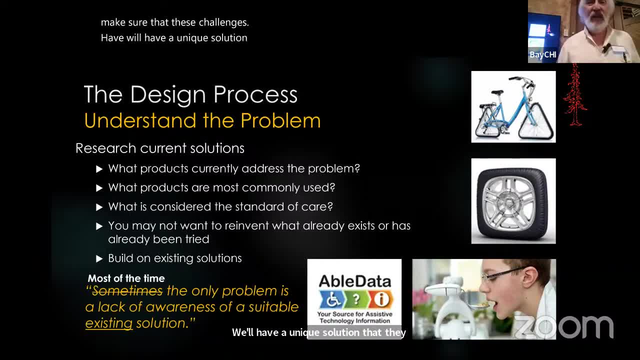 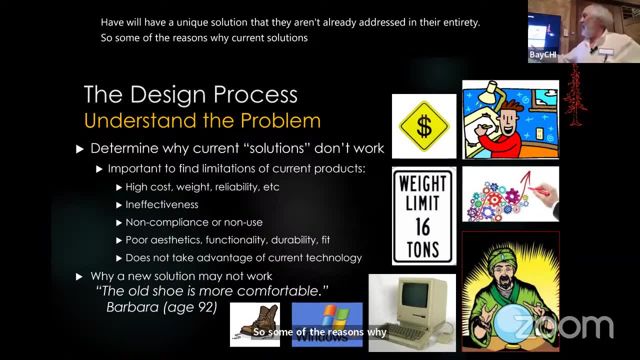 will have a unique solution that they aren't already addressed in their entirety. So some of the reasons why current solutions don't work: they may cost a lot of money, they may weigh a lot, they may be unreliable, ineffective, the student that the users may not use them. 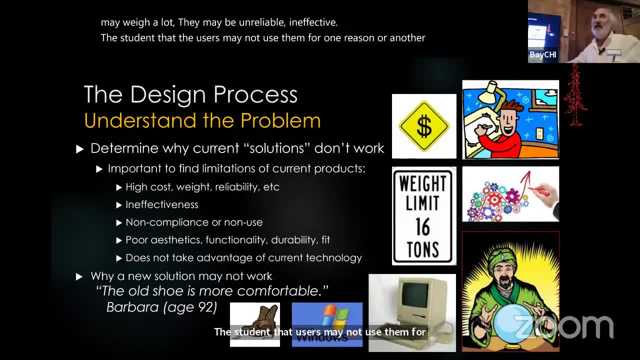 for one reason or another, because it may be a poor aesthetics or they don't function specifically for that individual. They again may not fit that individual or it may not take care of current technology. But I had a person who we made a custom-made walking stick for. 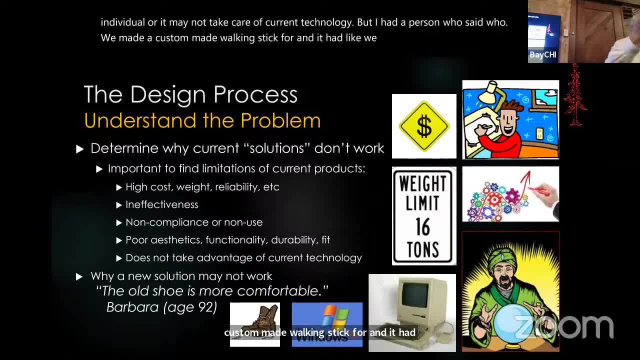 and we took a mold of her grip and they 3D-printed that and we got a custom cane and colored it and it's nice. And she said: you know, I have this cane that I made that has duct tape on it and I actually like that better. 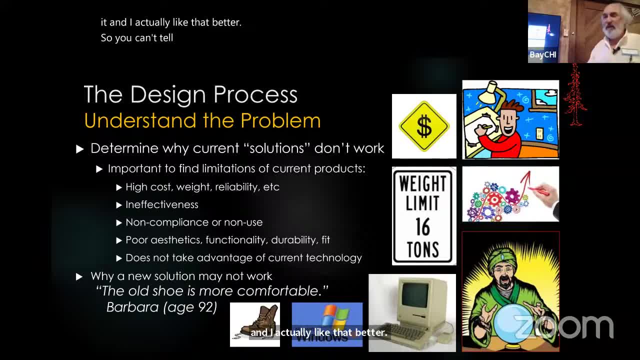 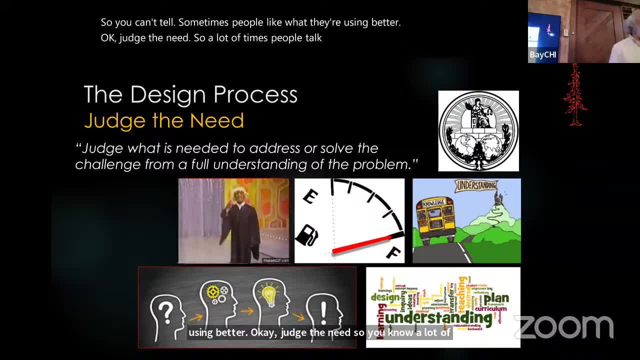 So you can't tell. Sometimes people like what they're using better. Okay, judge the need. So you know, a lot of times people talk about need-finding and to me that's not the right term because need is a judgment in my mind. okay, 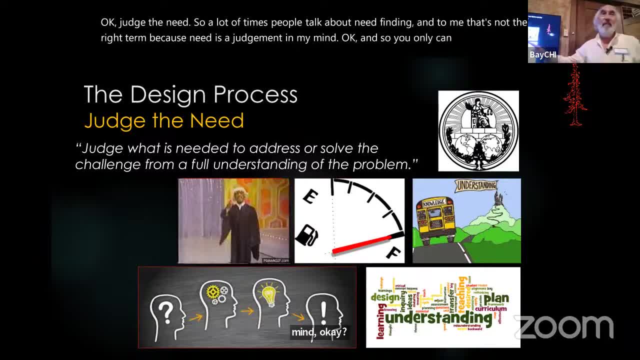 And so you only can judge what's needed by having knowledge of a full knowledge, by having knowledge of a full knowledge, by having knowledge of a full knowledge of the problem, a full understanding of the problem. okay, You can't start brainstorming. 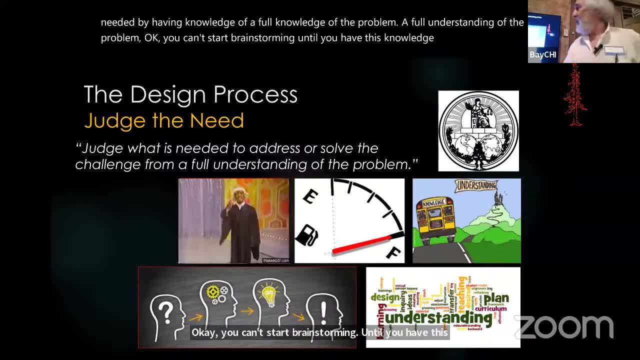 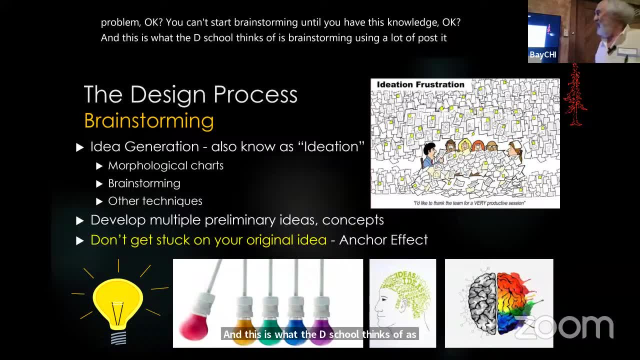 until you have this knowledge. okay, And this is what the dschool thinks of as brainstorming using a lot of Post-it notes. So there's all sorts of techniques for doing brainstorming. So the idea is to come up with lots of ideas. 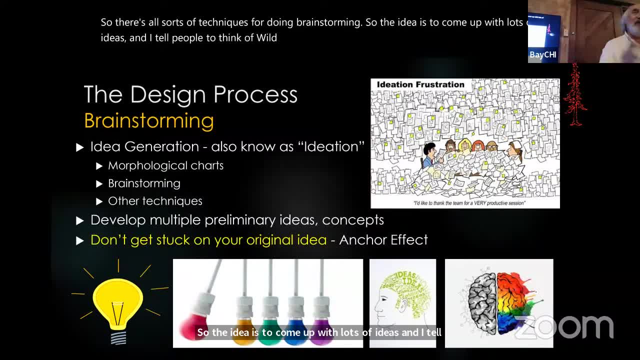 and I tell people to think of wild ideas and they're not done until they cross over to the the other side of the laws of physics and stuff like that and talk about you know really weird things, because at that point you know. 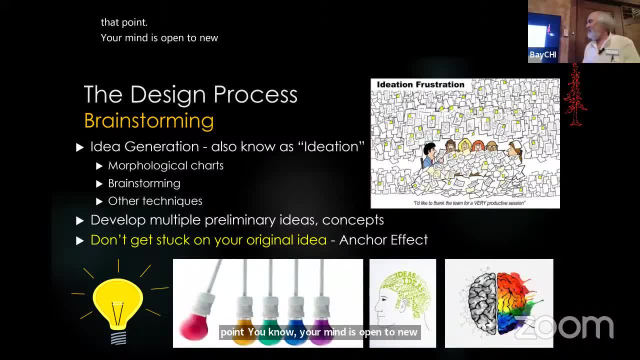 your mind is open to new kinds of ideas. Don't get stuck on the original idea. I had a student who all she wanted to do was brainstorm, So every new person she met was another opportunity for brainstorming, and she filled up like two sketchbooks. 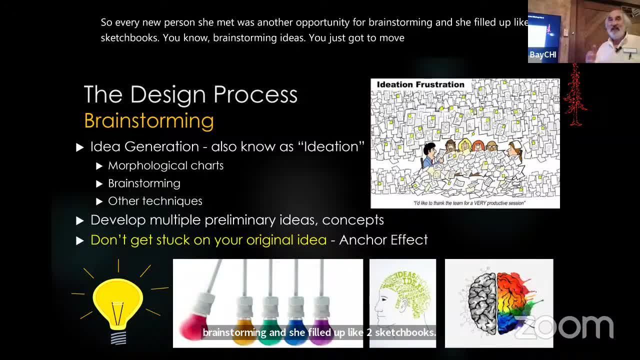 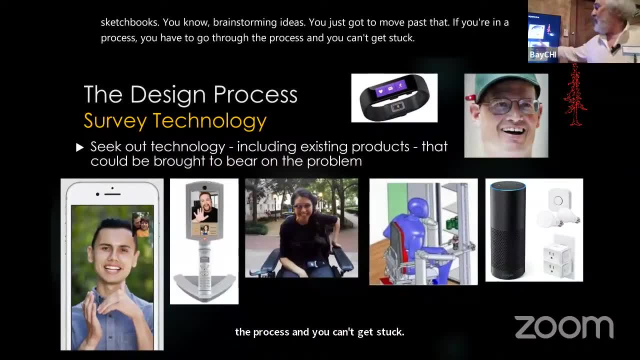 you know brainstorming ideas. You just gotta move past that. If you're in a process, you have to go through the process and you can't get stuck. And there may be technology out there that you can apply to your the current problem. 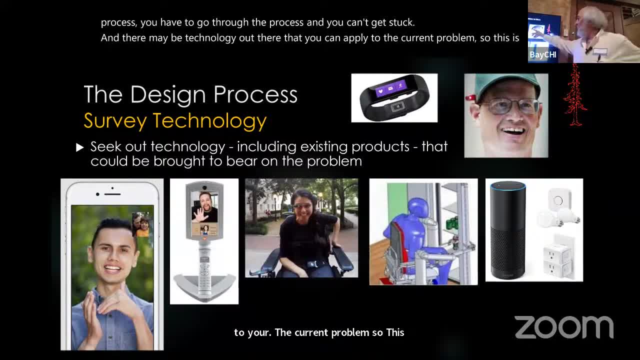 So this is Henry Evans, and he's using this laser pointer to point to an alphabet board because he's a non-vocal individual, And so that worked out really great. Other people you know use the Google Glass as a because they're a photographer with a disability. 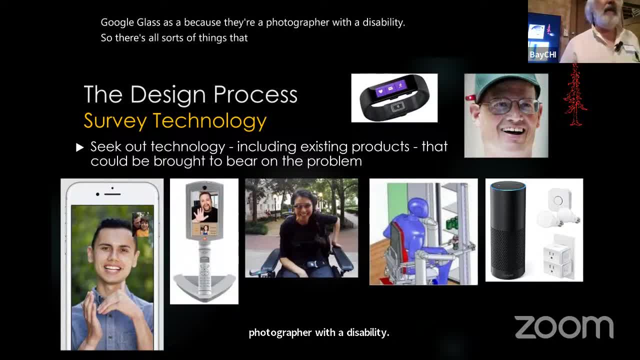 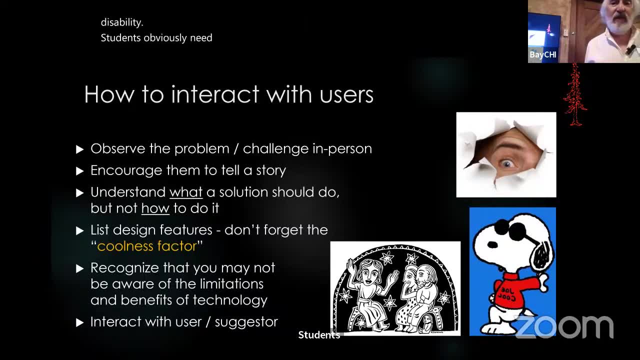 So there's all sorts of things that are on the market that could be adapted for people with disability. Students, you know, obviously need to talk to the person that they're working with and observe the problem and challenge, encourage them to tell the story about what they do. 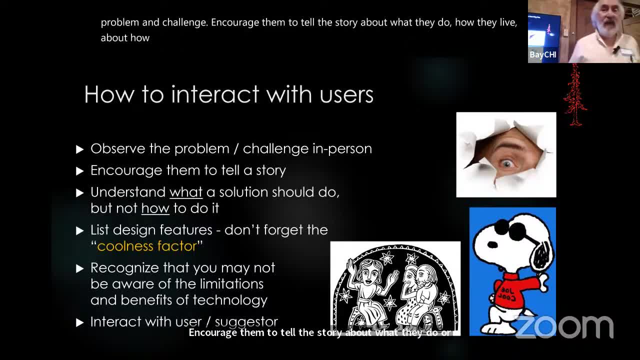 how they live, about how they do things, And so the understanding that they should have from that is to understand what a solution should do. but maybe it's too early to say how it should work. And an underrated design feature is coolness- Everybody you know needs 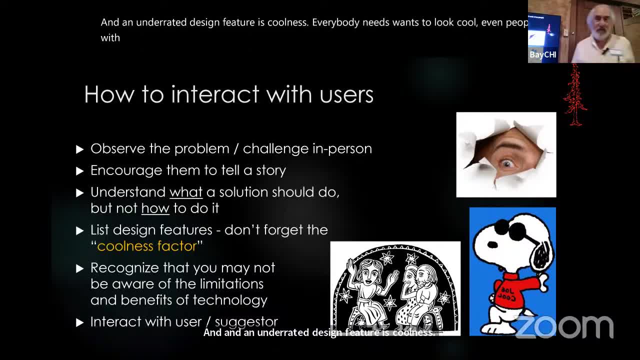 wants to look cool, even people with disabilities and older adults. So when you come up with lots of ideas, you're going to have to think about how you're going to. You put it in a pew chart, a spreadsheet, and one of the factors besides all the design concepts- 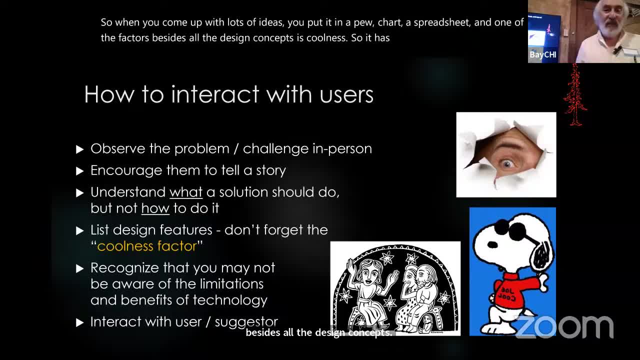 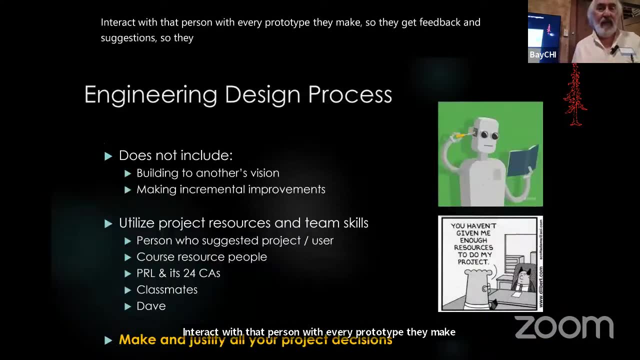 is coolness, So it has to be cool. That has to be checked off, Okay. And students need to interact with that person with every prototype they make so they get feedback and suggestions so they can refine their design. So the design process does not include building to somebody. 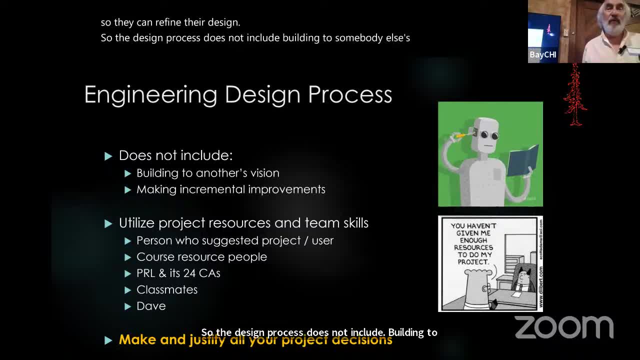 else's design. It's a process of building to somebody else's design. So it's a process of blueprint or making incremental improvements on things. Students who work in a class- you know they have resources from the course- resource people. in the product realization lab There's 24 graduate students who can assist them Their. 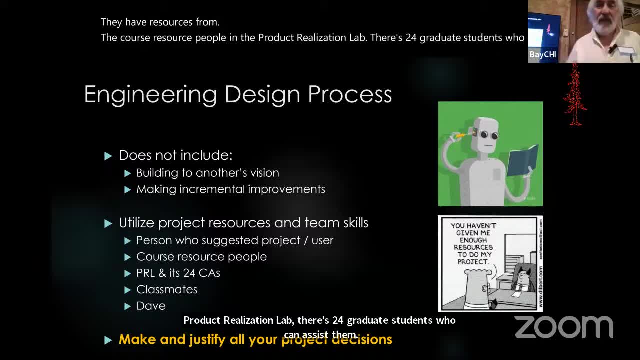 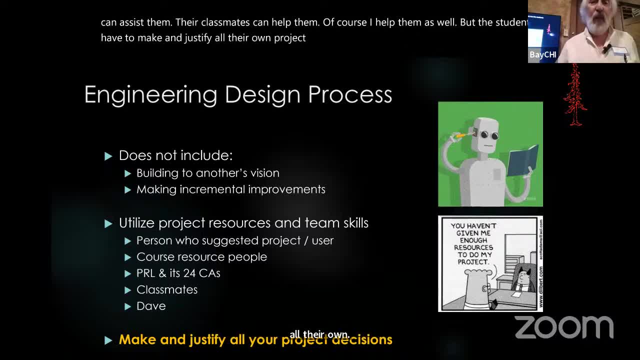 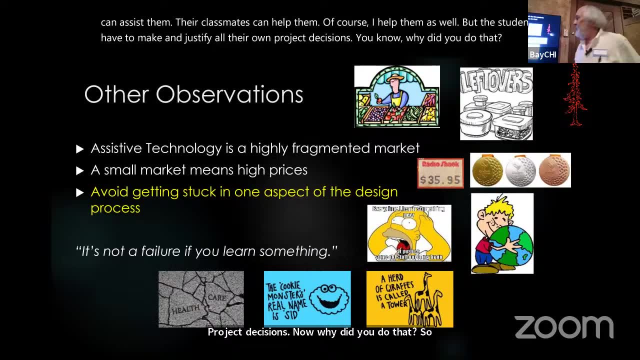 it's a process of building to somebody else's design. So it's a process of building to somebody else's own project decisions. You know why did you do that? So, to summarize, assistive technology is a highly fragmented market. A small market means that there's high prices for the products and 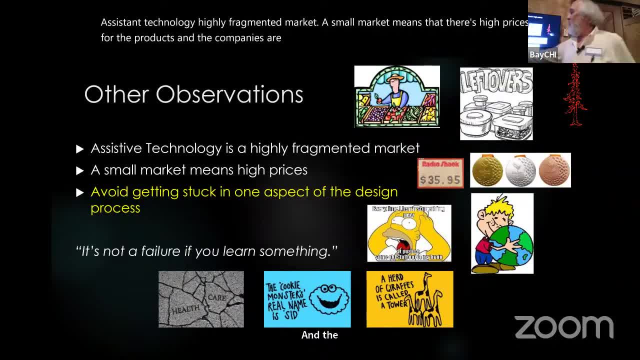 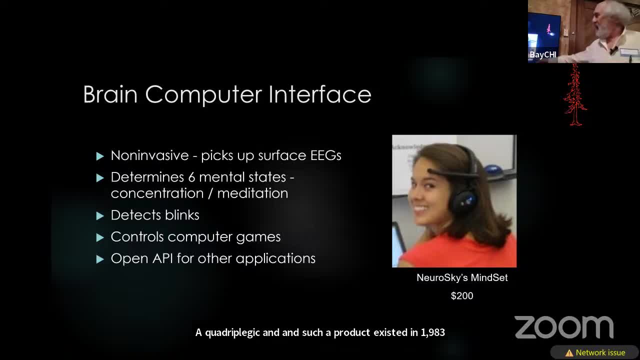 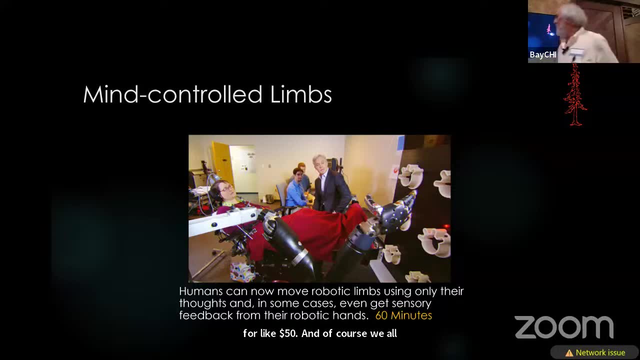 And they're going to be working on a bunch of prototypes. And they're going to be working on a bunch of prototypes. This was a little bit later, and now they sell a version for like $50.. And, of course, we've all seen brain-computer interfaces. 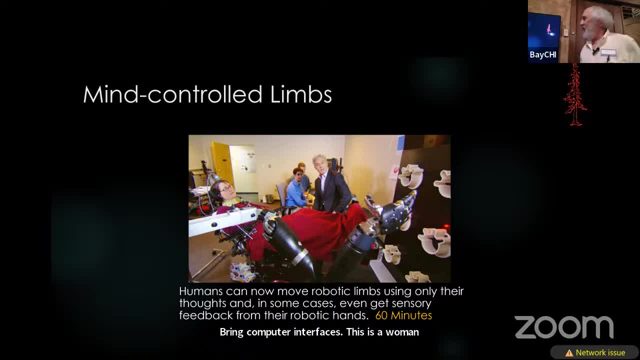 This is a woman that has a couple cables coming out of her brain, that has sensors and she can control. At this time it was one robotic arm, just by thought, and I think she progressed to controlling two robotic arms at the same time, which is actually pretty amazing. 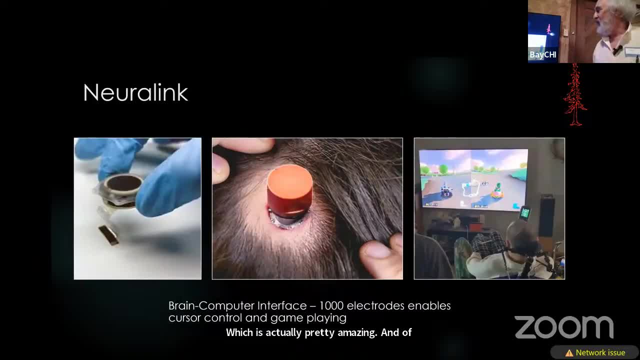 And, of course, we have the Neuralink device, which has 1,000 electrodes, and here's a guy that's playing video games using it. So this is the state of the art. This is what Neuralink is doing these days. 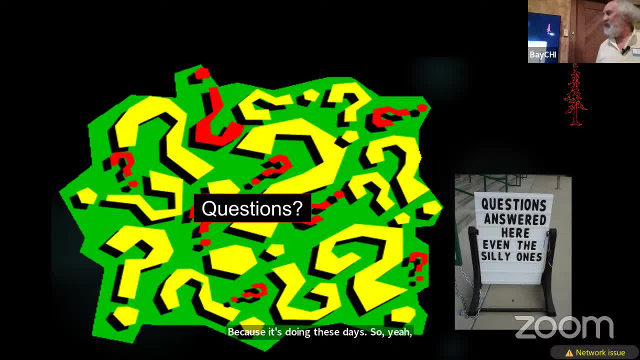 So that's it. I hope I haven't gone over time or got you too bored or whatever, but if you have any, Yeah well, I want to start with Al. I had a question online. Can you unmute and speak for yourself, or I will speak your question myself? 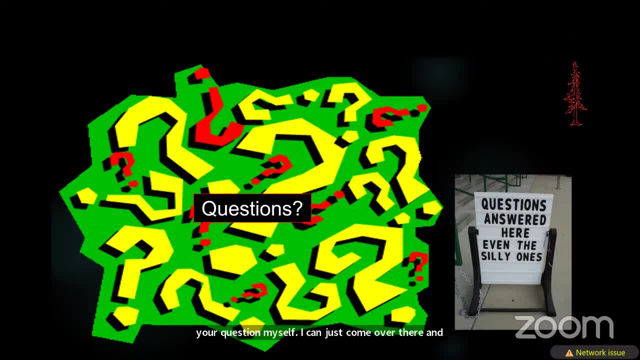 I can just come over there and yell. I just wanted to ask it. if you want, I guess I can Go ahead. Are you able to hear me? Yeah, I can hear you. Okay, great, Great talk. Thank you so much for sharing all this. 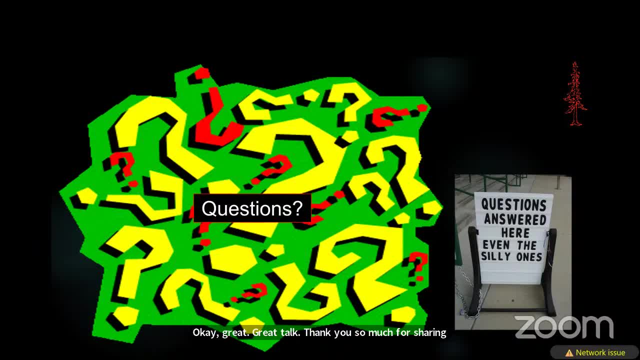 This is really good. So my question is: from your perspective, has robotics evolved And they become highly intelligent and mobile, which seem to be coming up relatively soon- maybe not in our lifetime, but relatively soon, Do you think, Or maybe? 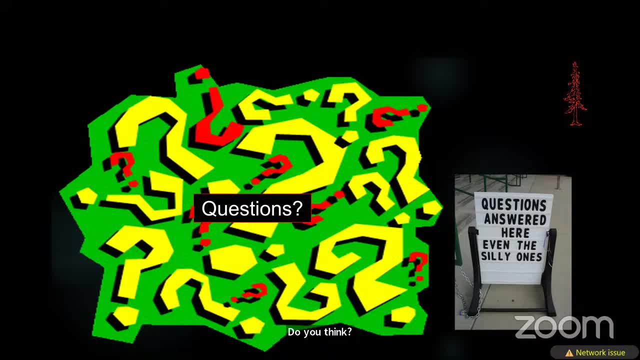 Yeah, well, Go ahead. Robotics helping disabled in all kinds of different ways. Are you okay? Do you have help On their behalf? Do you? Do you have a question or I can read it for you? Yeah, Do you think that's going to introduce new issues or it's going to be a lifesaver for many people? 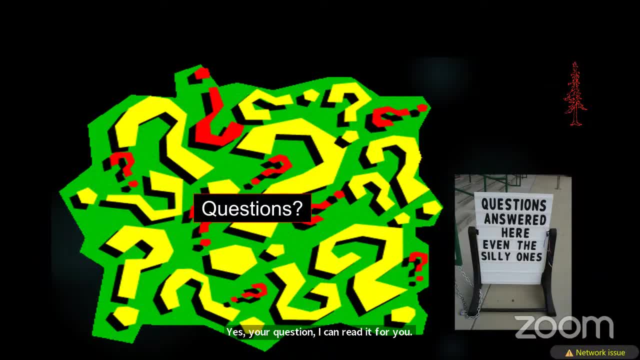 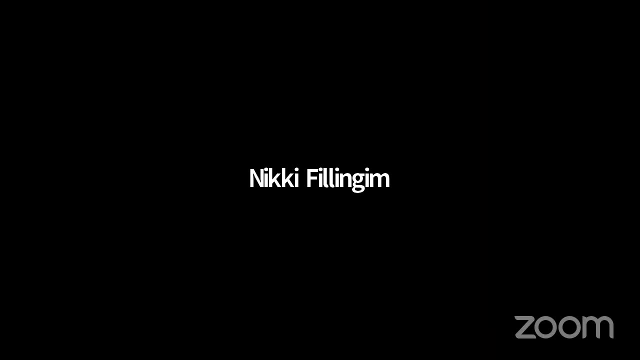 Yes Once again if you had to go. not everything absolutely works out, So can you chat a little bit about that? Sure, I think that goes back to talk about the funnel world and such. So when you reach the Department of Health at the Office of休working, all sorts of things like that talk sort of get stuck. 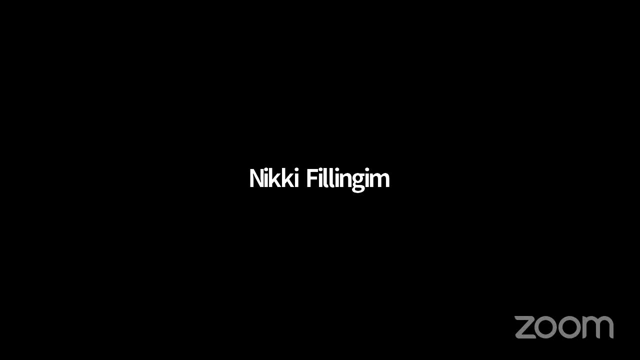 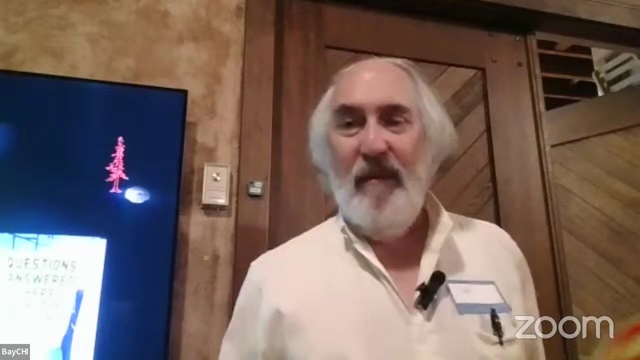 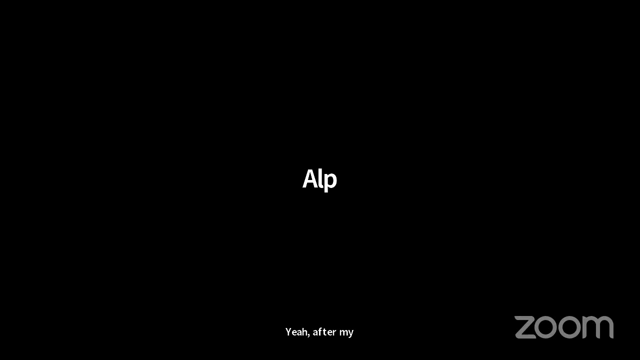 And the whole system works really weird. you Excuse me, We can't hear anything, Okay, Okay, You should be able to hear me now. Yeah, After my question completely went quiet, So maybe you'd like to re-answer it. 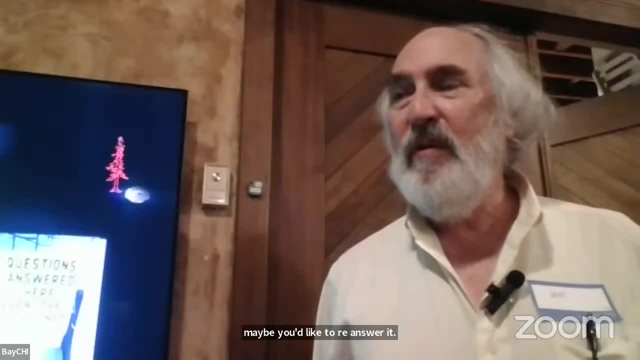 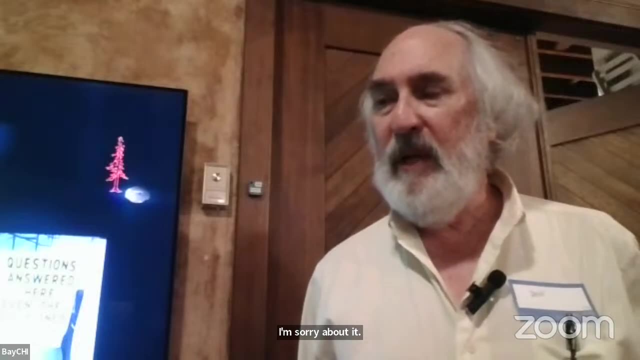 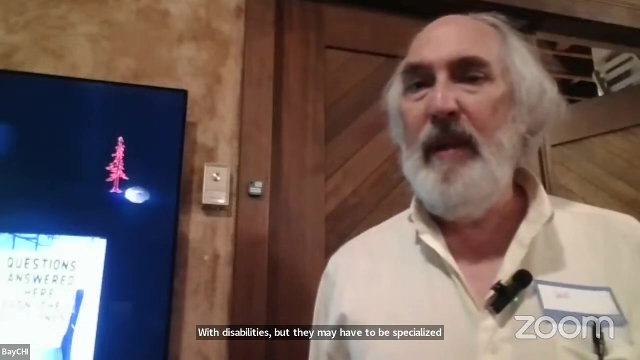 I'm sorry about that. Well, I think technology will advance and there will be applications that would be more workable for people with disabilities, But there may have to be specialized robots for certain things You know there may be, you know. 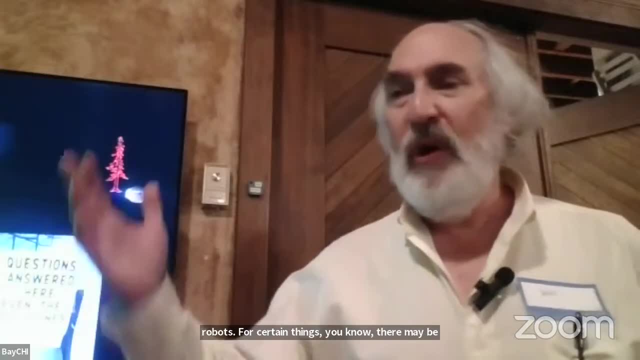 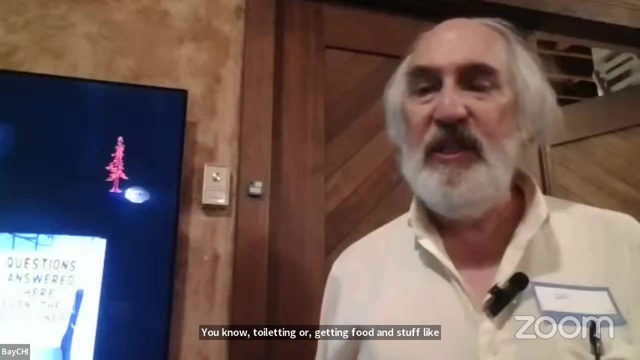 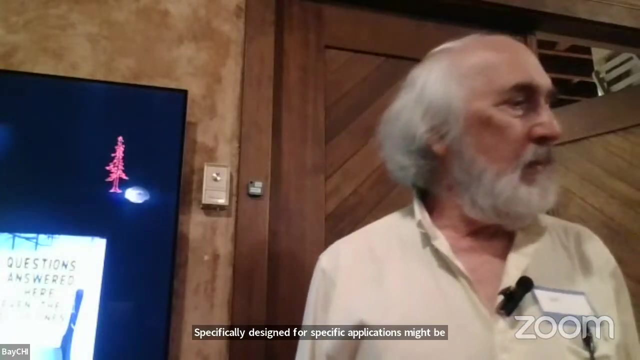 a robot for cooking, another one for, you know, toileting or getting food and stuff like that. So maybe multiple robots specifically designed for specific applications might be the answer. I think part of the question that I saw online was the issue of when we start having AI. 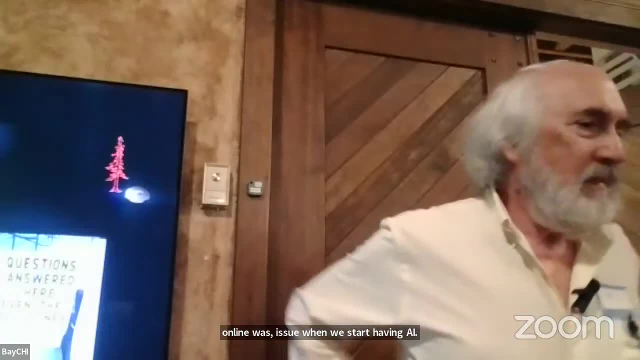 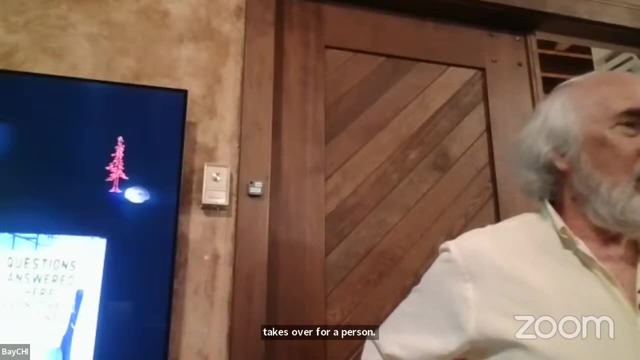 answering with chat, GPT and stuff like that. when it takes over for a person, is that, do they lose agency? And when does it cause problems and when does it solve problems Right? It depends on what the robot is meant to do. 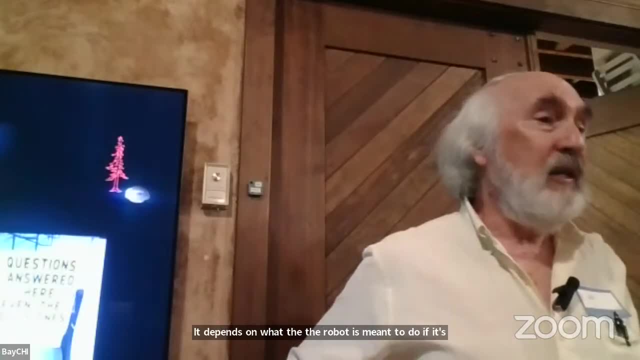 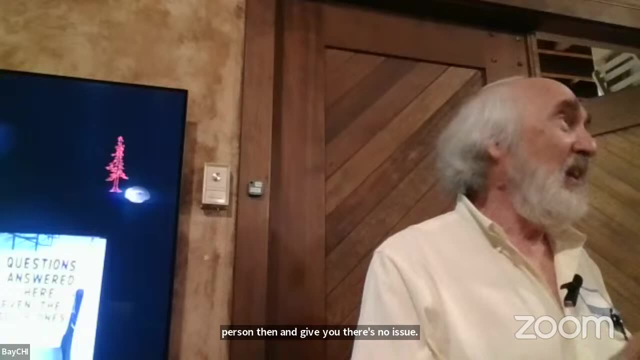 If it's meant to be a caregiving robot and assist the person, then maybe there's no issue. But it's another thing to have it speak for that individual or act for that individual. That's something completely different. So at this point, 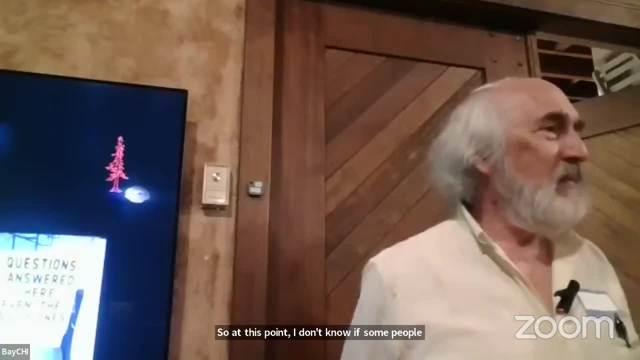 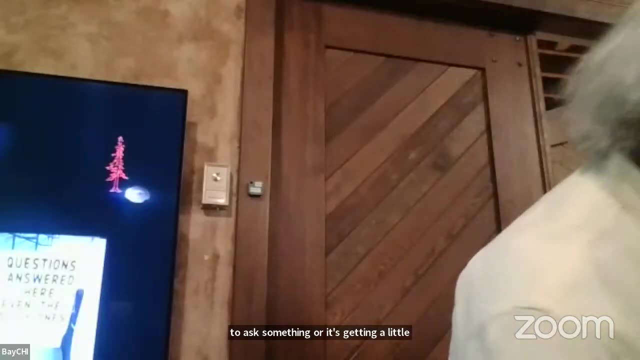 I don't know if some people that haven't asked questions- I've been asking a few- want to ask something, or it's getting a little late and you know, maybe that'll be close to the end, But does any of you? 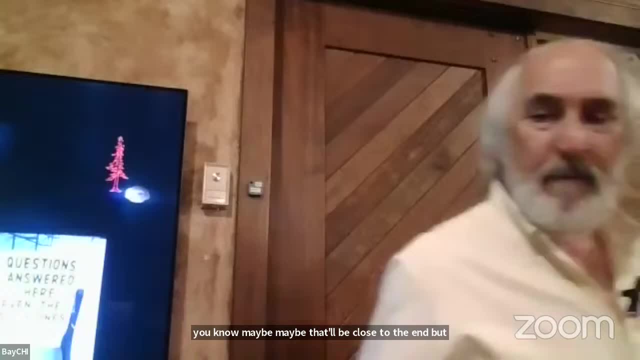 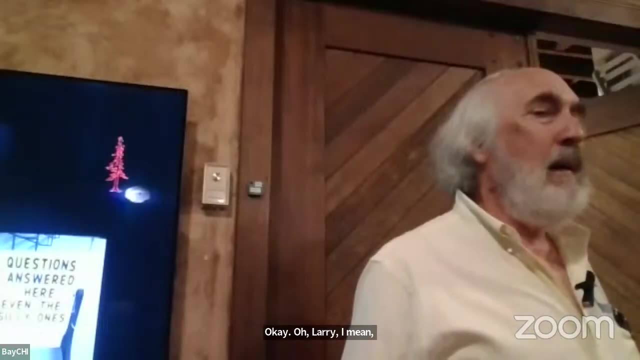 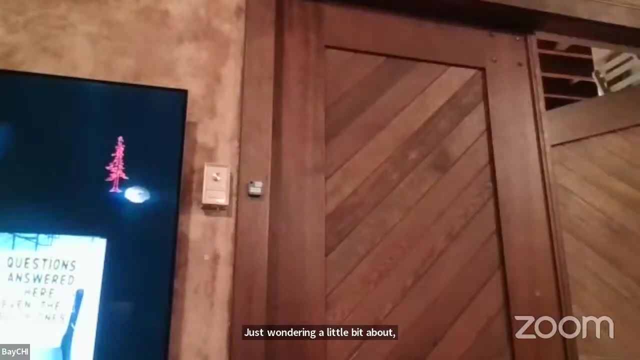 do you guys want to add to the commentary at all, please? No, Oh, Larry, I mean Pete Pete Lynn here from other lab, Just wondering a little bit about neurodiversity and with, in very specific ways, 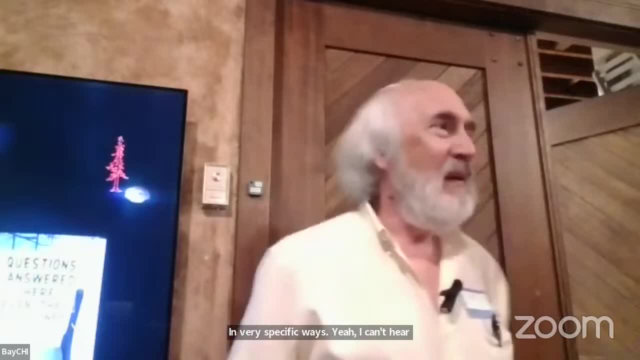 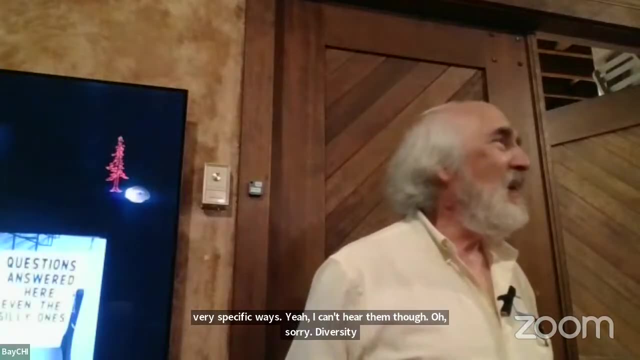 Yeah, I can't hear him though. Oh sorry. What Diversity? Okay, I'll just use my voice. Yeah, I'm wondering a little bit about neurodiversity and whether or not obviously, different people have different things. 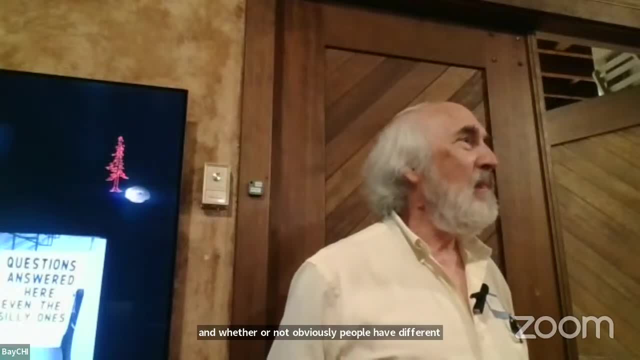 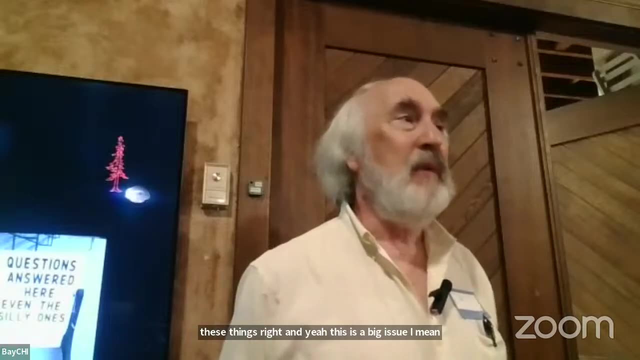 that they're strong at, other things that they're weak at, I mean, whether or not we will be able to directly compensate for these things. Right, Yeah, This is a big issue. I mean, I've always thought that everybody has something. 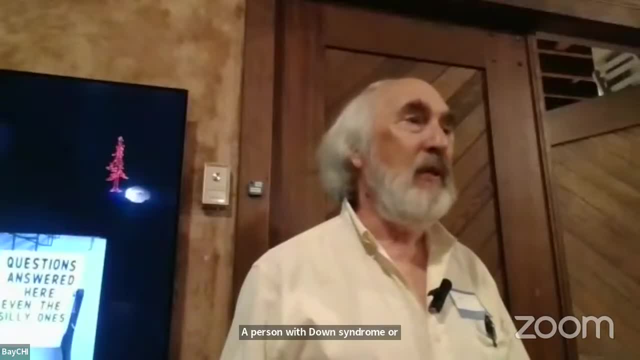 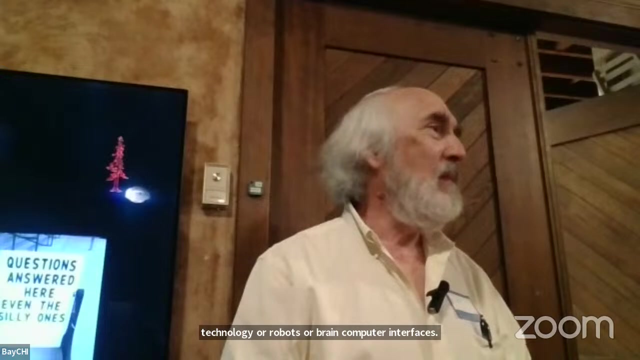 to contribute, even if it's a person with Down syndrome or somebody with autism. everybody has something to contribute. So making that contribution happen through assistive technology or robots or brain-computer interfaces is something we look forward to. That sounds pretty good. 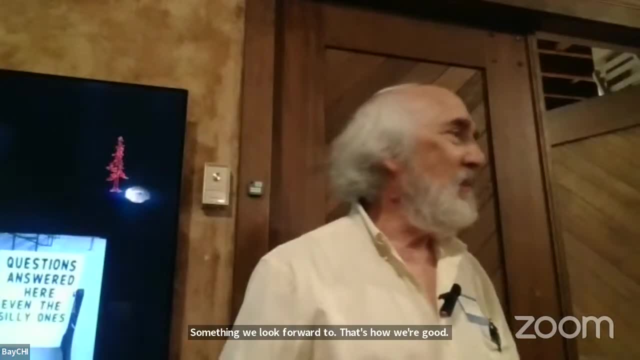 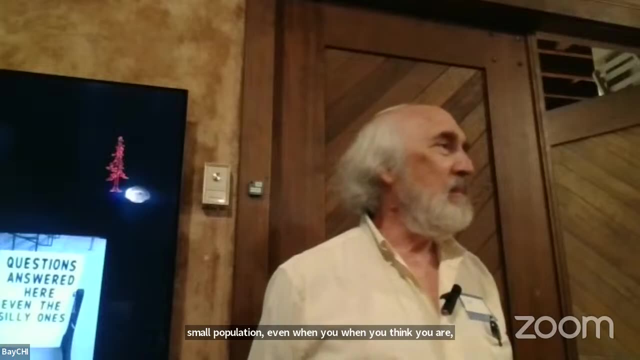 Yeah, I actually think that even when you take a very small population, even when you think you are, you know, selecting for certain kinds of people, it turns out the full diversity of problems and creatives and people who are doing, you know. 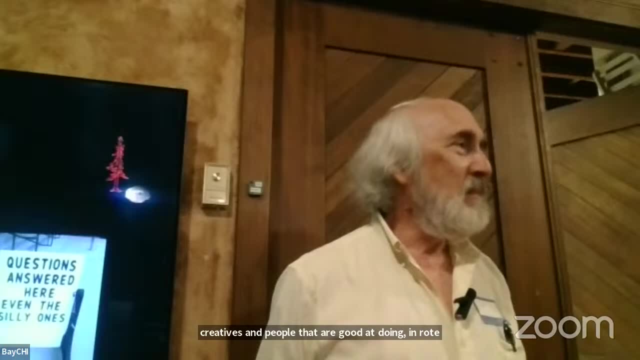 in rote work come out in the population, And I think maybe it's because these different abilities that people have are useful in different situations And actually that diversity is kind of what makes us more viable. Right, I know that there are vocational training programs. 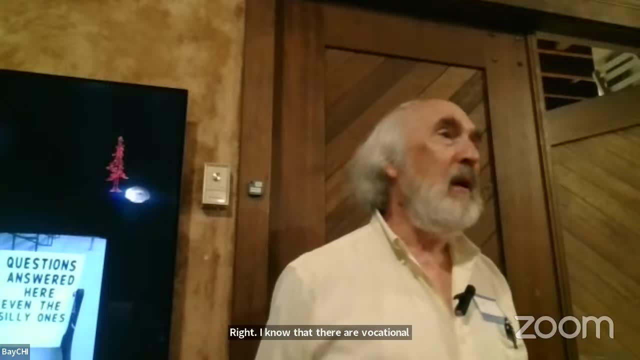 specifically for people with autism, And so you know- I think that's something that you know- everybody can be a contributor. I've seen some awful great artwork and music produced by people with disabilities. Great writing, There's a number. 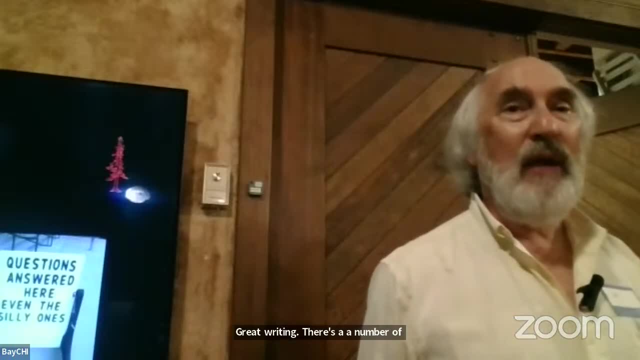 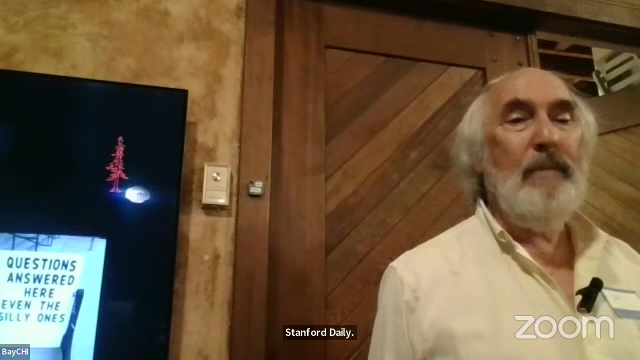 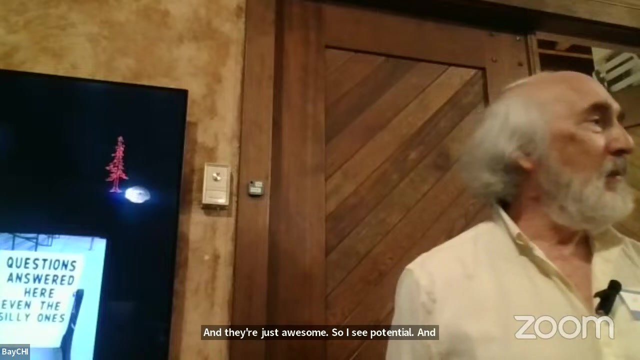 of students at Stanford with disabilities and they all write for the Stanford Daily and they're just awesome. So I see potential and contribution in everybody. So with that, Dave, it's been a very broad discussion. You've given us an understanding. 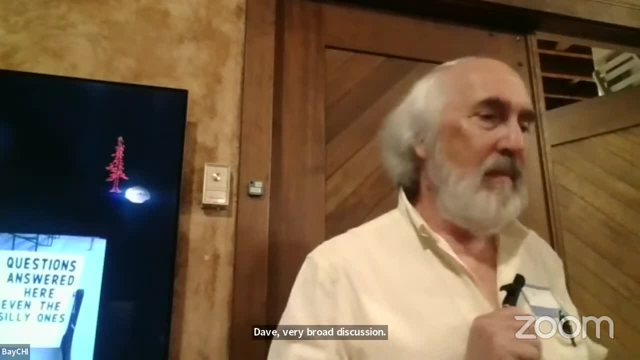 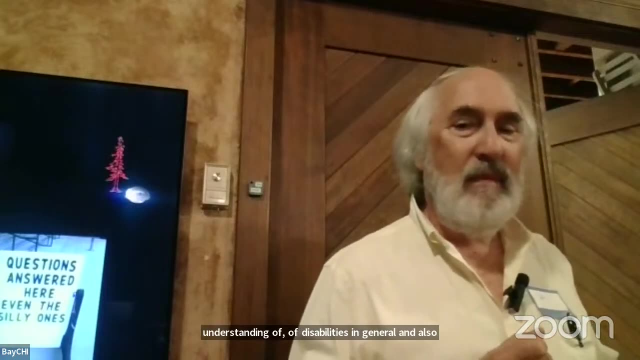 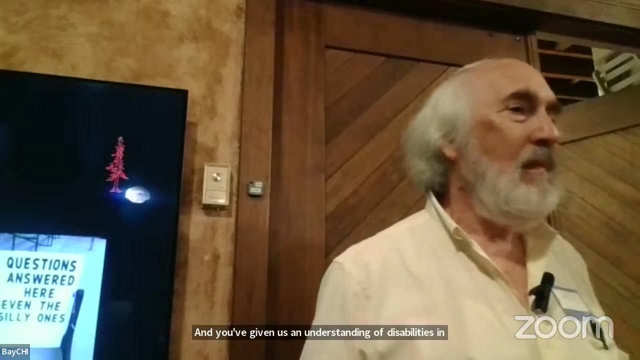 of disabilities in general and also what you teach in your classes, But more importantly, a lot of different examples across a large spectrum, Really more mechanically oriented. not so much software in your examples, And so my last question is: I have to call it. 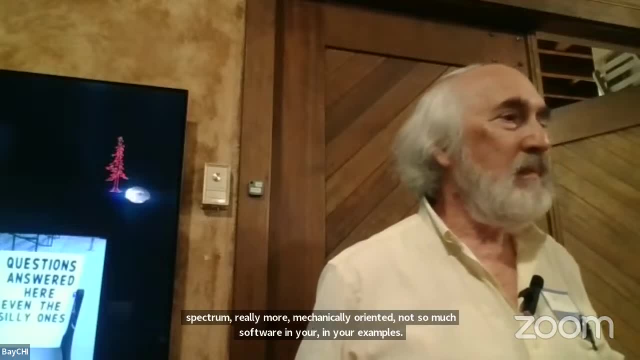 a night very, very soon is: what do you think of the possibility of your class taking on more software projects and what do you think the reasons that it might be more fun to stay with a mechanical or move over to Right? I have had 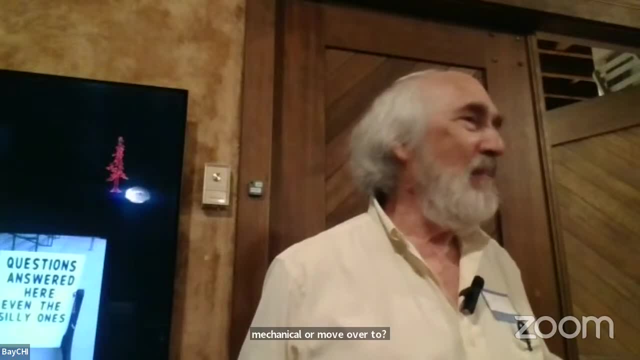 software projects in the past, but I really enjoy when people create something physical. okay, but I'm not adverse to software, but I like the hands-on building of things. But you can imagine a course. that is all. it's all about AI. 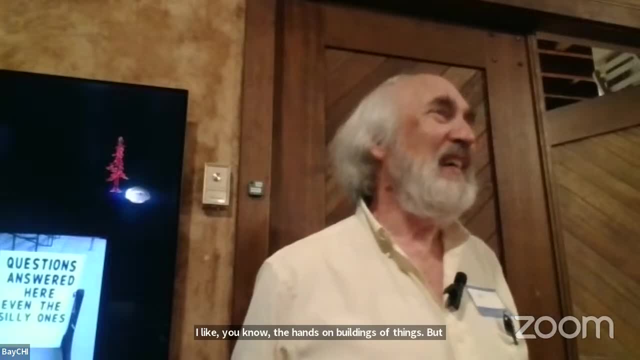 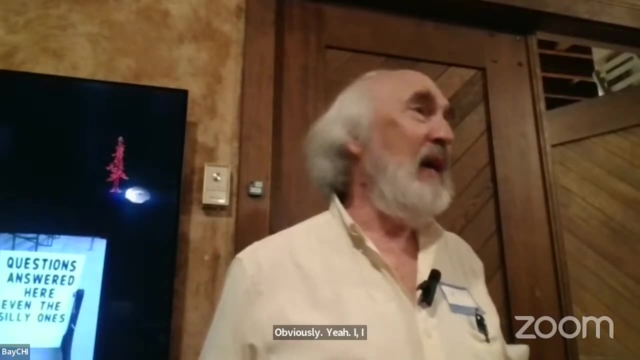 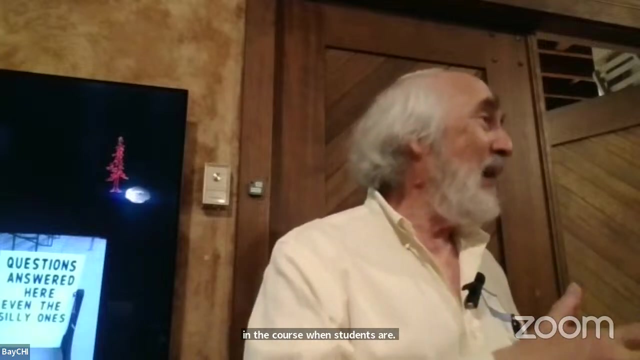 and interaction and language. Not your class. not your class, Obviously. Yeah, I do have a small AI component in the course. when students are trying to understand the problem, I ask them to ask AI about what kinds of solutions AI might have. 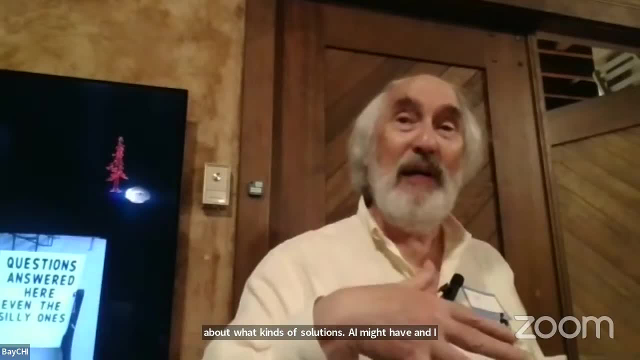 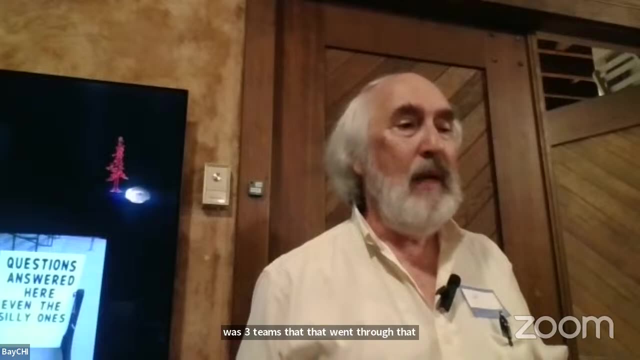 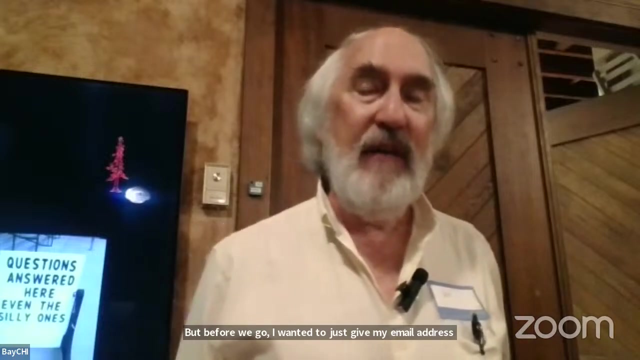 And I have the students comment on those responses And so there was three teams that went through that exercise. But before we go I want to just give my email address. It's davejaffe at stanfordedu And my course.